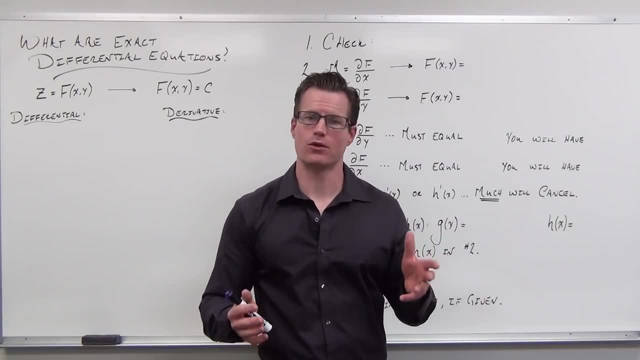 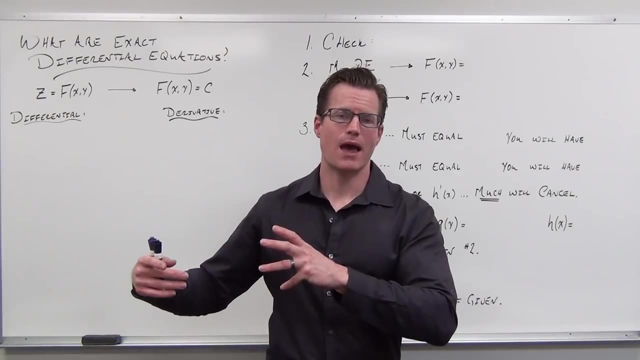 curves And in physics and engineering these level curves happen an awful lot and they're very important And a lot of times we're trying to get this potential function that's giving us a level curve And that's the impetus for talking about these exact differential equations. So one 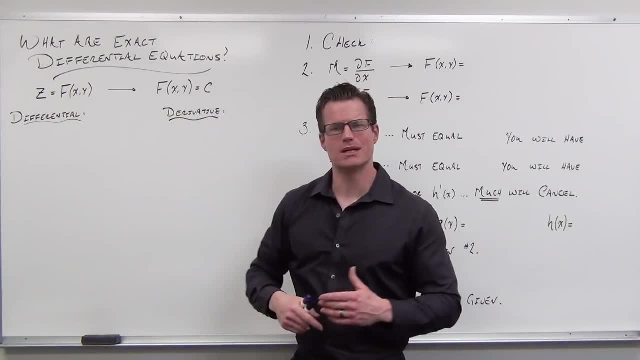 more time. Those are surfaces. set them equal to a constant. you get something called a level curve. Now I'm going to show you two ways to get down to the idea of what is an exact differential equation. So I want to discover what that means, but what it required. 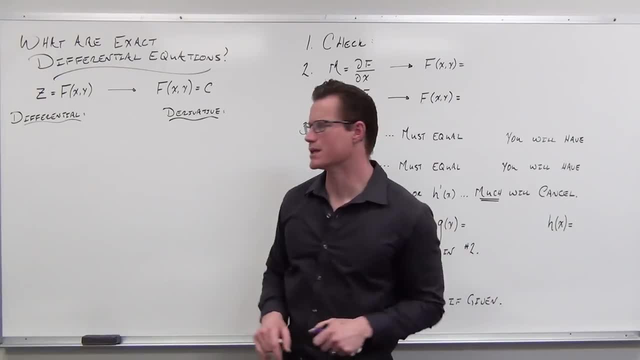 was us kind of knowing where we're coming from. So why in the world are we doing this? We have these things called surfaces. If we set them equal to constants, we get these things called level curves, An exact differential equation. this is a little bit complicated. Well, that's what we're going to do. In physics and engineering, we're going to get something called a level curve. So what we're going to do is we're going to show you two ways to set both surfaces equal to a constant, and then, all of a sudden, we're going to get something. 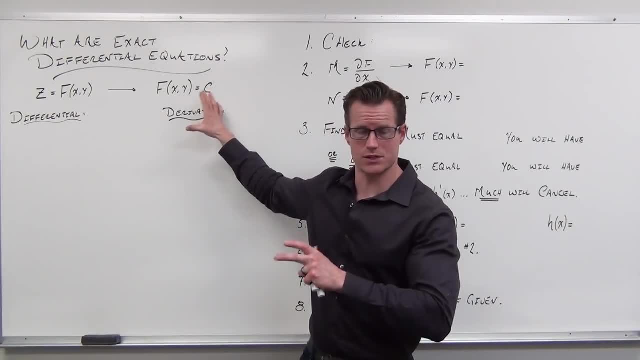 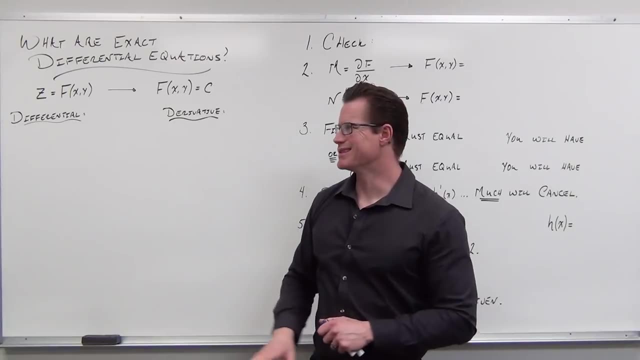 exact differential equations deal with level curves. That's what they're dealing with, So let's see where they come from. Now, the two different ways I'm going to look at this is: if you remember, back to surfaces, the way that we can find differentials took a long time to. 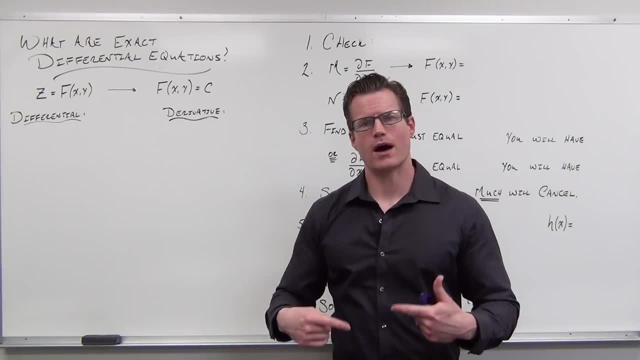 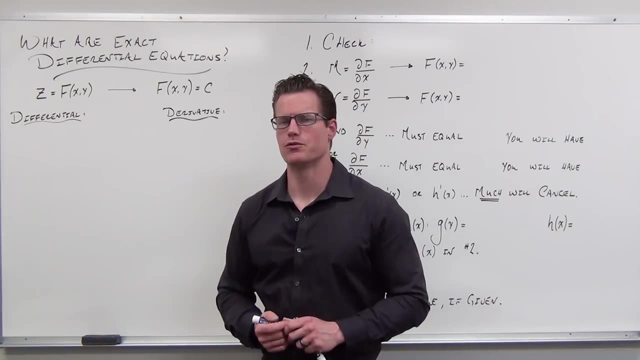 explain And again you should check that out. But in order to find the differential of such a function, what we would do- and by definition we sort of proved it and kind of loose proof when I went over it would be like this: What we'd say is we'd say the differential. 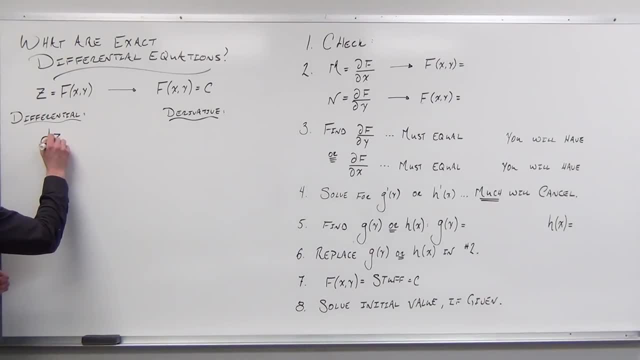 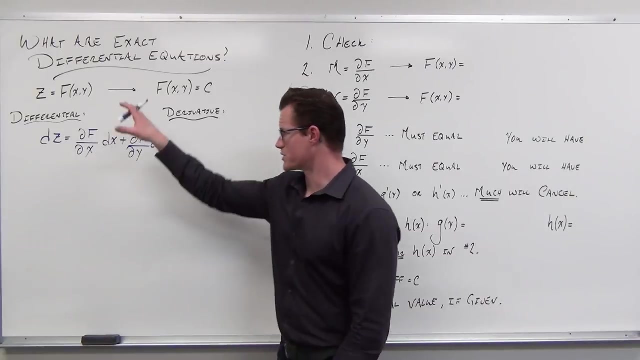 of z is the partial derivative of f with respect to x, dx, plus the partial derivative of f with respect to y, dy, And that is the definition of a differential of z For such a function. Well, let's look at it a different way. Let's look at it from here, So, 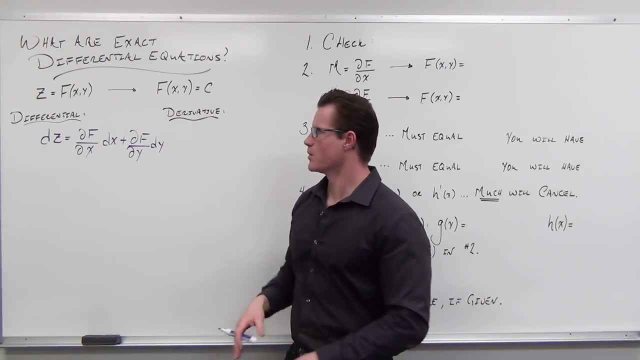 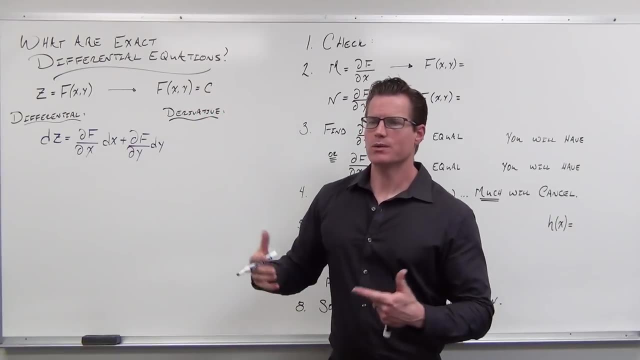 imagine you start with these functions. that's a surface, Okay. well, the differential would be this, And you'd find that in any calculus book or one of my videos. Or let's suppose we start with the level curve. How would we get down to the same thing And the idea, a different way to look? 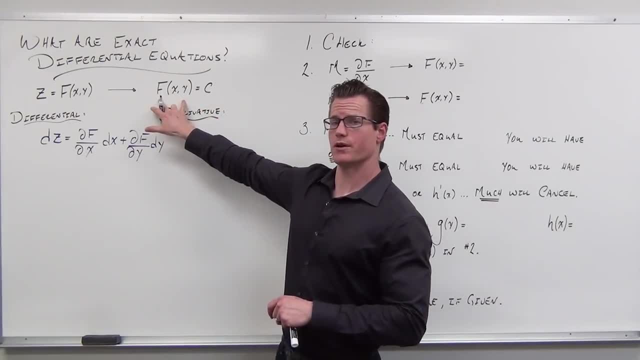 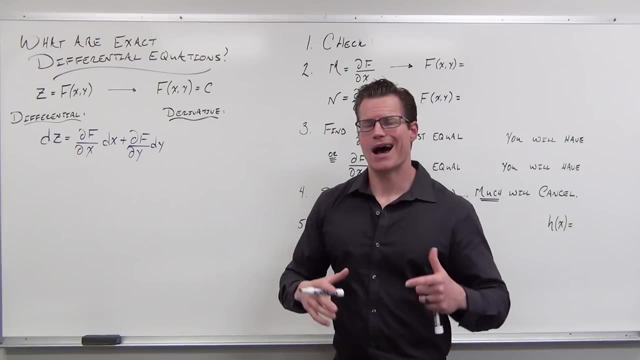 at this would be what if we looked at this as a function of two variables equal to a constant? Well, in such a case, if I wanted to find the derivative of that function with respect to x, I could do that by looking at the same thing. And I could do that by looking at the same thing. 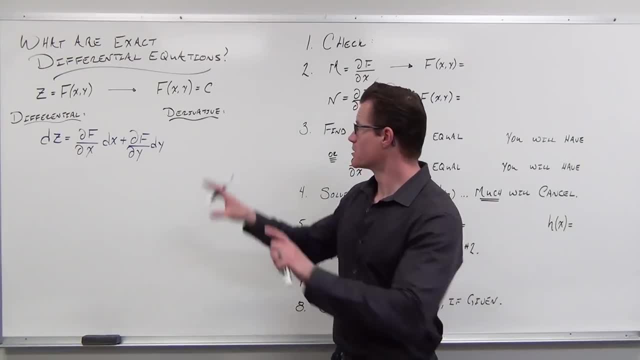 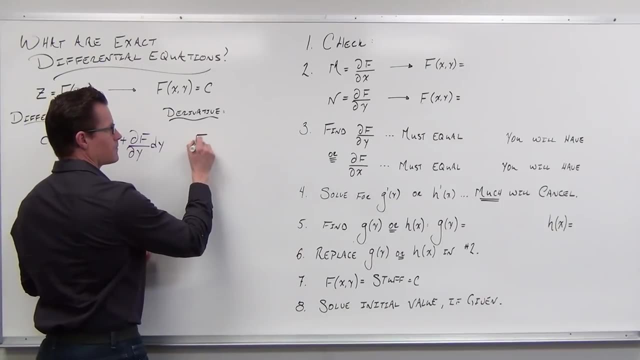 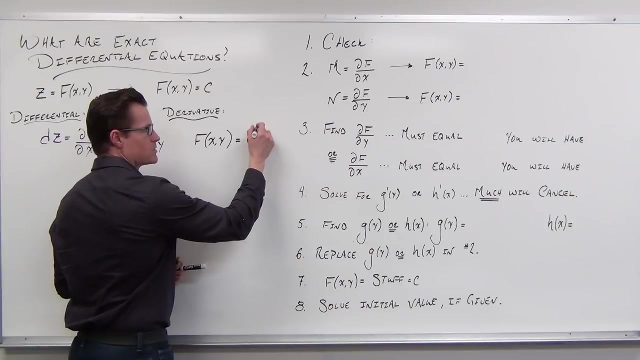 and I could do implicit differentiation And one way to accomplish that, so taking a derivative on both sides with respect to x. So let's take a derivative on both sides. Excuse the notation here. I'm just going to do this Derivative with respect to x On the right-hand side man. 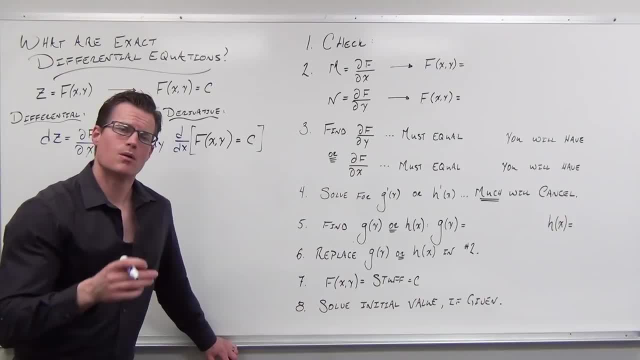 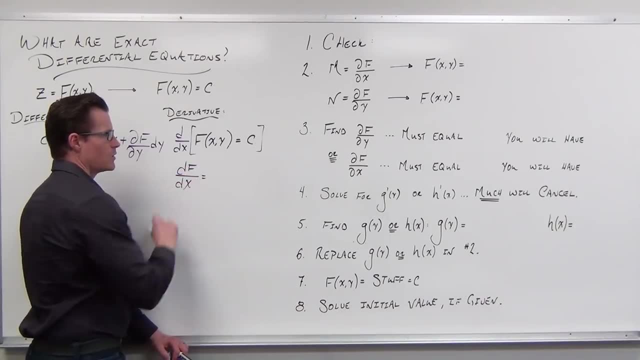 we know we're going to get zero. Derivative of a constant with respect to x is zero, But on the left-hand side the derivative of f with respect to x would equal. we would take- and this is kind of cool. this is a way that you can do implicit differentiation with respect to x. 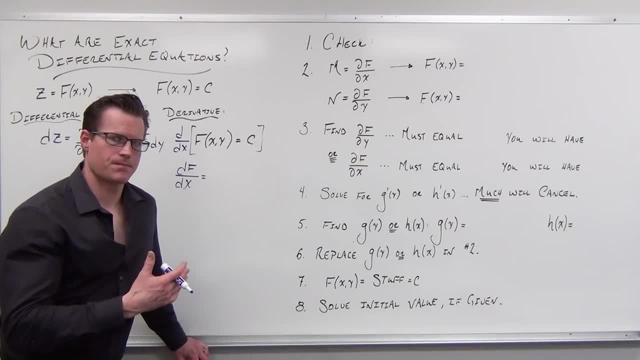 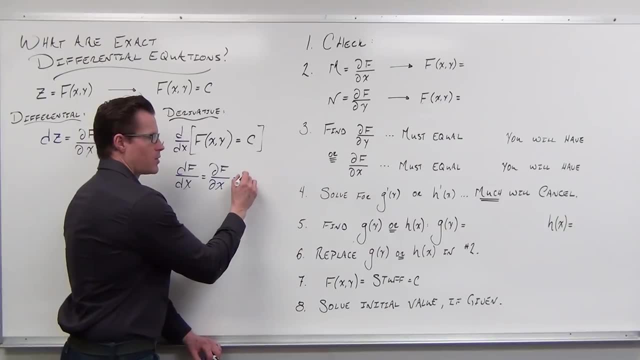 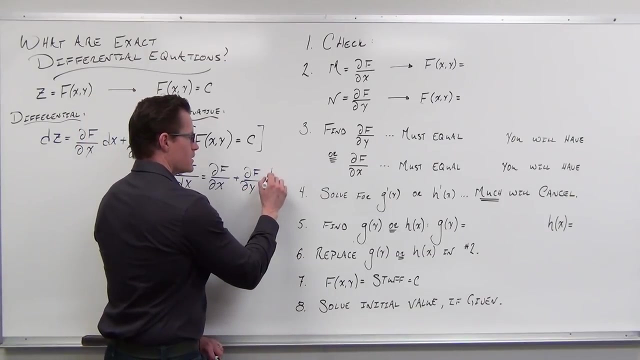 You would take the partial derivative of f with respect to x plus the partial derivative of f with respect to y. But because you have that chain rule, we'd have this dy, dx, And again on the right-hand side, the far right-hand side, you would get zero. So just, 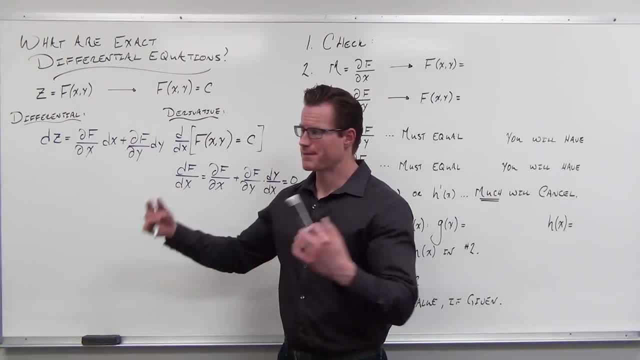 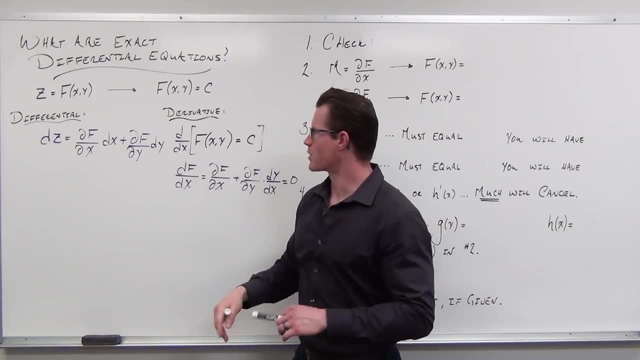 like a 10-second recap here. we're looking at this two different ways, And so we can get the same thing. I'll show you that in a minute. So if we have these surfaces, the differential would be defined like that. Okay, that's a differential, No problem. If we look at this as a level curve. 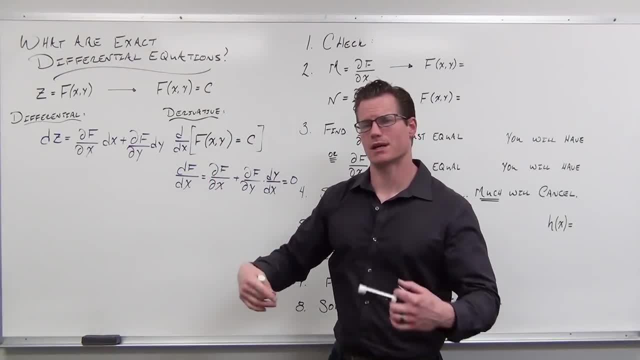 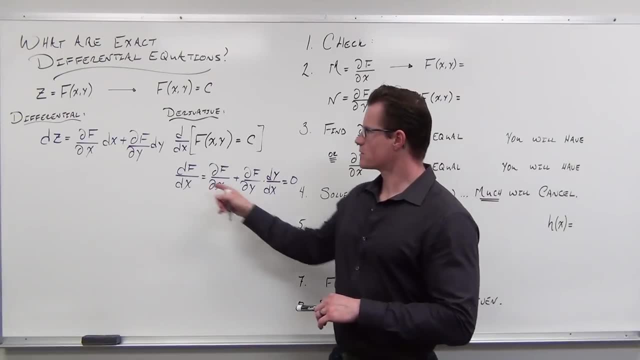 well then, if we take a derivative on both sides, implicitly with respect to x, that's going to involve implicit differentiation. or we can think of this using partial derivatives. So you go. well, those don't look the same. How would we make this look? 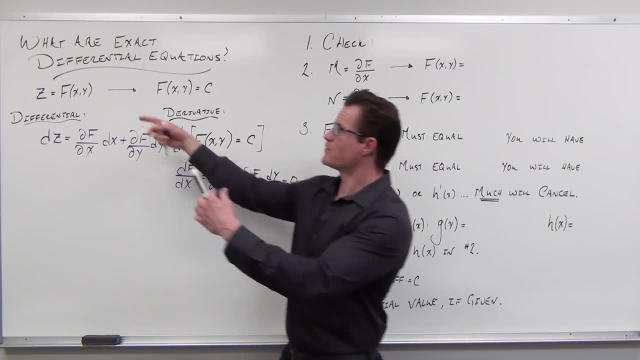 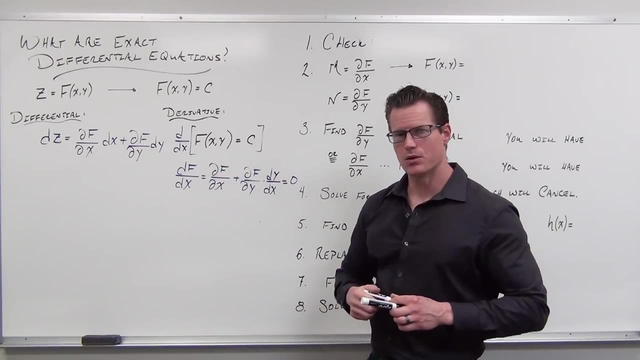 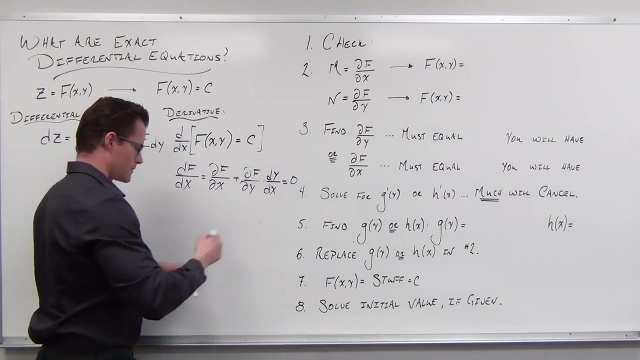 like that And you go. well, firstly, they're coming from a slightly different place right now, So we're going to have to change this one a little bit. But if we formally multiply both sides or all of this by this dx, that we can do so if we just multiply everything by dx. 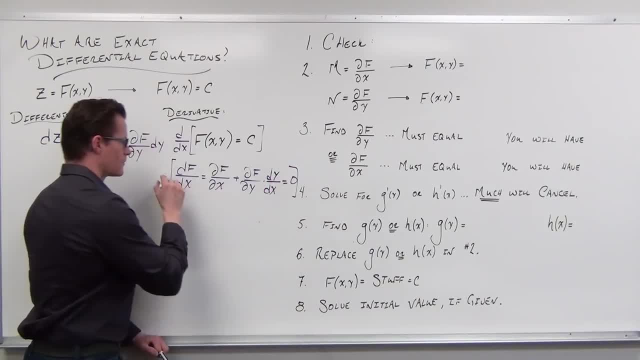 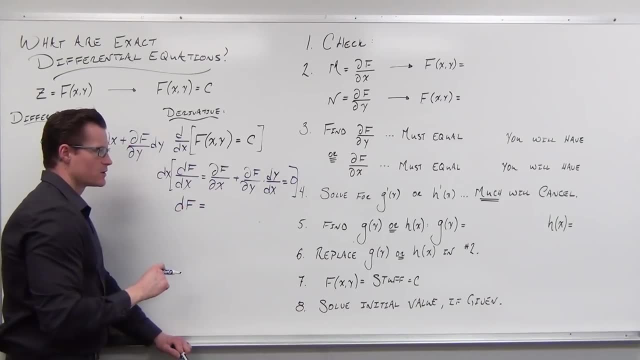 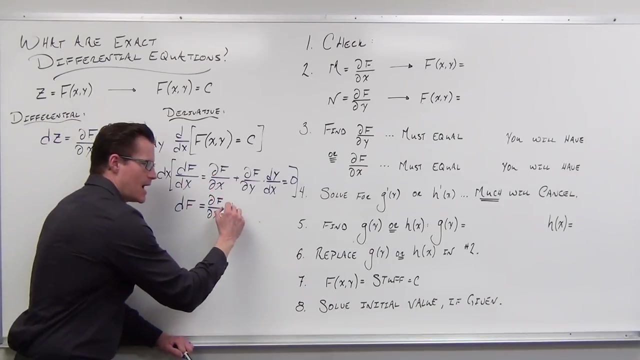 then we would get df, or the differential of f, is we would get a partial derivative of f with respect to x, but we would have a dx. Now this would give us a partial derivative of f with respect to y, but we would get rid of that dx and just have a dy. We would still have. 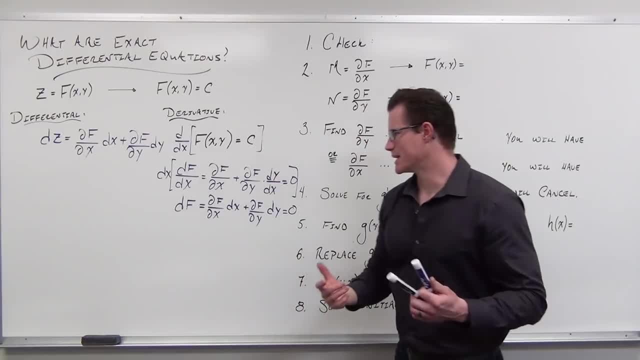 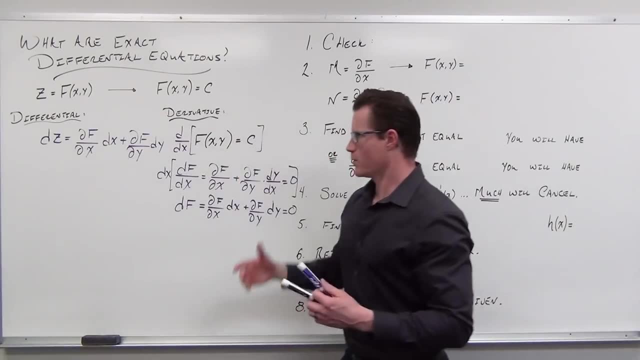 zero, Zero times anything still gives us zero, which is kind of an interesting idea. Now I'm going to change this just a little bit, and then we'll talk about how these things are the same. So let's go back over here. We go: okay. well, how's the differential? That looks. 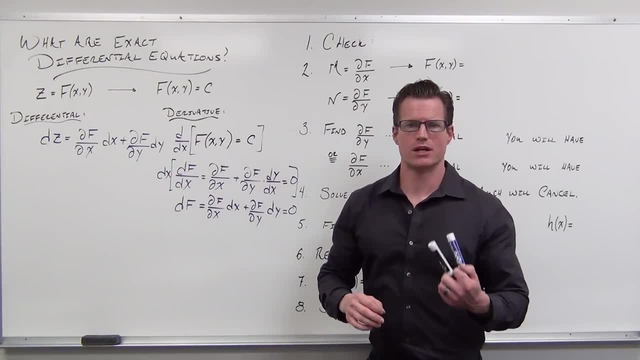 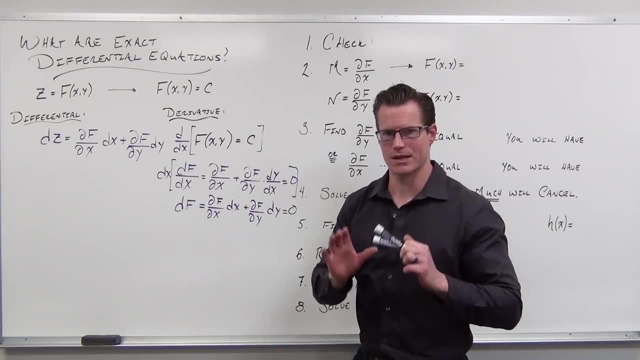 pretty close actually. We just don't have a zero. Imagine that z changes to a constant. We go all right. well, if z is a constant instead of an actual variable z and we say we are going to set this function equal to a constant to give us those level curves from that surface, then this changes. 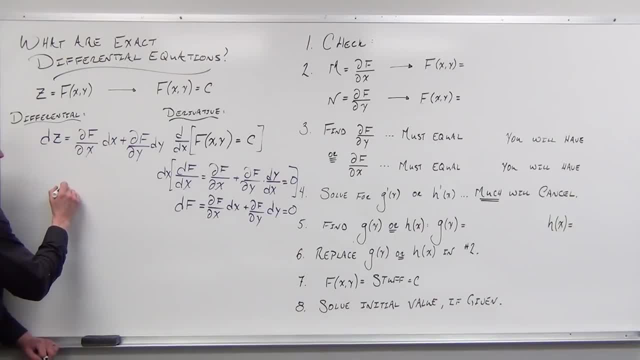 a little bit. Then this says: all right, then this differential: if we set this equal to a constant, it would just change to this: It would be the partial derivative of f with respect to x, dx, the partial derivative of f with respect to y, dy, and then we would get zero And we get exactly. 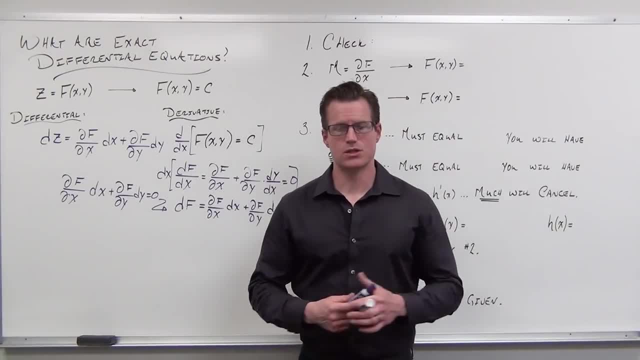 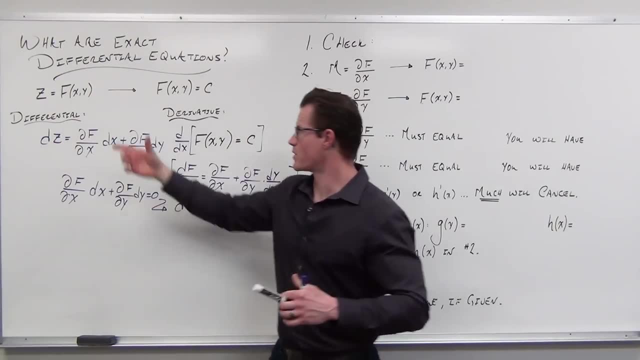 exactly the same thing. So, again, there's two ways to really look at this. Do you look at it as a differential of some function equal to a constant? Well, here's the definition of a differential. Here's the definition of a differential from this surface And we go. well, let's just make it equal. 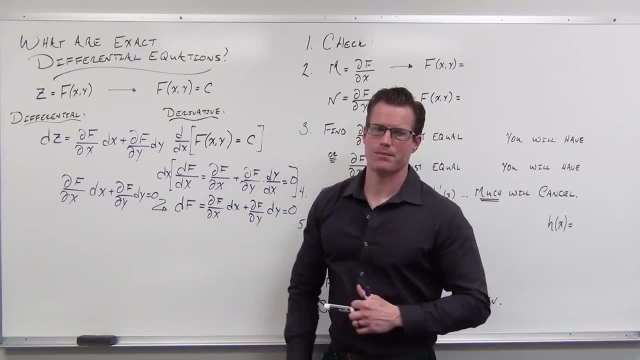 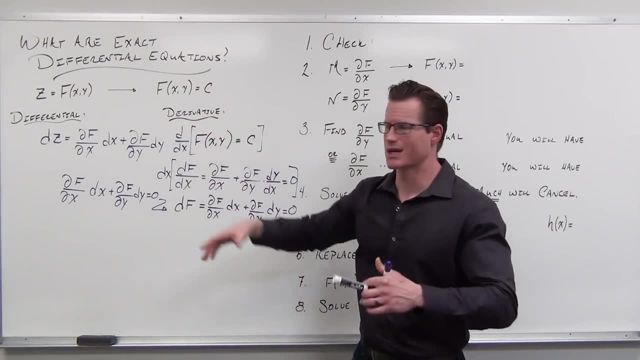 to a constant. If we do that, then the derivative gives us zero, And so we have this differential right there from that function: equal and constant. Or do you look at it as a level curve and take a derivative on both sides? Either way is fine. If you look at that implicitly, you got partial. 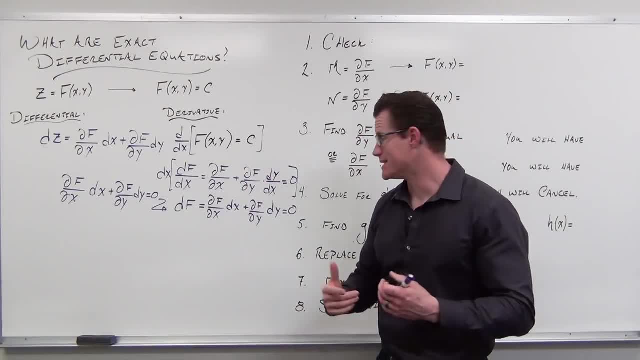 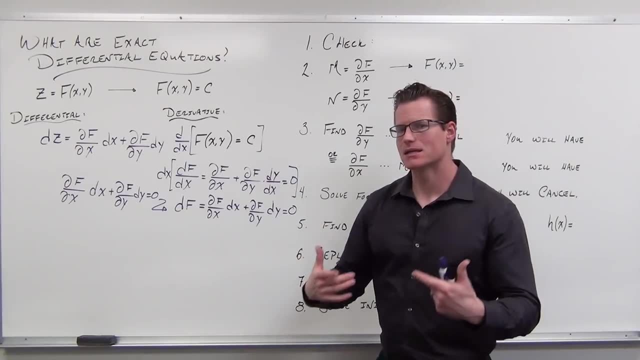 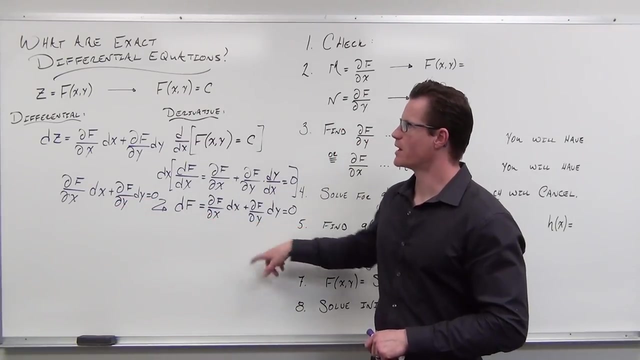 derivative of f with respect to x, plus partial derivative of f with respect to y, dy, dx, and we formally multiply by dx. Now here's where the name exact differential equation comes from. What these are called, what these are called, this is called the total differential. for some, 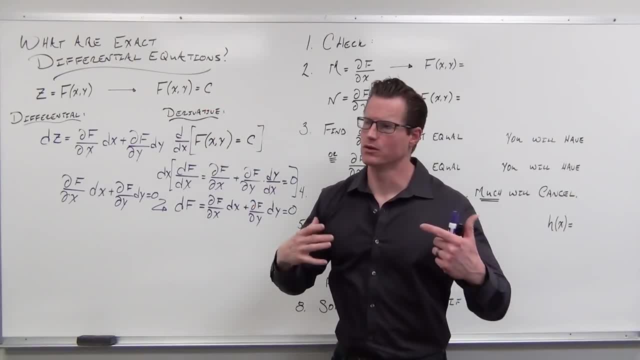 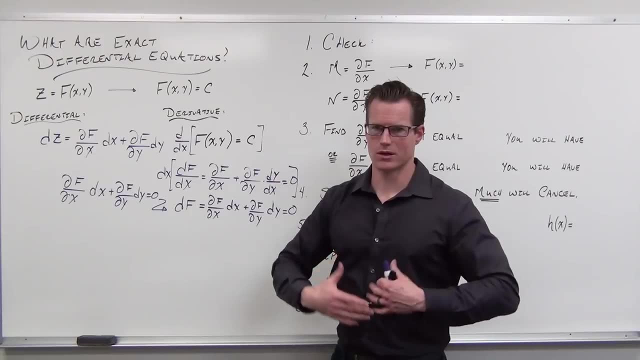 potential function I will miss. I learned it as parent function, so I will say that from time to time. If you hear me say parent function accidentally, it really is potential function. I learned it the wrong way when I was going through it, So that's called a potential function for some. 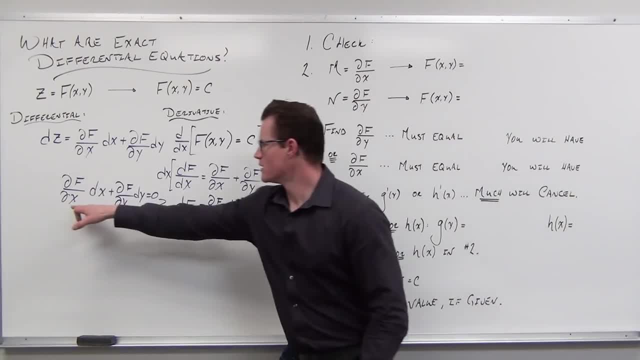 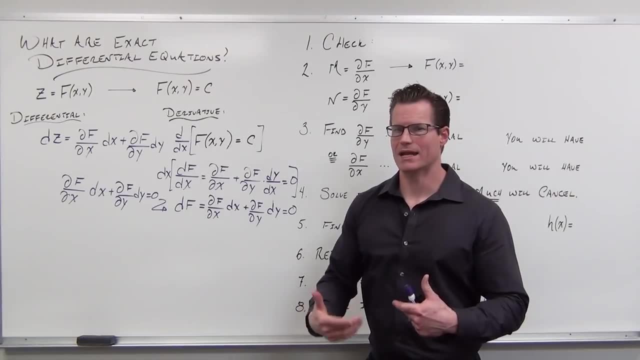 exact differential equation. Now why they're called exact differential equations? these things, this thing, this exact same thing here is called a total derivative differential or an exact differential. That's the name of it, And so when we talk about an exact 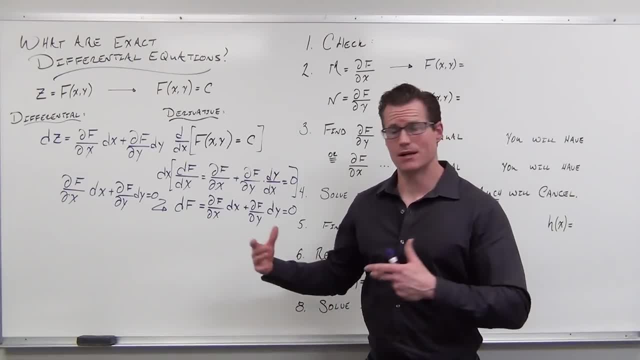 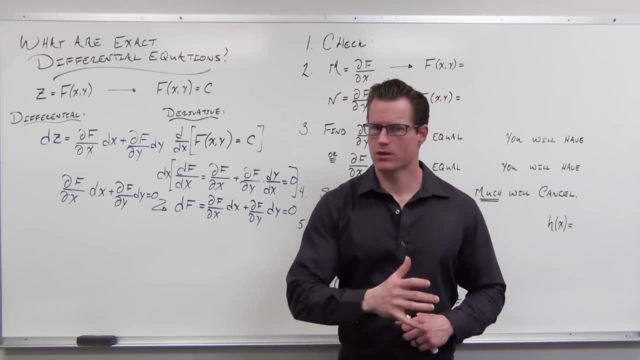 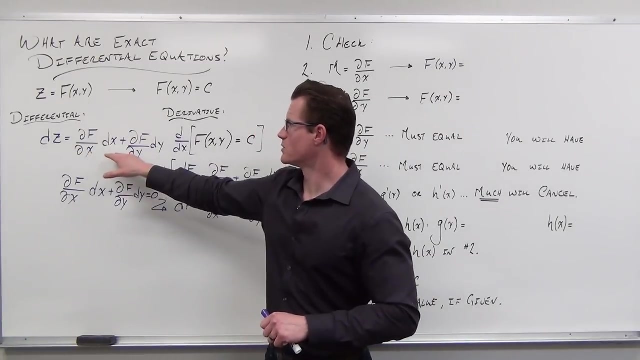 differential equation. what we're talking about is a differential that's coming from some potential function, which is a level curve One time all the way through as fast as I can go, like maybe a 20 second recap. We can look at this two different ways, just as a differential, and then say okay. 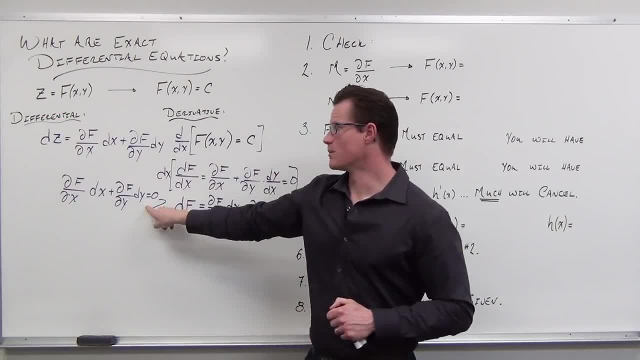 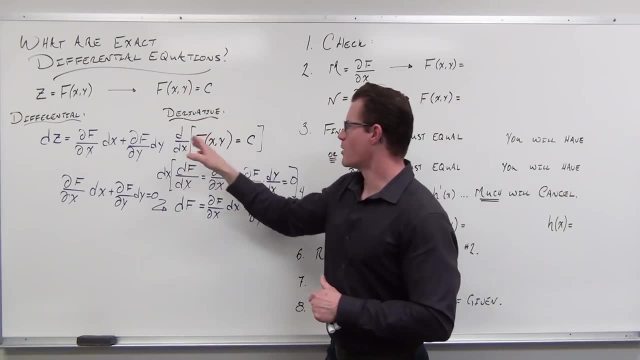 but what if that is a constant? Well then we get this equal to zero, And this is called the total exact differential. Or we say: let's look at this as level curves, Let's take a derivative on both sides, No problem, We'll have implicit differentiation, We'll have a zero over. 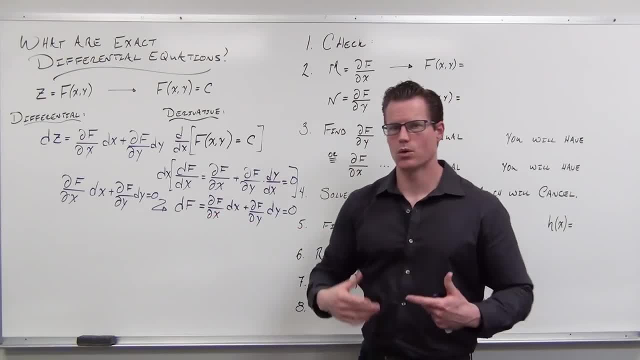 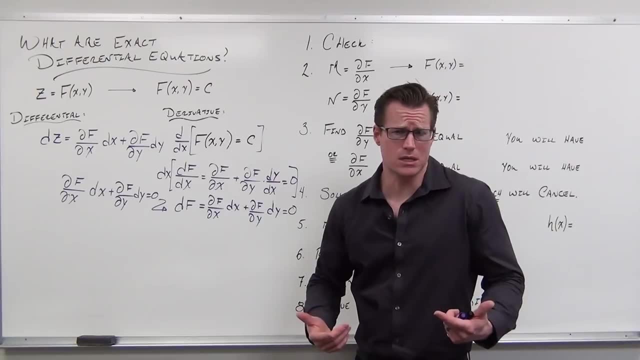 here We'll multiply by dx and we'll get again the total or exact differential. I hope that I've made this make sense of where it comes from. The first time I went through it I was like I have no idea what that actually means When I was learning it. what does an exact differential 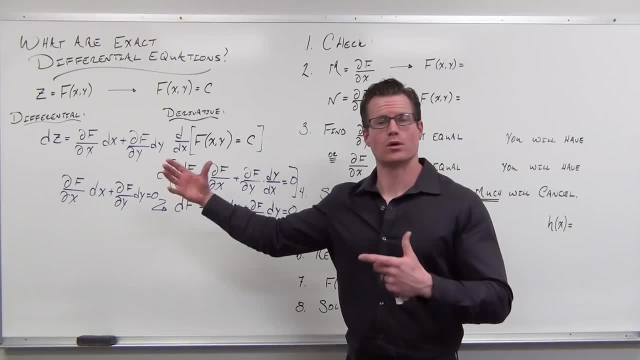 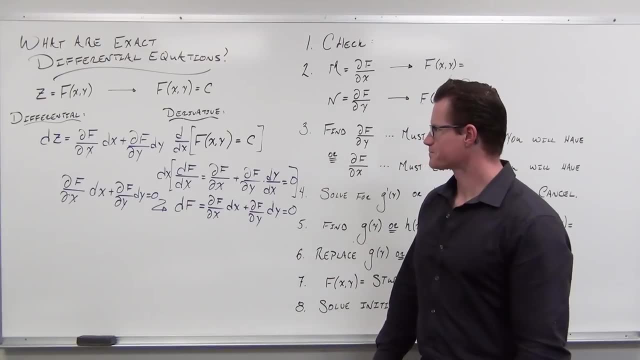 equation mean. Where does it come from? It comes from a differential or it comes from a derivative- and changing it into what's called differential form as a total or exact differential. Now, why is that important? What do we actually do? Well, let's go a couple more steps and see. 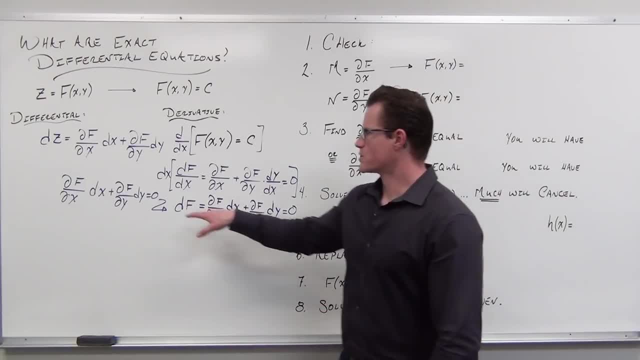 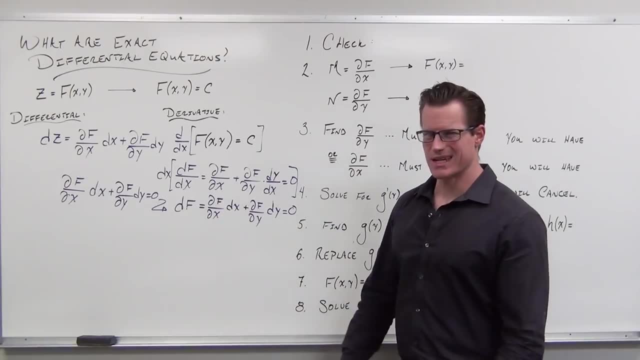 what's going on When we get these differential forms of these differential equations or a total differential here. oftentimes you won't see this partial of f with respect to x and you won't see the partial of f with respect to y. What you'll see is the letters m and n or some other letters. 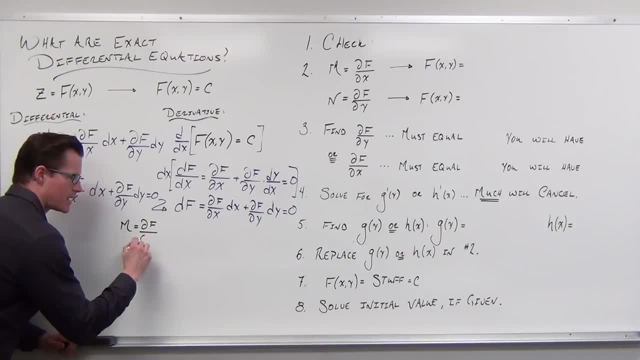 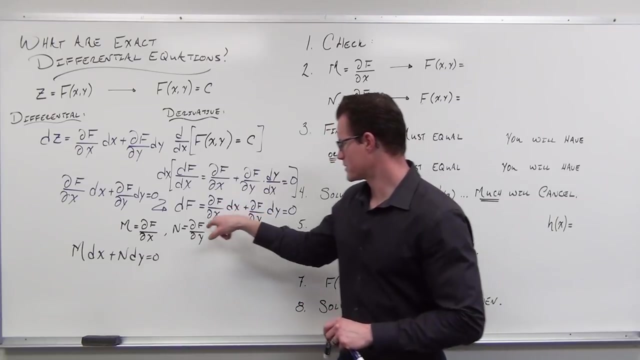 So if we were to combine m to be the partial of f with respect to x and n to be the partial of f with respect to y, then this total differential changes to mdx plus ndy, equals zero, And that probably looks familiar to you. Oh, yeah, yeah, that makes sense because we have this Okay. 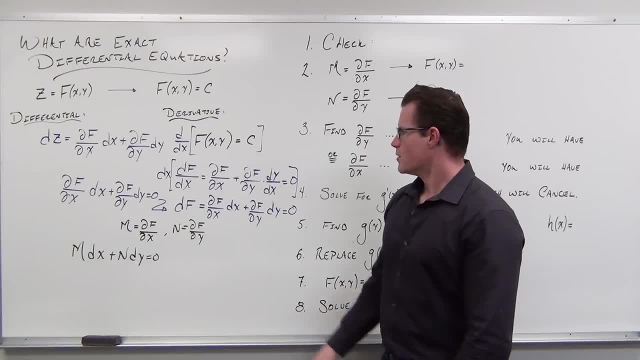 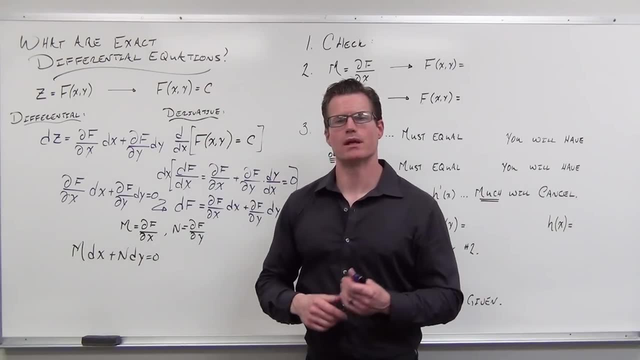 that's the exact differential equation I'm seeing in my textbook. but that right there is representing an exact differential of some sort of potential function. Now here's the issue. and this would be exactly what that differential is. Here's the issue. We're not starting here in. 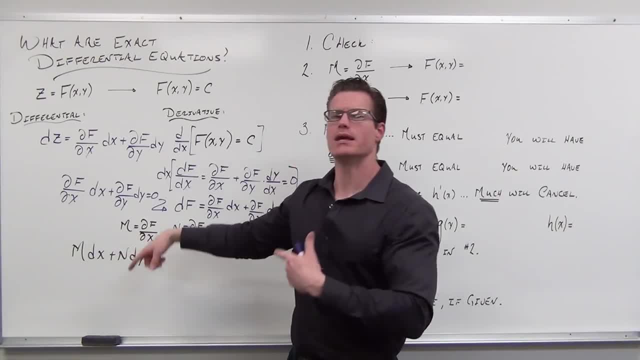 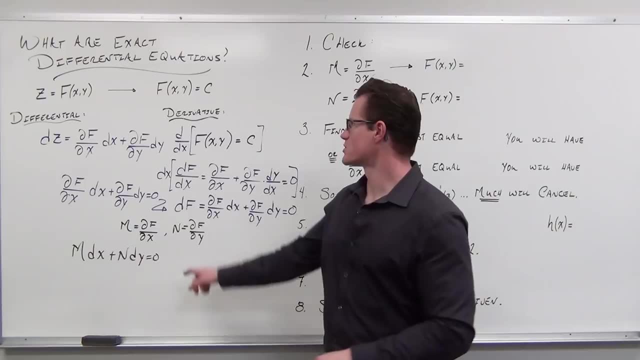 this class and ending here. Where we're starting is here and trying to end with some potential function. So how in the world do we know that this is an exact differential for some potential function? And here's the beauty of it. So I want you to listen real carefully to understand where. 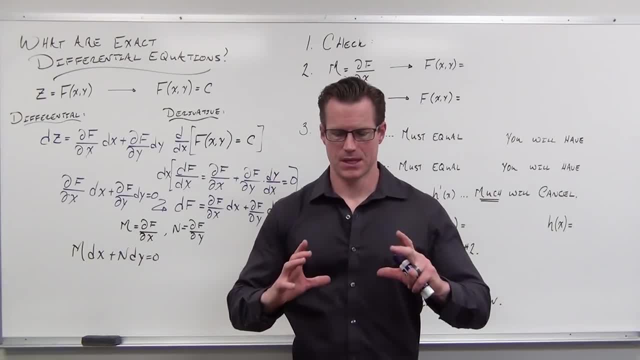 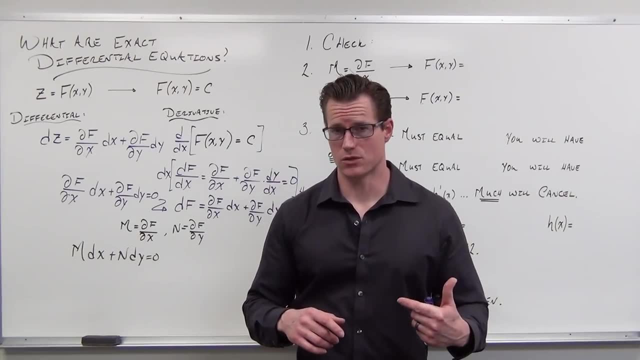 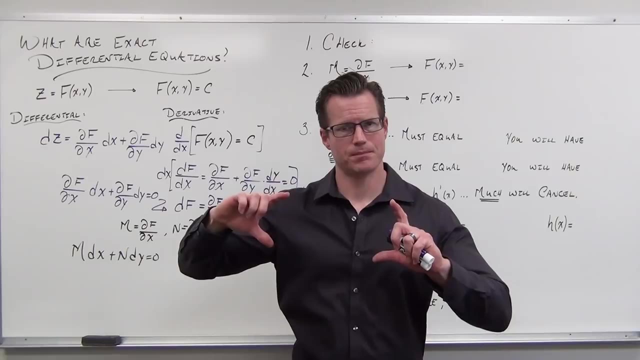 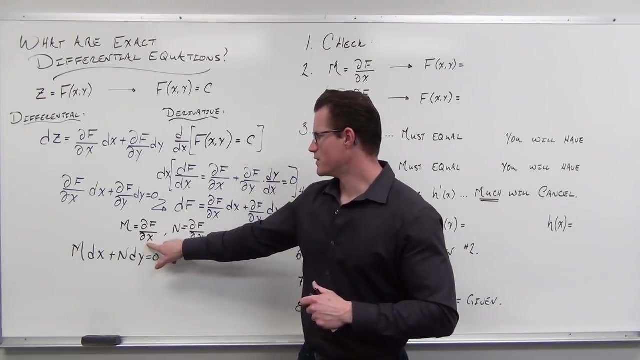 we're coming from. When we talked about continuous and differentiable functions with two variables, we learned something really interesting. What we learned is that mixed partial derivatives are always equal on some sort of a region where our function is continuous and differentiable. Let's say that one more time. So look, this is a partial derivative of f with respect to x. 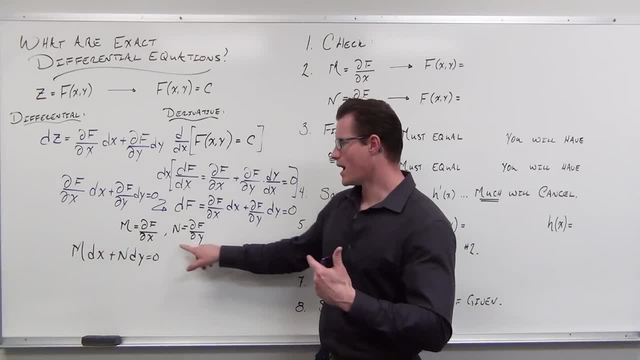 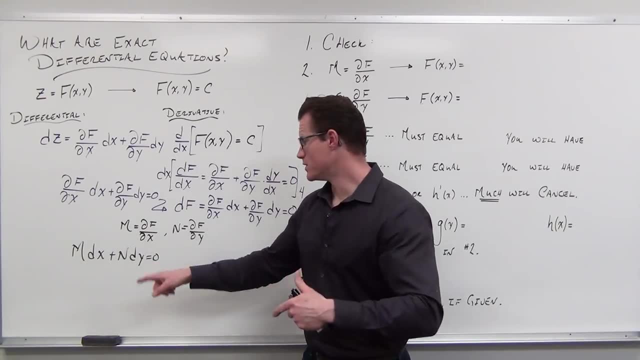 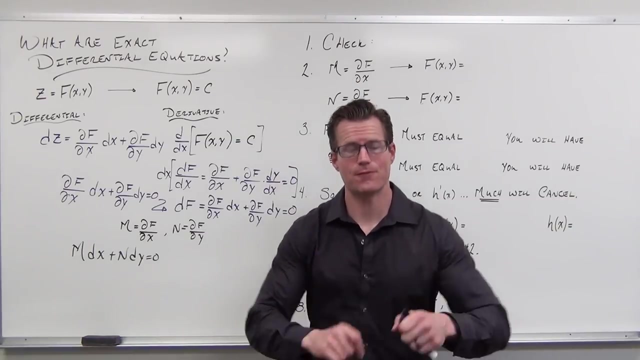 right, That's what m is, And this is a partial derivative of f with respect to y. That's what. that's what n is. If we take another, another partial derivative, this one with respect to y and this one with respect to x, those things have to be equal. if this is representing some. 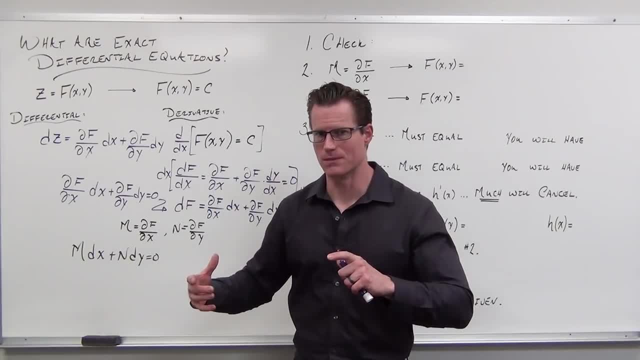 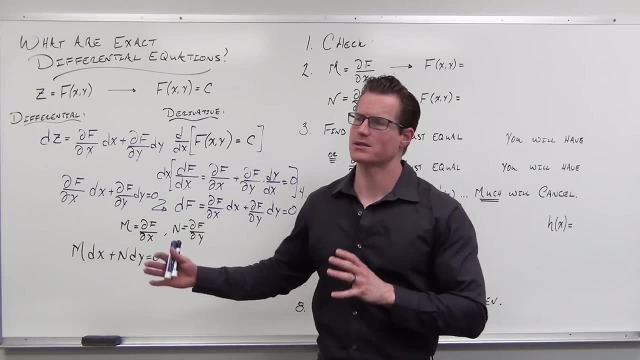 potential function that's both continuous and differentiable on some region. I know that's a lot of theory, but I want it to make sense because I don't want to just give you the how without you understanding the why. That's pointless. It'll work but you'll never really get it. 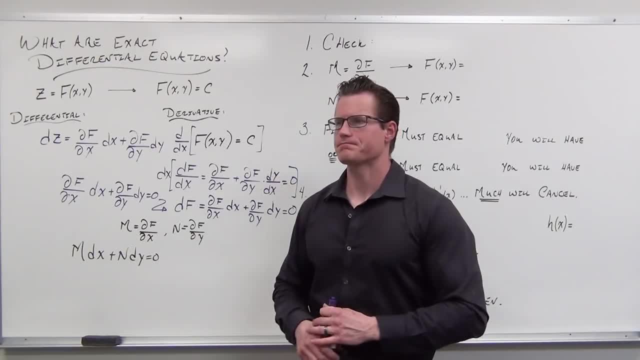 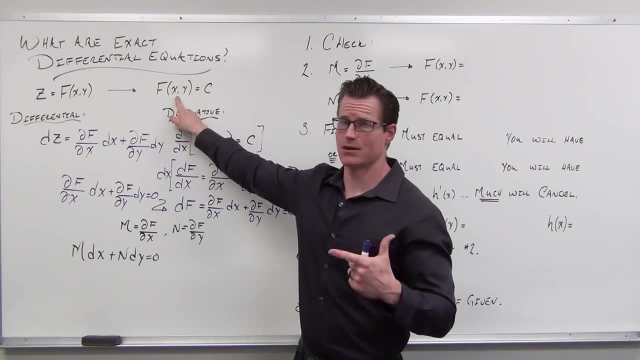 So, so let's, let's get this. let's get this real straight: In order for this to actually work, that function has to be continuous and differentiable on some sort of a region. Do you guys get that Like? it's got to be differentiable, continuous and differentiable for us to even do? 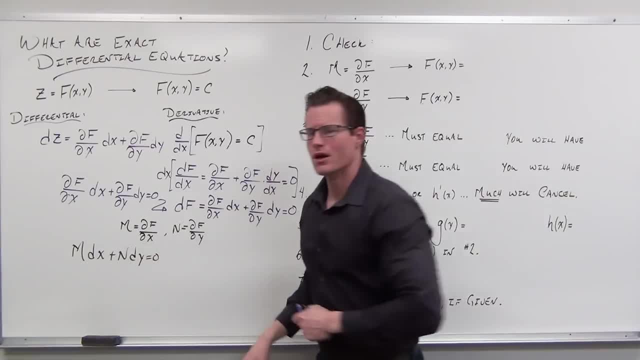 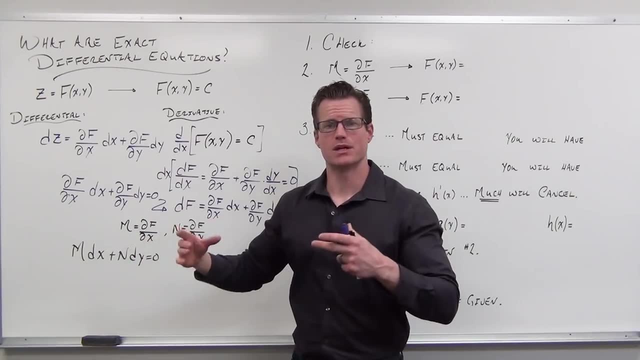 this. So we don't start here, though We start here. So how do we know we're going to be able to go backwards? Well, we know we're going to be able to go backwards if we have these mixed partial derivatives being equal, because we're going to be able to go backwards if we have these. 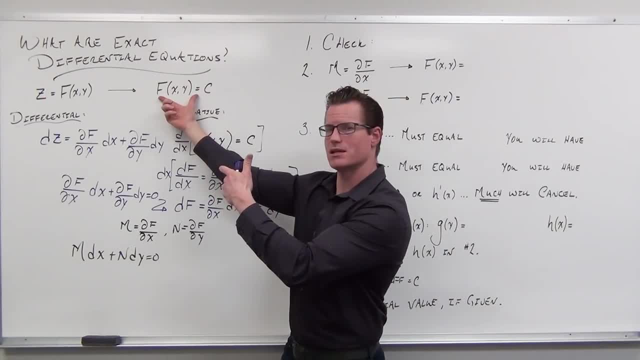 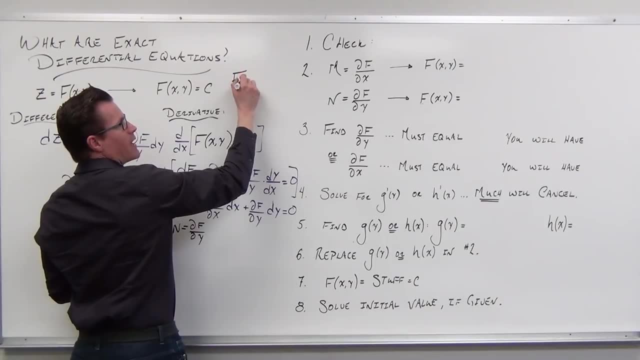 mixed partial derivatives being equal. So what that means is, man, if this is continuous and differentiable on some sort of region, then the mixed partials will be equal. That means if I take the partial derivative of x and then y, it will be equal to y and then x. That has to be the case. 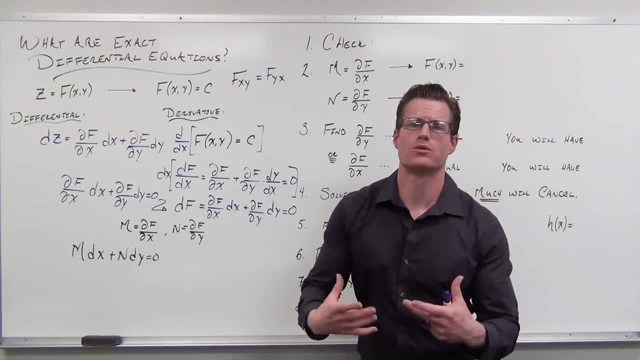 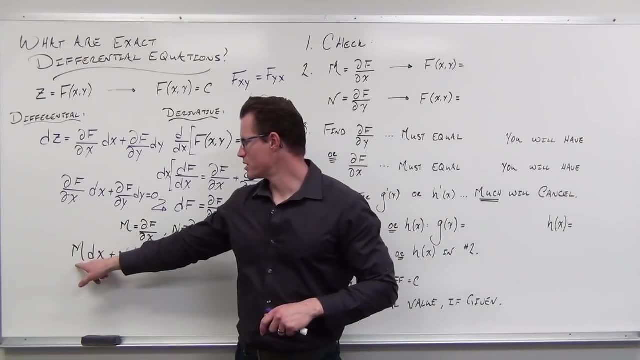 in order for this to actually be continuous and differentiable on a region, for this stuff to work. So when we start here we say there's a test that we can do. If this is the partial derivative of f with respect to x, let's say that we have a partial derivative of f with respect to x. 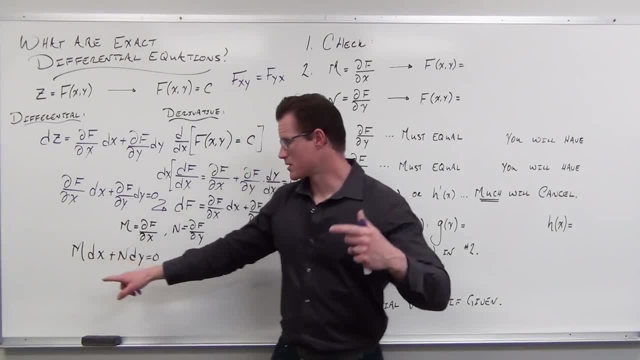 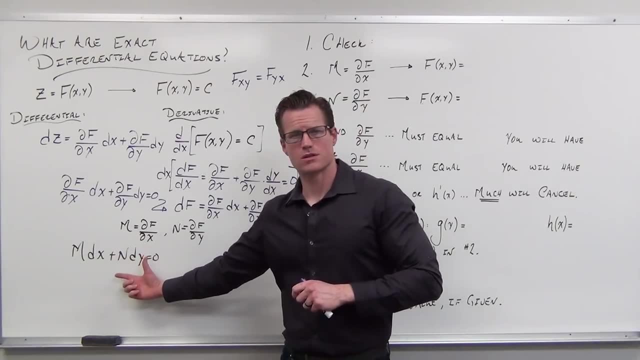 let's take the partial derivative of this with respect to y, Let's take the partial derivative of this with respect to x and let's see if they're equal, Because if they are, that means that this comes from some sort of a potential function that is continuous and differentiable. 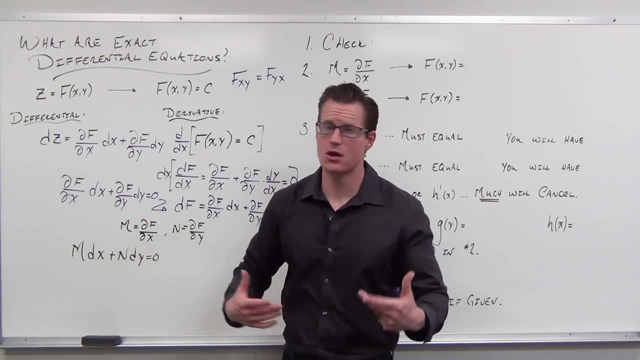 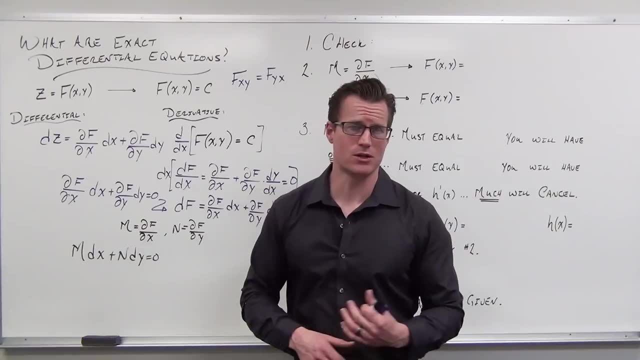 on a region, which means we can go backwards, and there's a way to do that And it's not that hard. In this video, I'm going to show you two techniques. I might show you one. I'll probably change my mind and show you both. I'm going to show you that a lot of textbooks will. 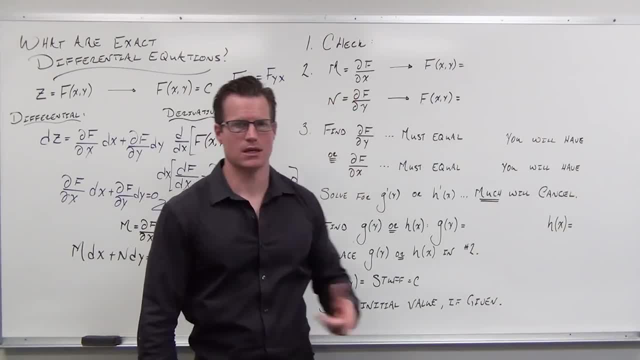 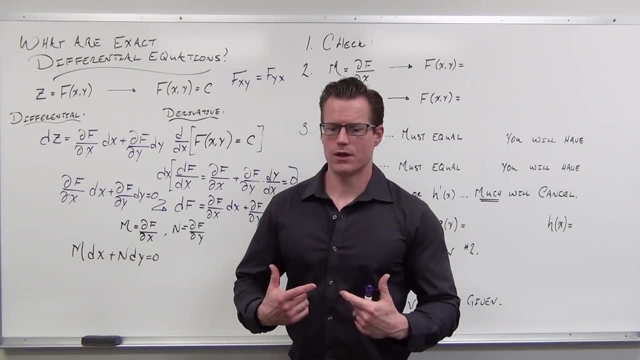 sort of make you choose this one to take an integral of all the time, and you don't have to do that. So I'm going to show you that And we'll practice in the next video. And in the third video I'm going to show you that there is also an integrating factor that we can find. So I'm 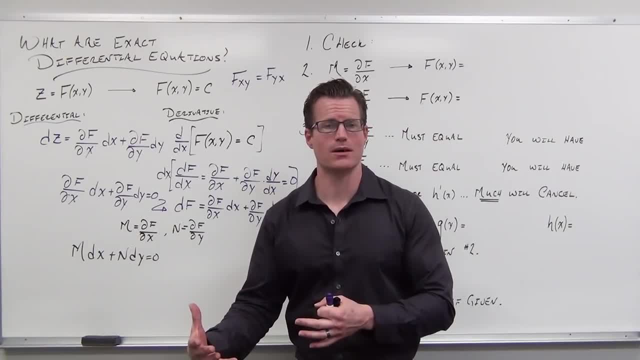 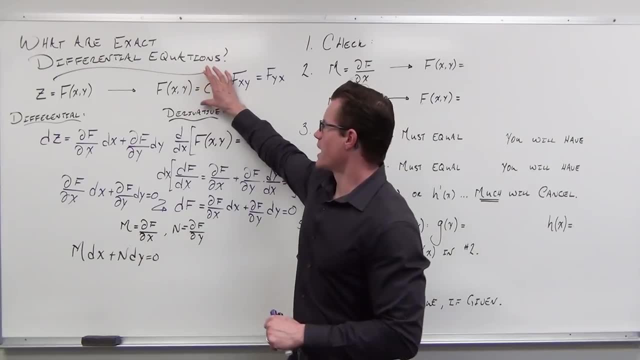 going to give you everything I know about exact differential equations that I can teach you in this particular class. Where we go. the driving thought behind this is: we're trying to get back to a potential function. You're going to be given this So in order to not waste your time. 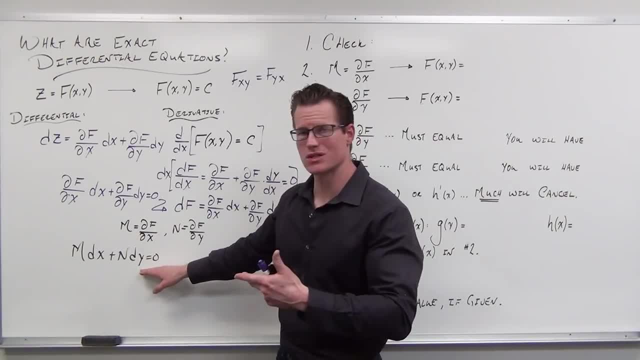 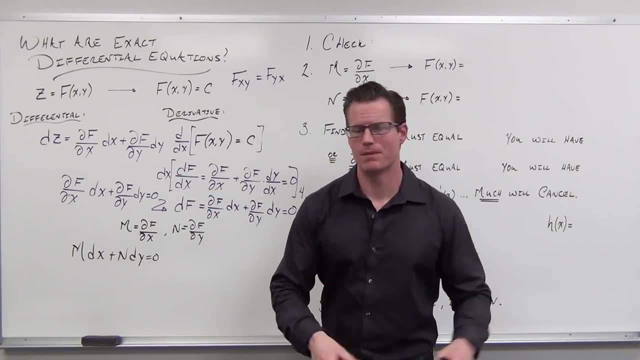 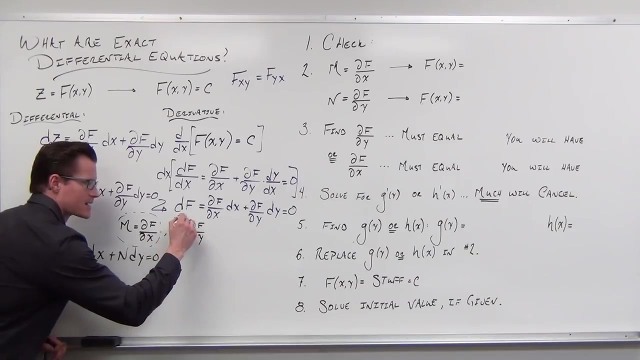 what we're going to do is we're going to test to see whether this actually is an exact difference with equation for some potential function by checking the mixed partials. Then we'll be able to undo it. So how is that going to work for us, Man, if m is the partial of f with respect to x? 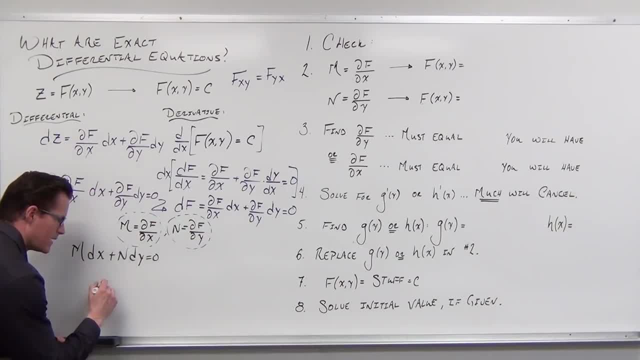 and n is the partial of f with respect to y, then the partial of f with respect to x, and then y is really just the partial derivative of m With respect to y. it's saying: look, the m is already a partial with respect to x. Let's just 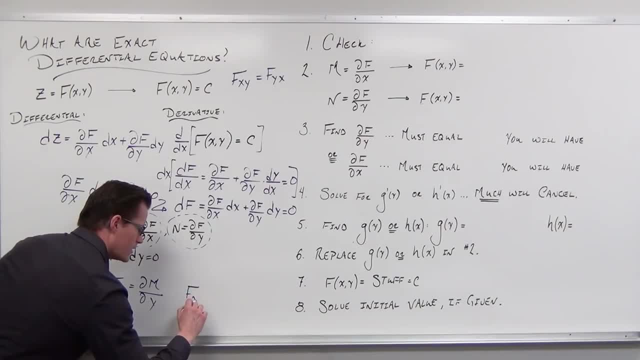 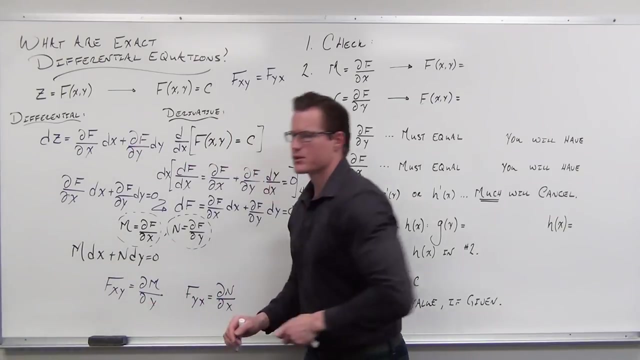 do it again with respect to y And the partial of y with respect to x. well, this already is the partial of f with respect to y. Let's just take that again with respect to x, And these two things are equal. This is the great point. If these two things are equal, it means that this: 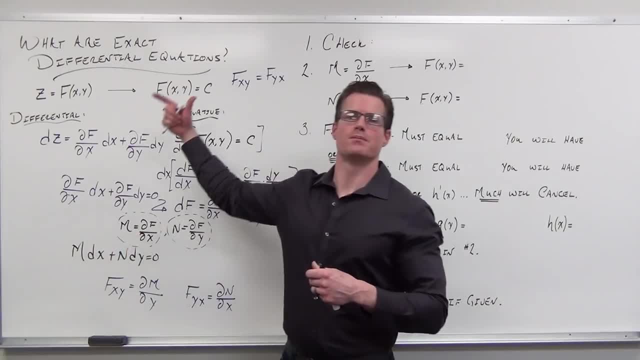 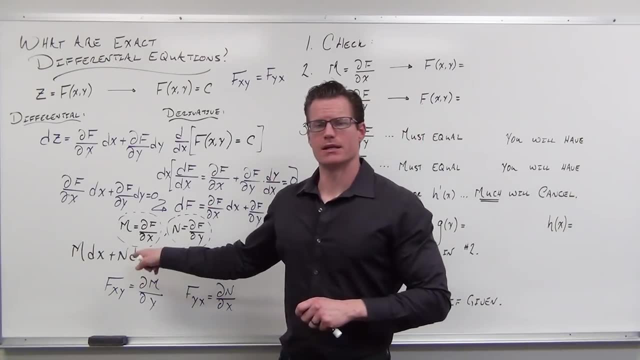 is representing an exact differential equation from some potential function, And then we can go backwards. What if these aren't equal? Well then, this is not an exact differential equation for some potential function, And we'd have to either A say it's not possible. 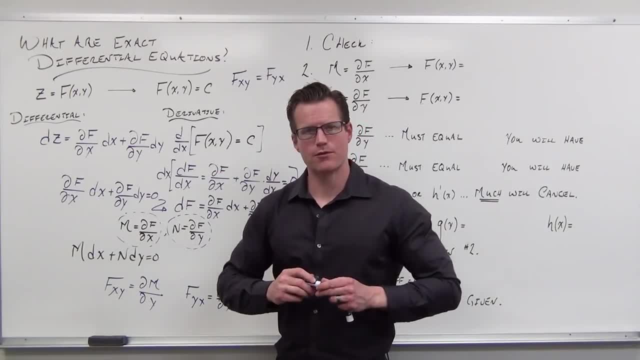 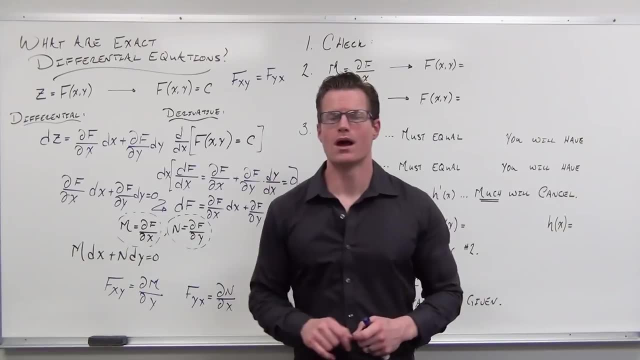 or B. theoretically it is possible with some sort of a function that we can multiply, And so we can make it an exact differential equation with something called an integrated factor, And we've had that before. That's going to be in the last video about exact differential equations. 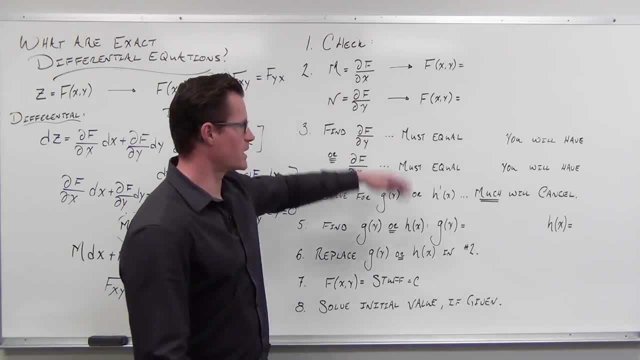 So let me start here. How in the world are we going to do it? I'm going to give you some steps right now. I'll talk about both methods that you can use to go back, And then we're just going to practice two. 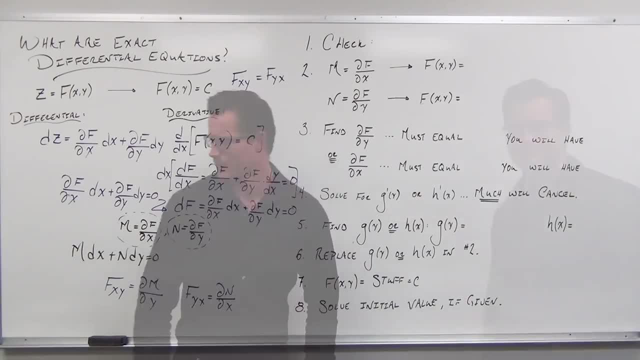 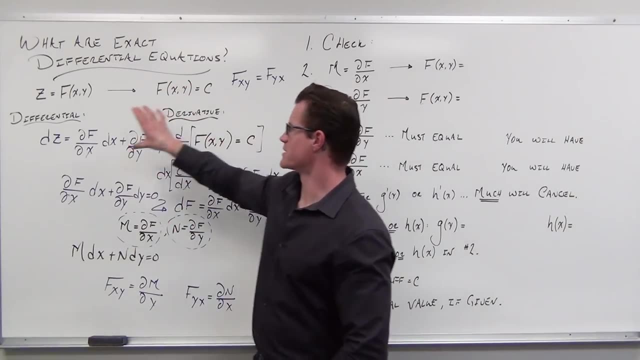 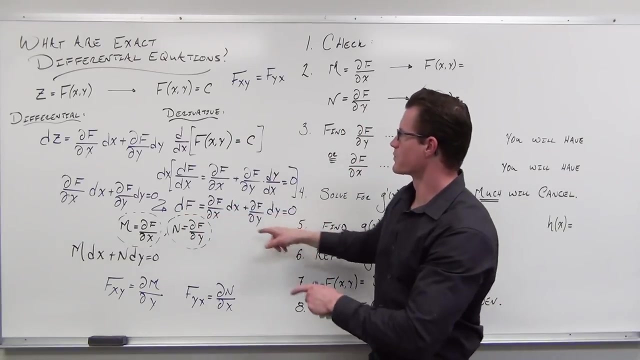 examples And we'll continue with that. OK, so hopefully I've explained this well enough for you to understand that. you understand where we're coming from, that you understand. this is a differential form. I'm sorry that this is the differential for this function. This right here is the total differential for this function. It. 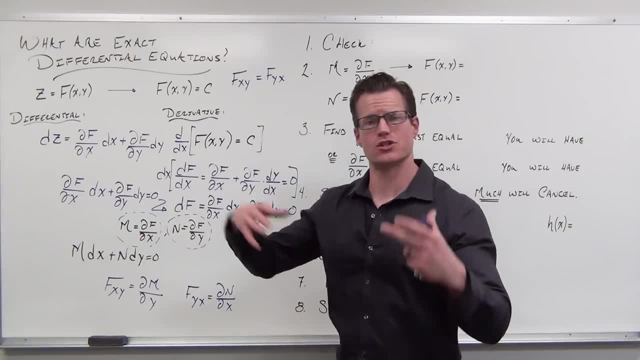 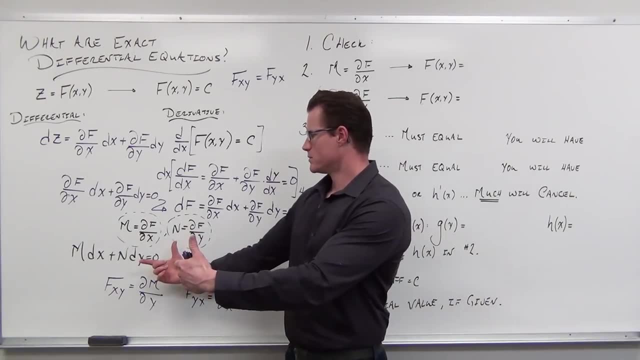 ends up being the same, if you let that be said, If you set equal to a constant. there's two ways to come down to that idea. What we also learn is that mixed partials are equal. So in this differential, exact differential equation, if our mixed partials 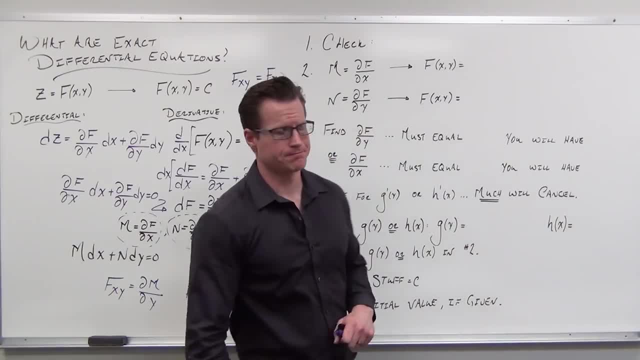 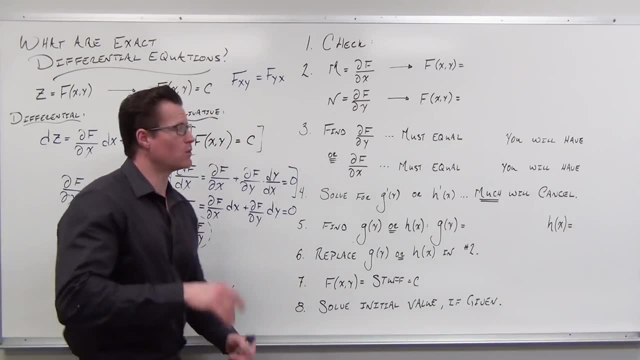 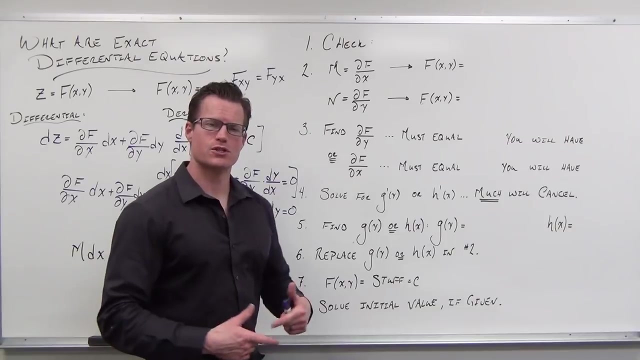 are equal. it's coming from sort of some sort of a potential function that we can go back to that is continuous in differential quantum region. Now let's suppose that we don't start here. We want to get here. Let's suppose we start here, at this exact differential equation, The first thing we want to 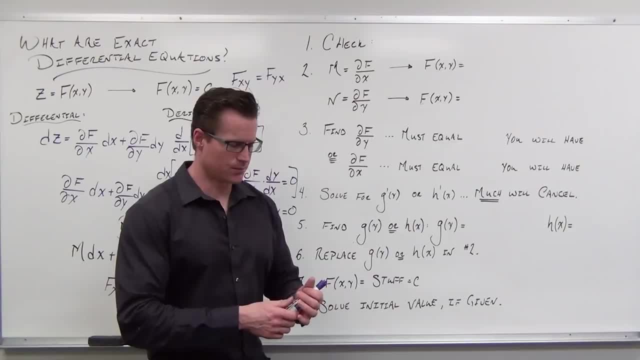 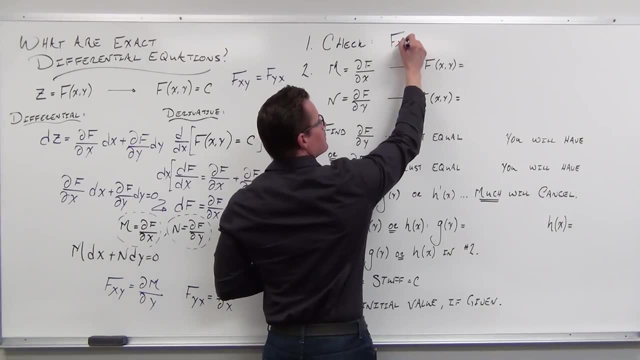 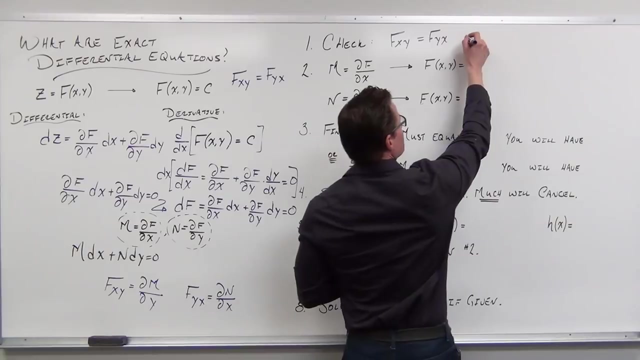 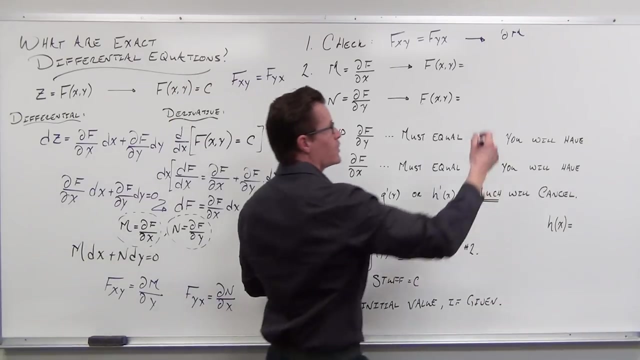 do is we want to check. We want to check the partial, the mixed partial derivatives here. So we want to check: Is that actually true? Which means, since n is already the partial derivative of f with respect to x, we just have to take that and do it with y. And since n is, 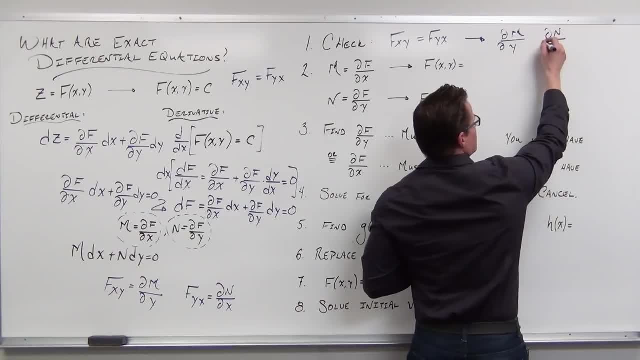 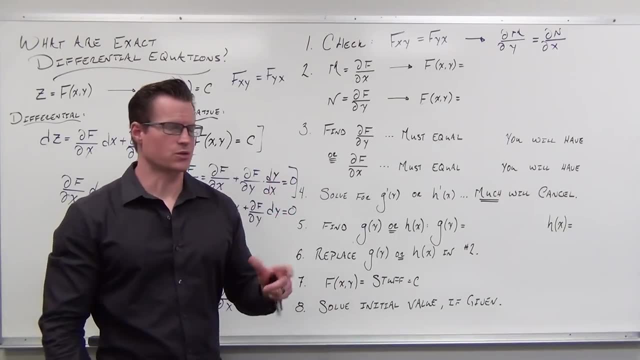 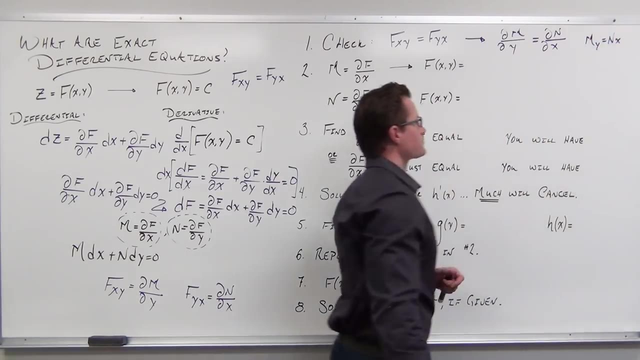 already the partial derivative of f with respect to y. we just have to take that and do the partial derivative of n with respect to x. Those right there represent our mixed partials. You could even see it like this: Partial derivative of n with respect to y must equal partial derivative of n. 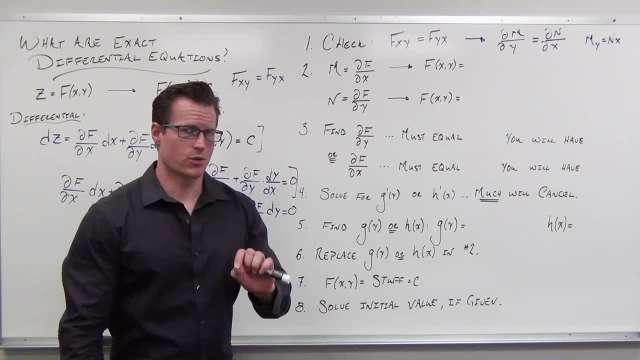 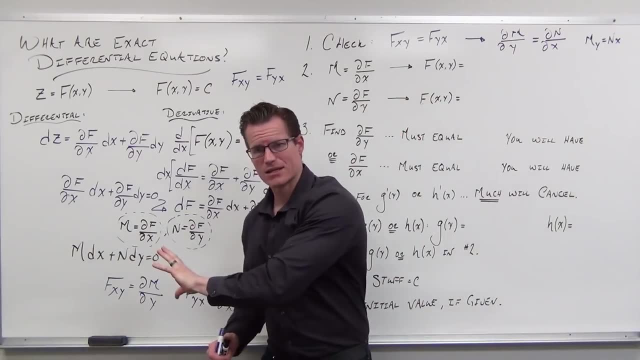 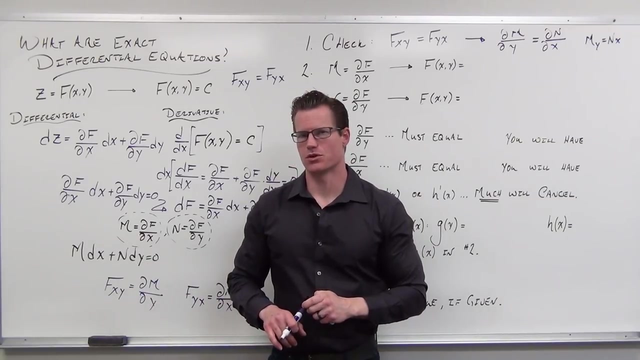 with respect to x, if this represents an exact differential equation. So get this real clear: If this, if this actually happens, then this is an exact differential equation of some potential function. So, like right off the bat, you don't just start calling this an exact differential equation. A lot of 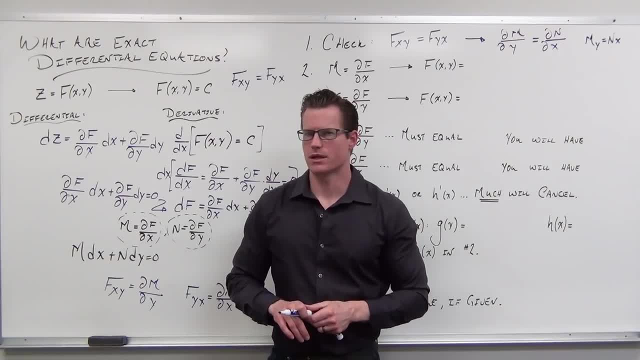 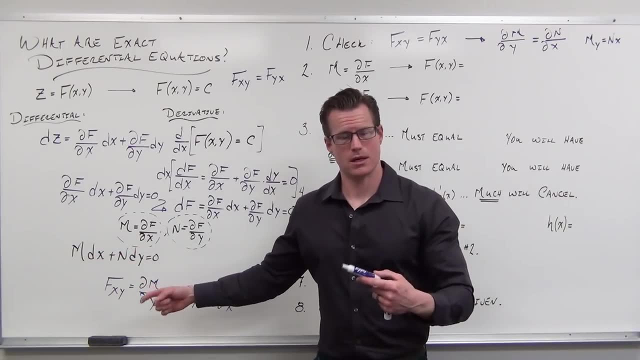 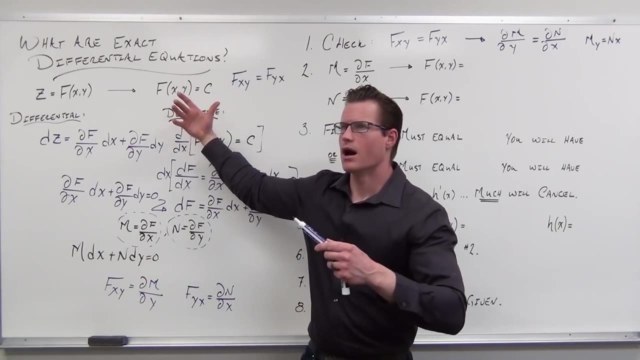 people do They go: oh, that's an exact differential equation. No, no, not necessarily It is if the mixed partials are equal, Because if the mixed partials are equal, then it's representing the exact differential for some sort of a potential function, Not the other way around, Not not this. 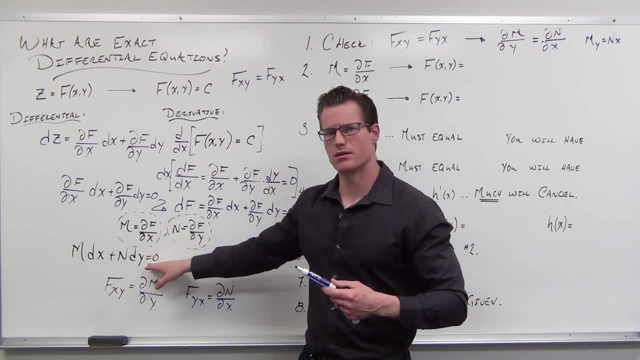 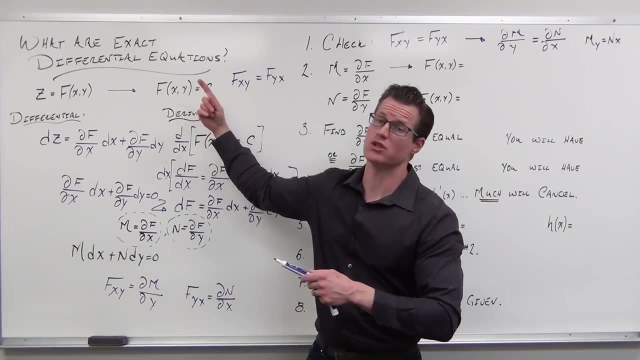 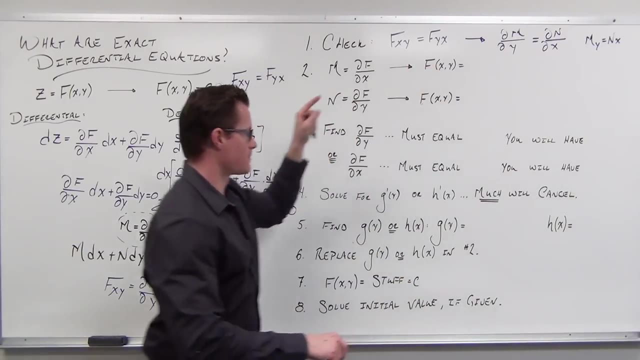 way Not. well, this is an exact differential equation. Therefore, this has to be true. No, no, no. This being true says that's an exact differential equation of some potential function that we can now find. So we check this and it says, hey, if that happens right there, if that happens, then this right here is. 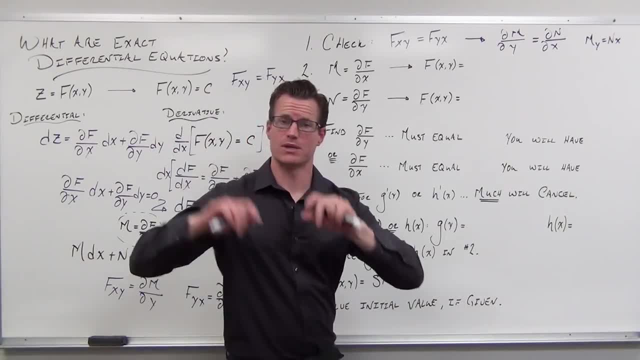 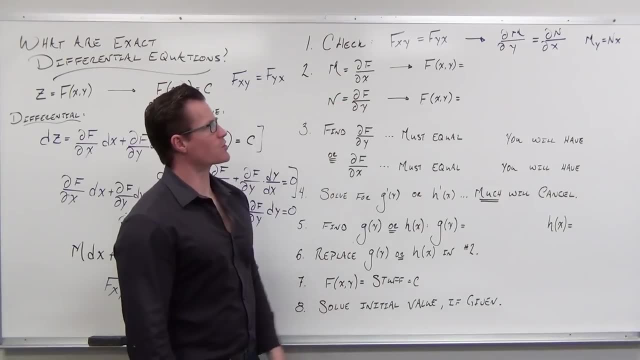 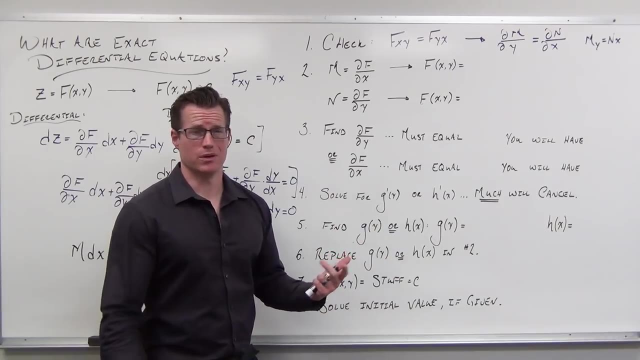 representing the exact or total differential for some potential function. Let's find the function. How do we do that? Well, let's think about it. If m represents the partial derivative of f with respect to x, how do we go back to f? How do we undo derivatives with integrals? How do we undo? 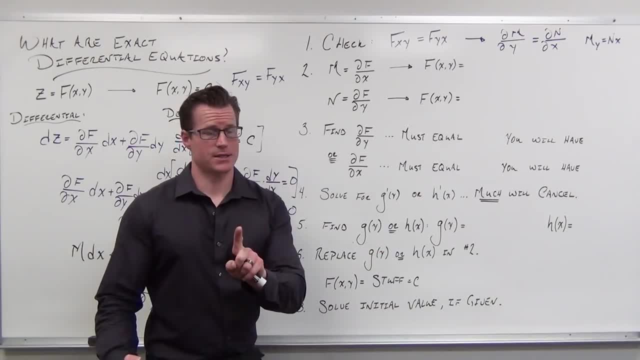 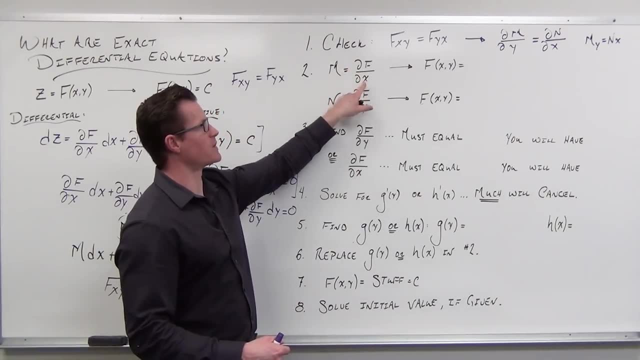 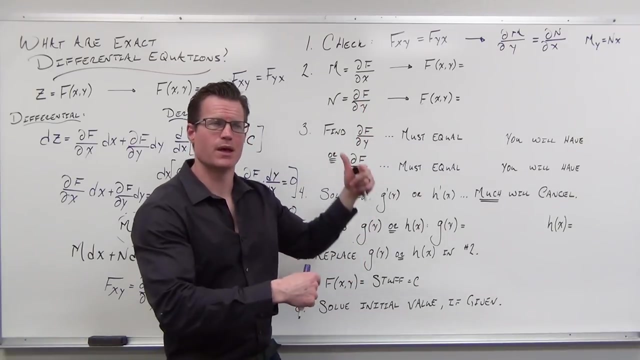 partial derivatives with integrals, but everything with the partial derivative that's held constant. For instance, if we took a partial derivative of f with respect to x, we held the y's as constants. So when we do this integral of this partial derivative, when we get that back, we have this: 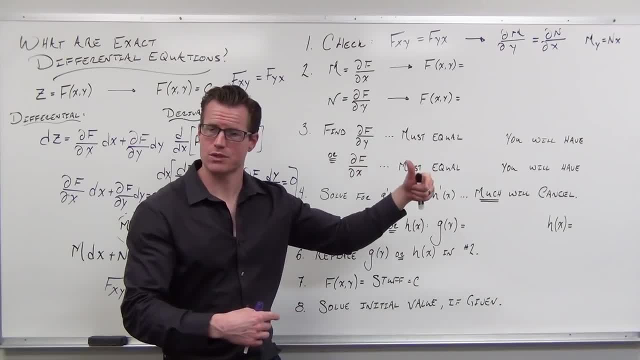 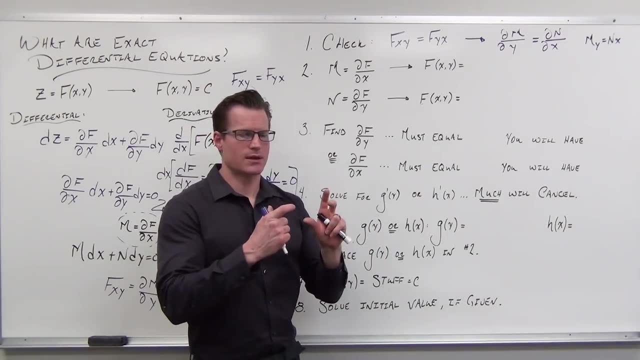 idea that there could be a whole lot of partial derivatives that are constant. So if we take a lot of terms with y's in them, that would have been canceled out. and I'll say this one more time: when you take a partial derivative of a function, everything that's not the variable under 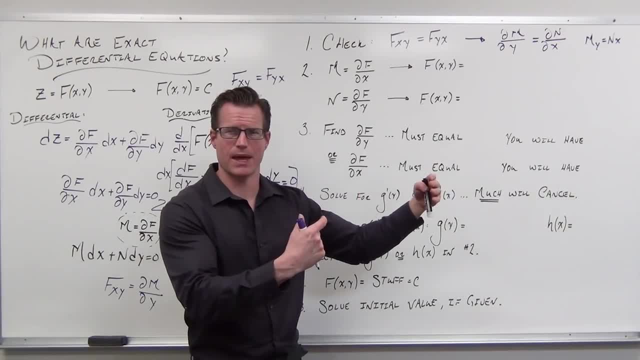 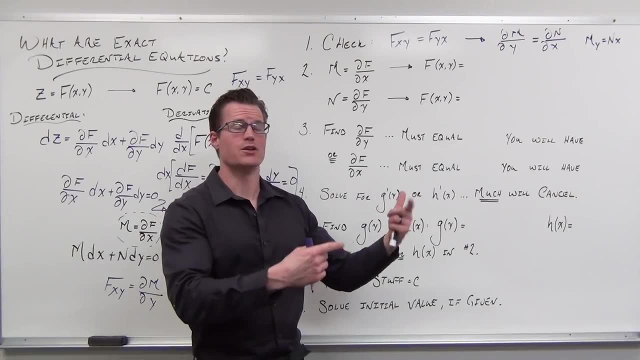 consideration goes to zero if it's a term. So, like x plus y, take the partial derivative of x, that y term goes to zero. Well, if I'm going to undo that derivative, I'm going to undo the partial derivative. then, yeah, I can just find an integral. 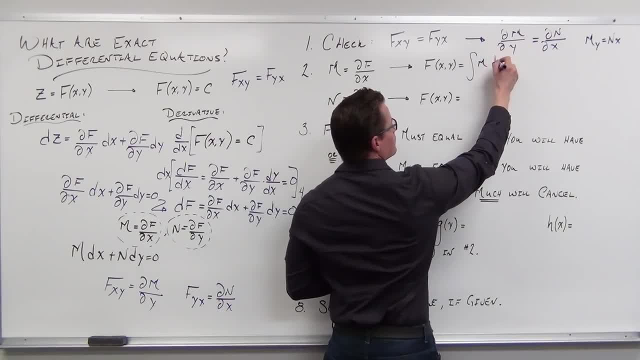 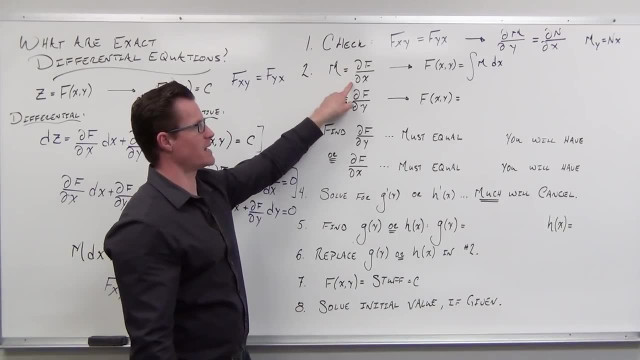 with respect to x. That seems pretty, pretty logical. This is going to say: well, hey, m is the partial of f with respect to x. How do you undo derivatives? Do an integral with respect to whatever variable you did the derivative to. 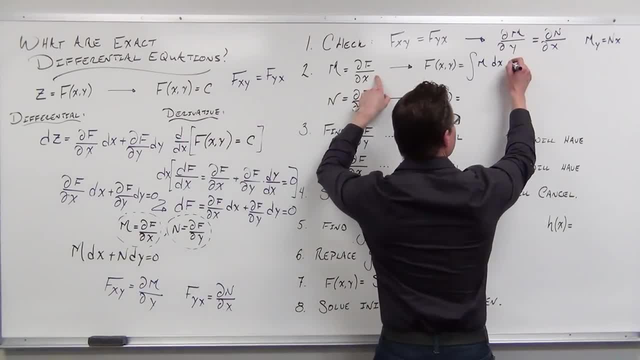 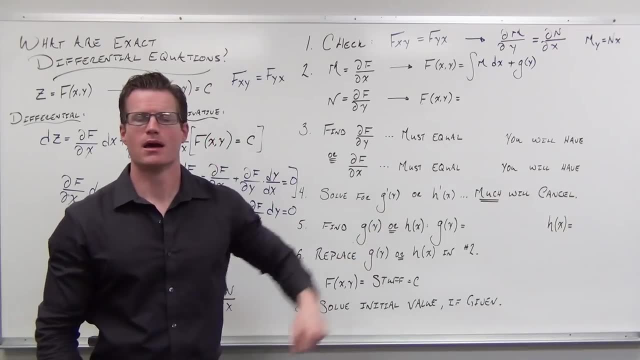 But since it's a partial, I very well could have a function in terms of y. that would be completely annihilated. Imagine it If I took a derivative of this piece. this is all going to have x's right. All of it's going to. 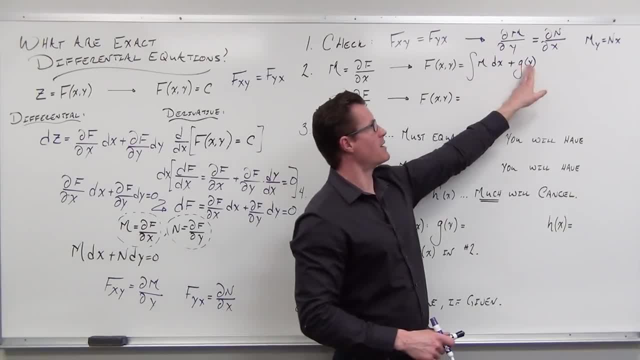 have x's, You're going to be able to get the partial of f with respect to x. So if I take a everything over here that has no x's, just terms of y, that's going to go to zero, And so we have to. 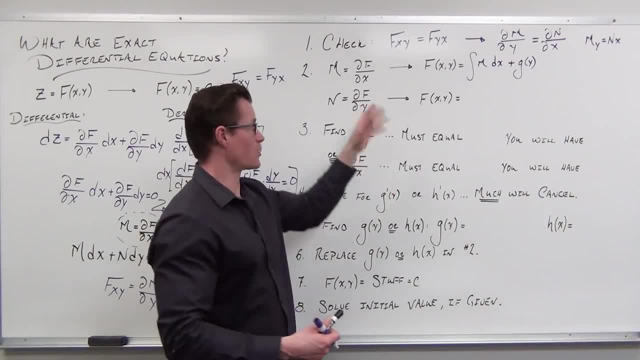 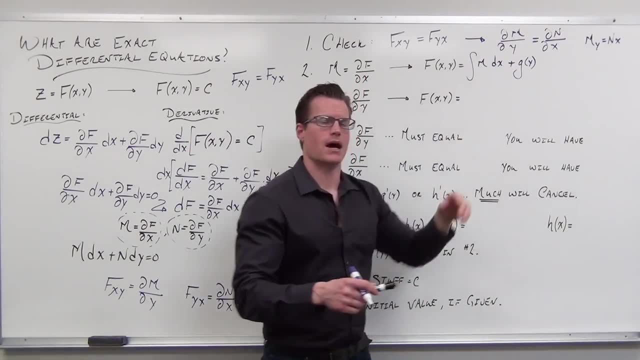 represent that. I hope you're getting that Like: if you have a partial of x- sorry, a partial of a function- with respect to x, your y's are gone. We've got to show that doing an integral would give us something of y. Now most of your textbooks are going to end right there and say: 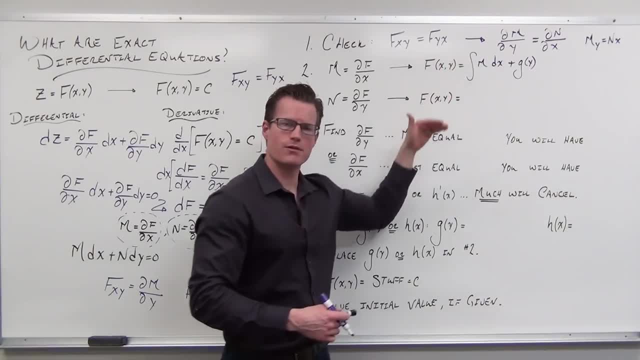 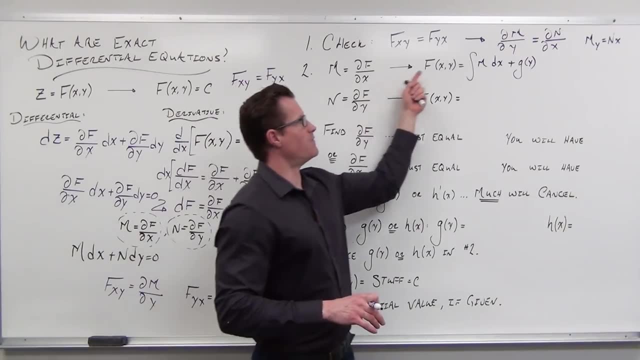 that's all you need to know. Then what we do is we take a derivative of this piece and then we set it equal to n and then you're good to go. And that is true. But sometimes this can be very challenging, And what some of the textbooks don't tell you is 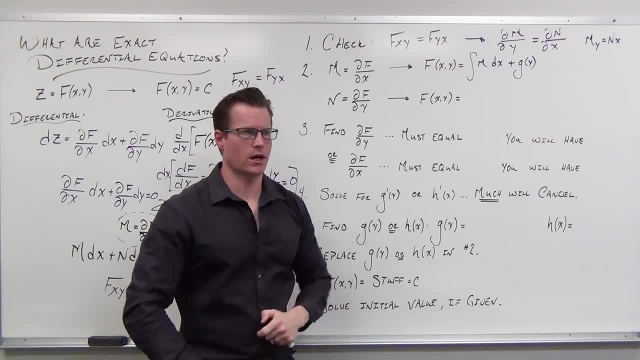 you can actually do it another way. So instead of just saying: well, I got to take the integral of m, I have to do that. I have a g of y and that's really hard. What have we thought about different? 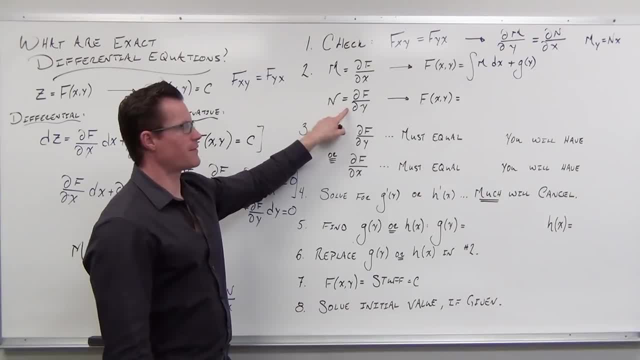 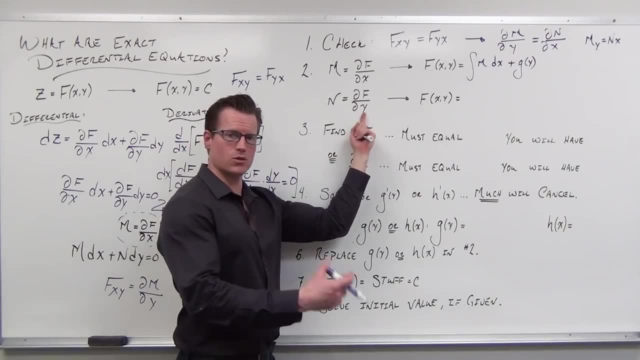 What have we thought? Wait, wait, a minute. If n is the partial derivative of f with respect to y, could we find the same exact thing by saying: let's undo that derivative with respect to y, Let's do an integral of n, this time with respect to y? 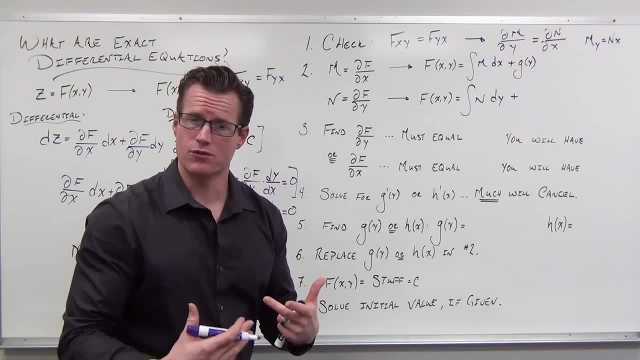 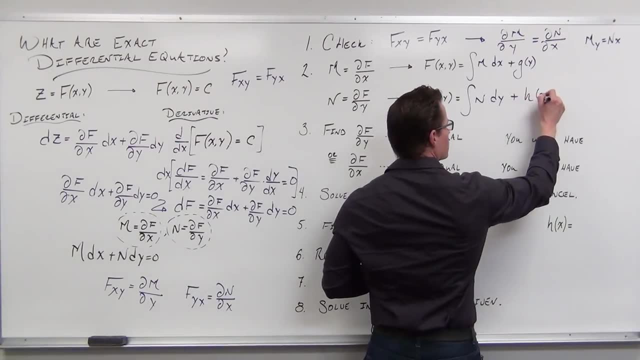 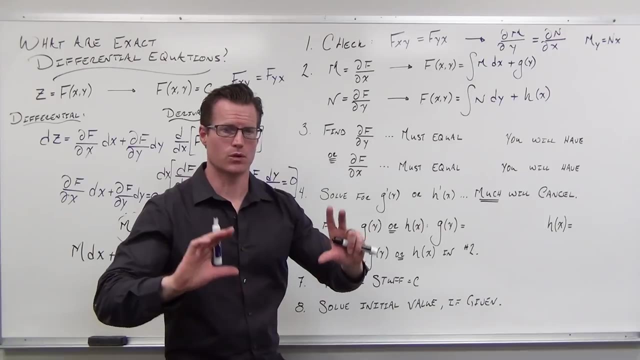 But keeping in mind that you're going to have this function of x that would have been knocked out when you take a partial derivative. So we check, We go: hey, if that's equal, that is an exact differential or total differential for some sort of potential function, We go. well, what's that mean Then? this is the partial of. 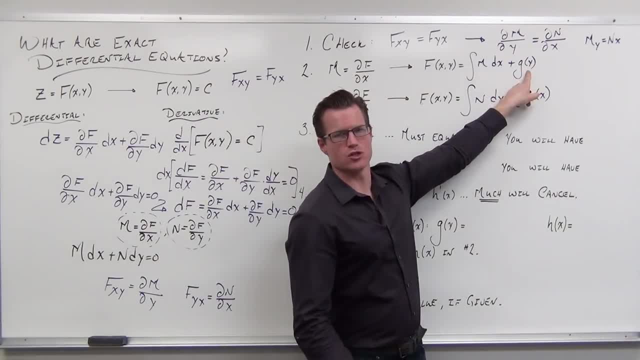 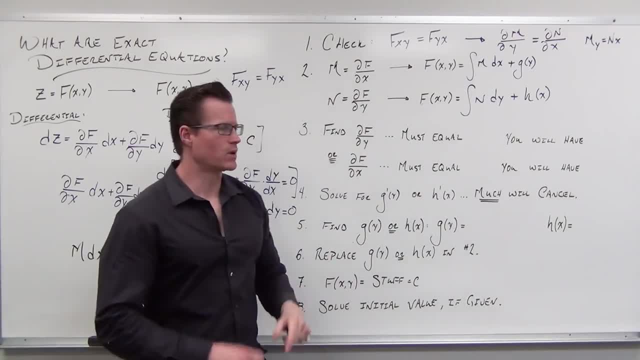 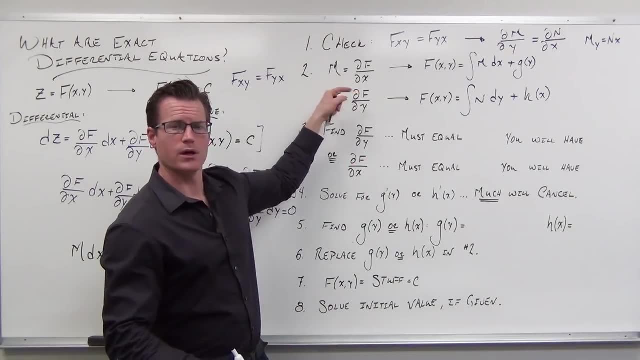 But we're going to have a function in terms of x. Now, that seems well and good, but you're thinking, by the way, just so I'm real clear here- you don't do both, You don't do both. You look at this and 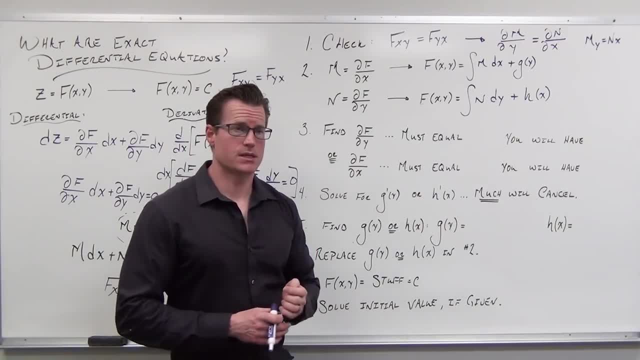 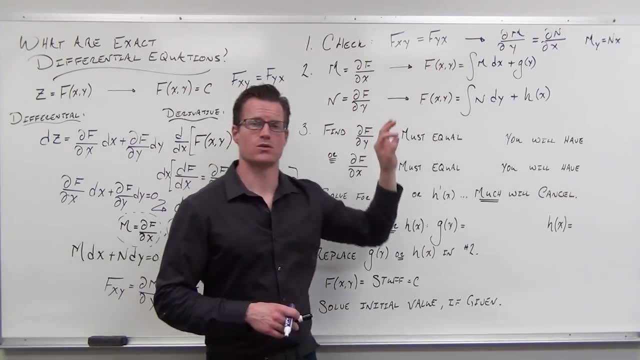 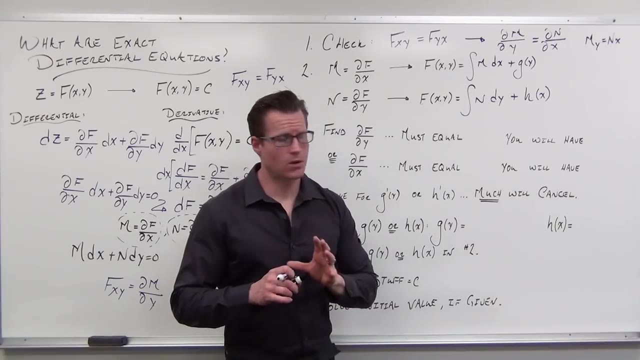 you say which one would be easier to deal with. Is it easier to look at the integral of m with respect to x, Or is it easier to look at the integral of n with respect to y? Again, m with x or n with y? which integral would be easier? And you do that one. You don't need to do both. It's. 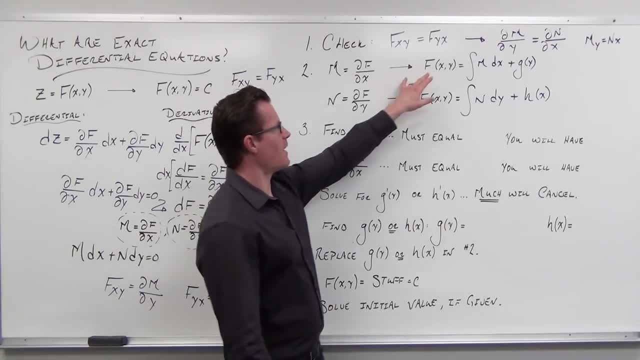 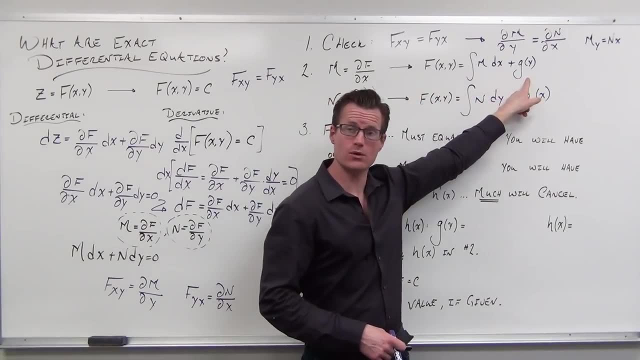 one or the other, And then you go: well, but wait though. I mean, this is the function of f with respect to x. This is exactly what we're trying to find. This is it, But there's half the function. I don't know. But here's the beauty in this technique. If you take an integral of m with 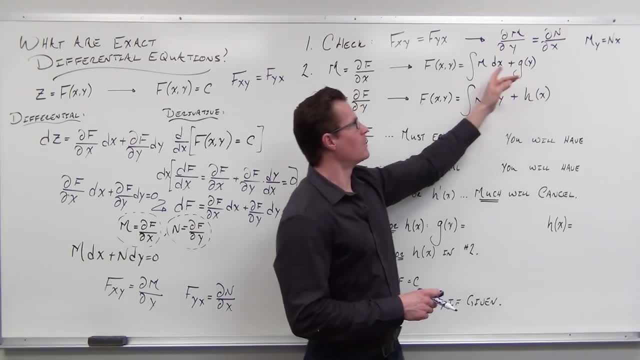 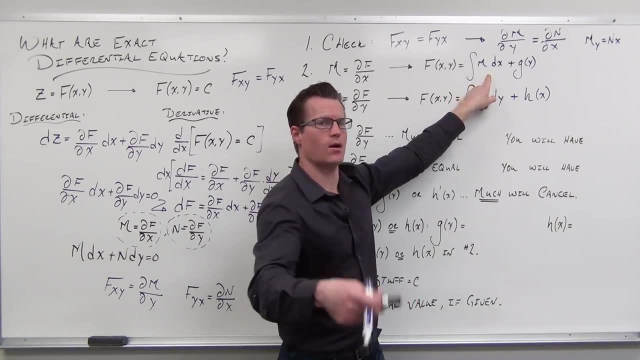 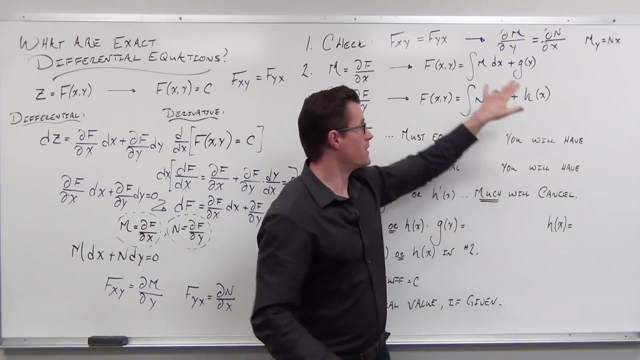 respect to x and you get a function of y. well, what about this? What if we took this and took a partial derivative of this piece with respect to that y? So we're integrating x. We could say some y's, we don't know. Let's take the partial derivative of this function. whatever we're going. 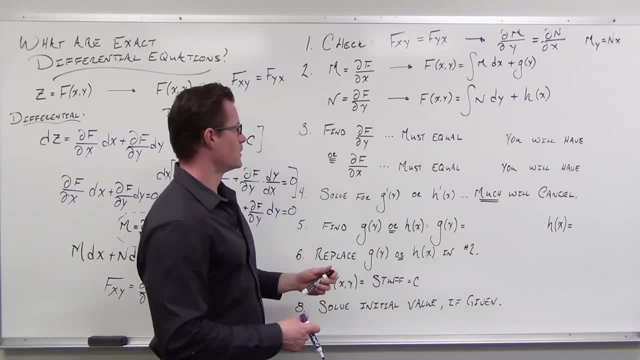 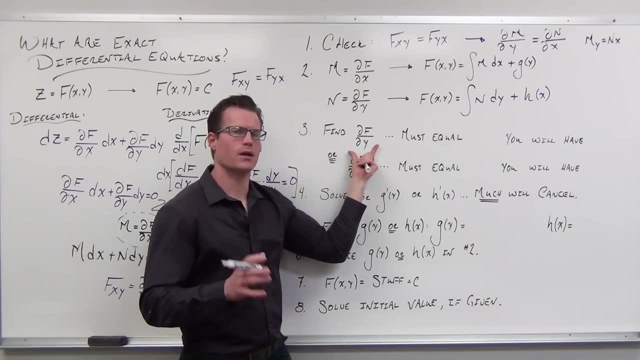 to get with respect to y. All right. Then, if I take the partial of this with respect to y- that's what I'm doing right here- Well, this must equal. think about it. What must it equal? If I take the derivative of f with respect to y? if I take the derivative of f? 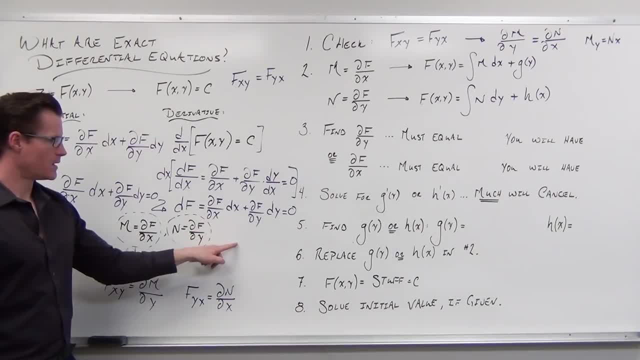 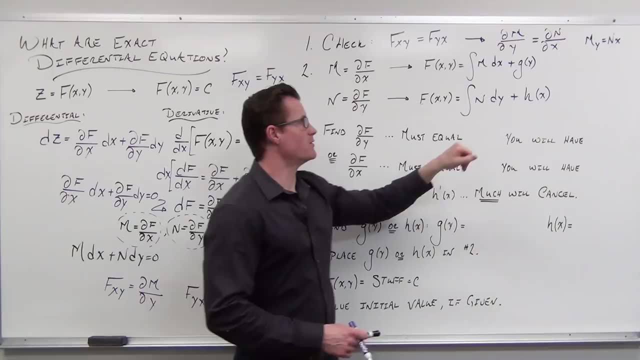 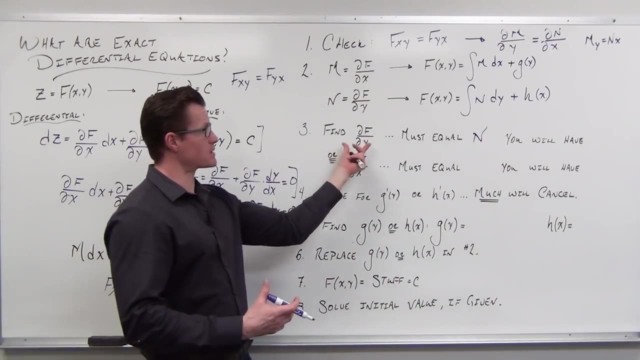 with respect to y, it has to equal m. So the idea is: take your m, do an integral, tack it a y, Take a derivative, and then that derivative, with respect to y, must equal n. It has to. That's what this means. That is the n that you're seeing on your work. 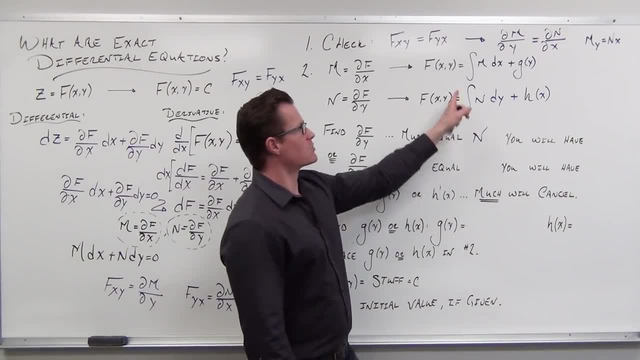 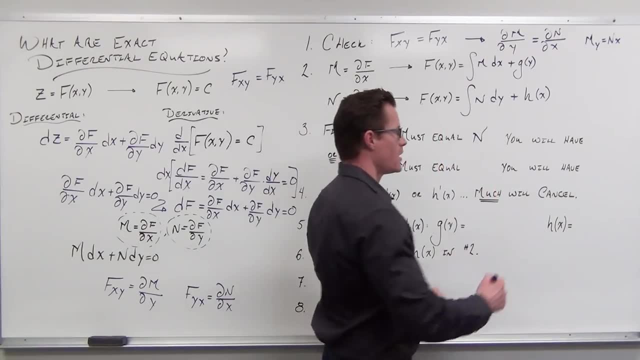 right now. Also, when you do this, if you take a derivative of this with respect to y, you're going to get a g prime of y, the first derivative of whatever that function is with respect to y, Isn't it Likewise? 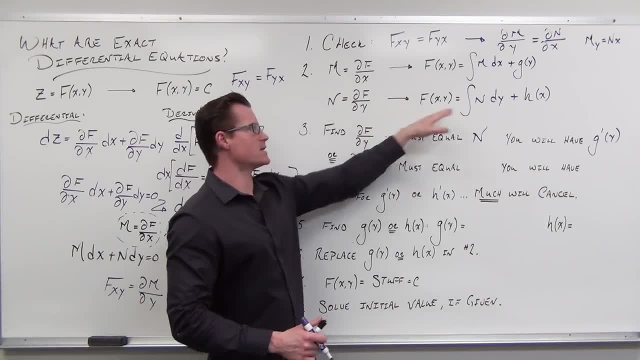 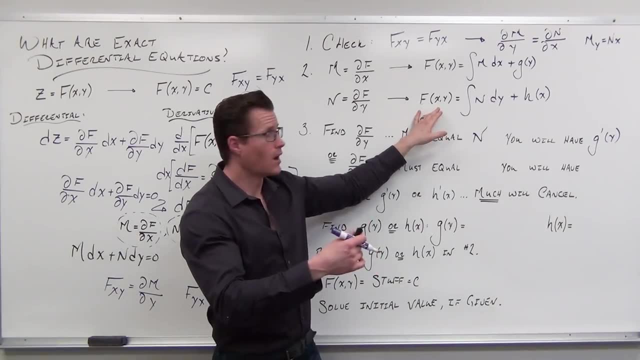 the other way we can think about it. let's say: you did this one because that was easier. Okay, great, Right now, this is the function of f. This is what the function you're looking for. This is the function that you're looking for, but you don't know the x's. Well, we do have. 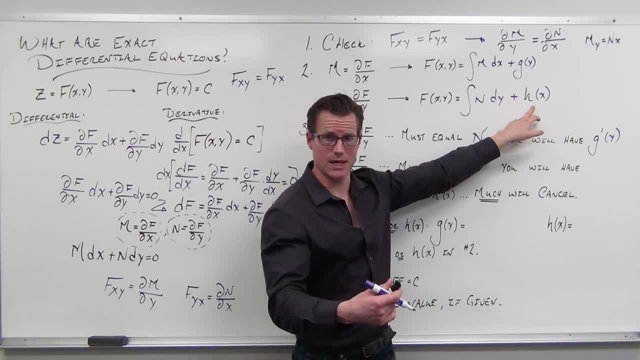 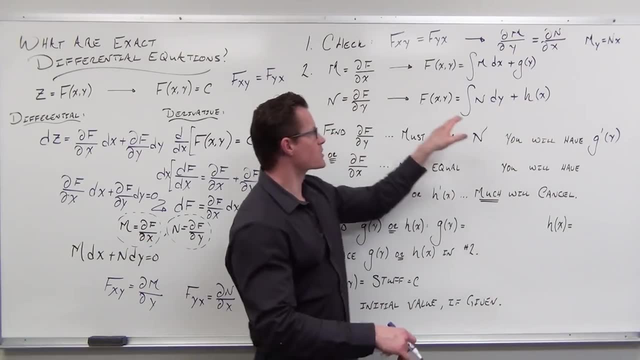 something that we understand about the derivative of f with respect to x. We understand that the derivative of f with respect to x is m. It's the same thing. So we say: all right, well, now that we've integrated with respect to y, we're going to integrate with respect to y, So we say: all right. 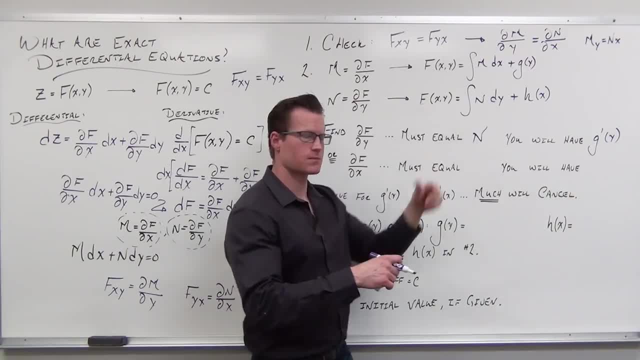 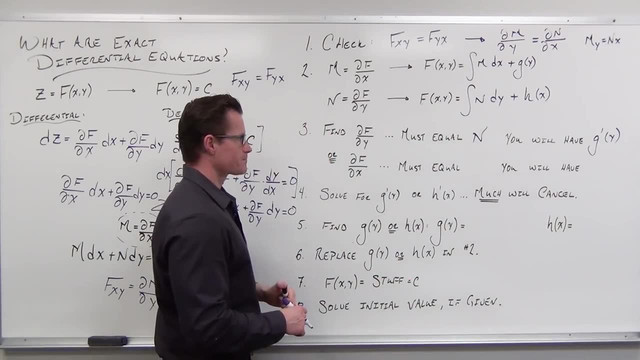 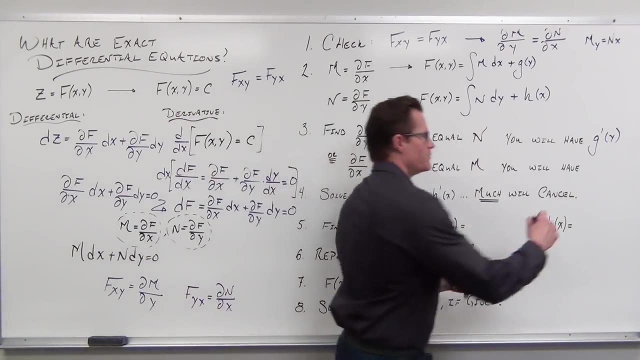 well, now that we've integrated with respect to y, let's take the derivative with respect to x. So we're going to have this thing, derivative whatever it is, with respect to x, and it's going to have to be equal to m. You're going to get some derivative of that function of x. 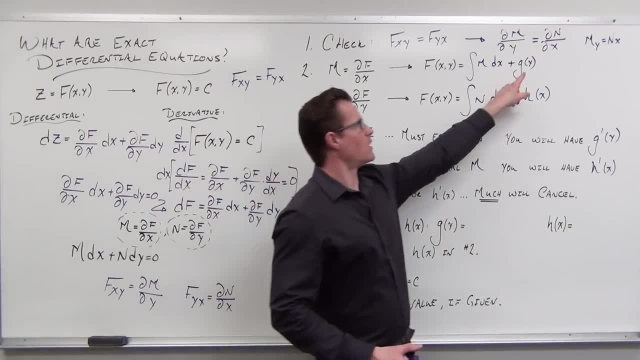 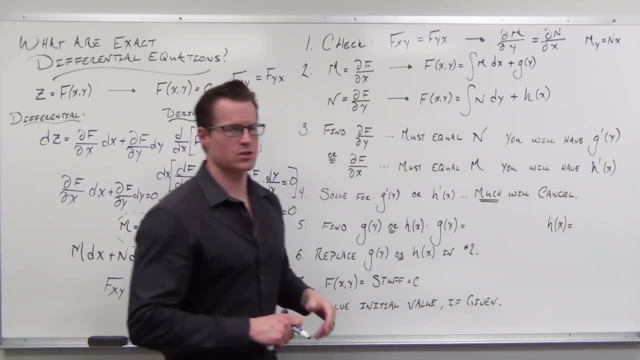 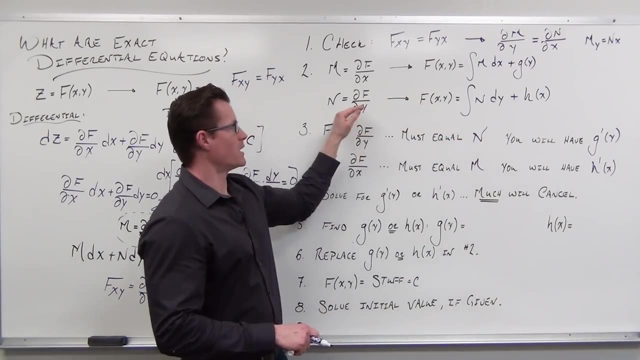 A couple questions that students always have. Is this always going to be only y's? Yes, Is this going to be only x's? Yep, So long story made real short. integrate m with x, then take a derivative with y instead, equal to n. or integrate n with respect to y, take a derivative with respect to x. 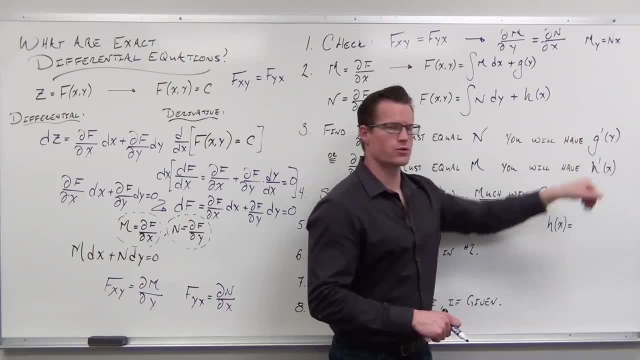 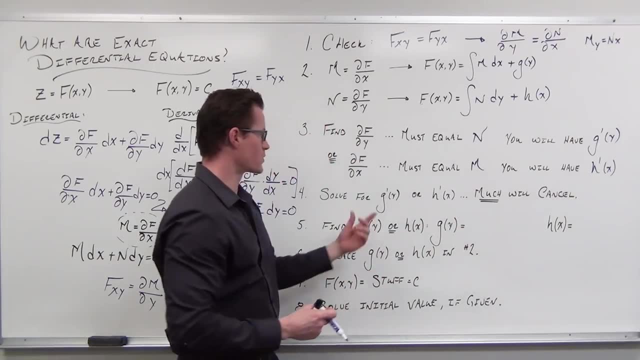 instead equal to m. You're going to have some sort of a derivative in there. Solve for that derivative. So you're going to. you're going to have these set equal. you're going to solve for that derivative. So solve for g prime of y, or solve for h prime of x, and lots of stuff is going. 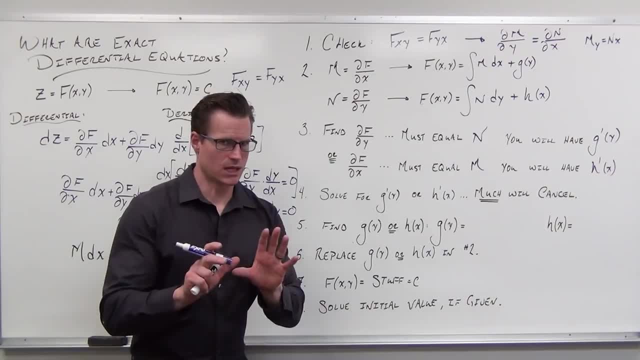 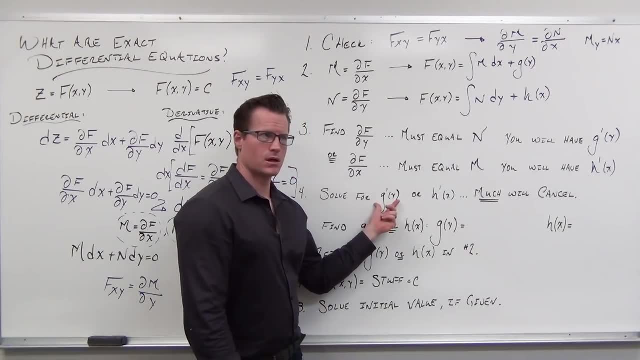 going to cancel, typically, So you'll get something that's nice. Now, again, when you solve for this, should this be in terms of y only? Yeah, that's kind of the point, right, Because you have a function of y's. Should this be in x's only? Yes, Now how do we undo? So you solve for this. 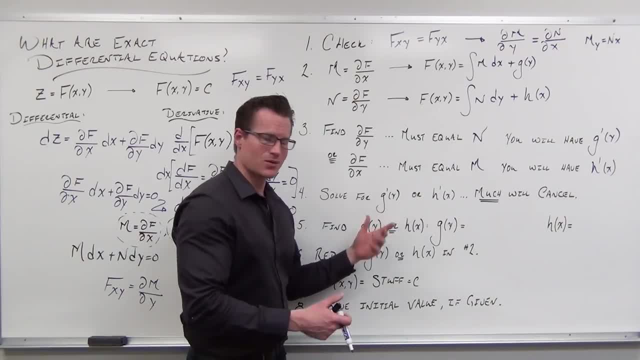 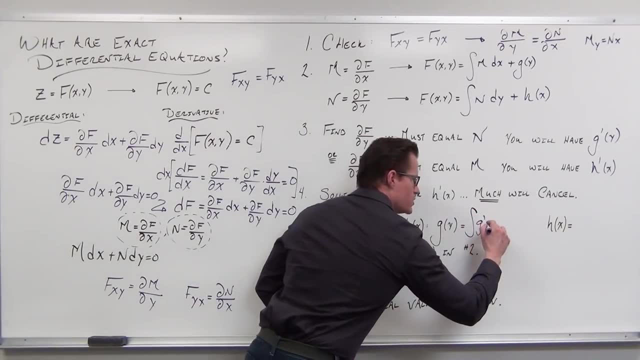 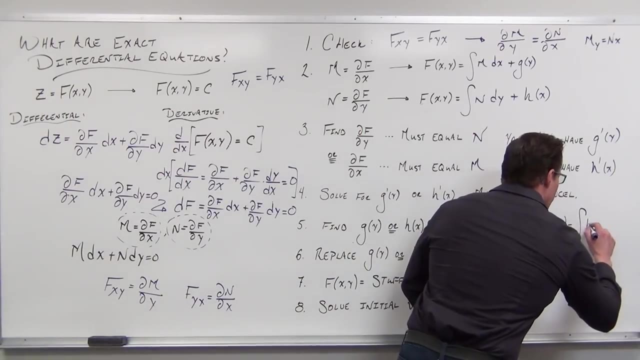 right, You have this equal. How do you undo that? Well, we do it in rules. So let's find g of y or h of x, g of y. let's do an integral of g. prime of y, dy, h of x. Let's do an integral of h. prime of x, dx. 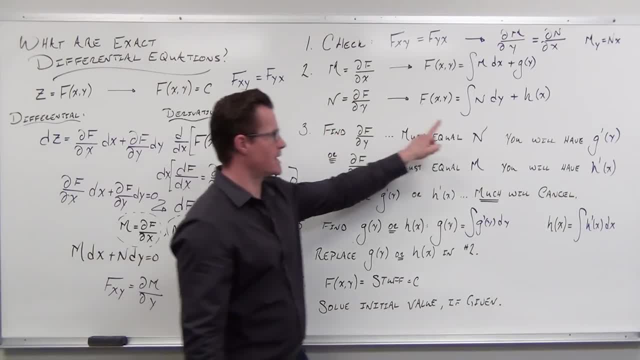 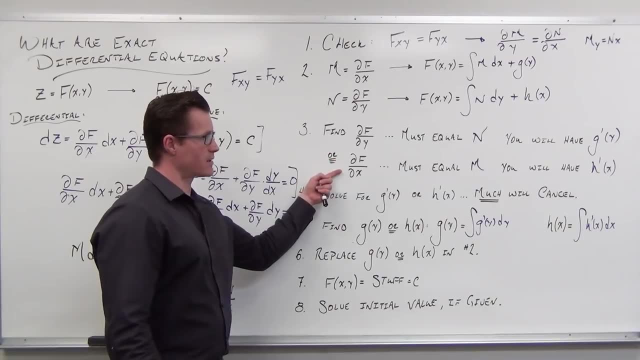 Shoot, that's how we got it anyway. We took a derivative with respect to y to get n, to get this thing All right, cool. And then we undo that with respect to y. Or we took a derivative of x to get to m, And then we undo that with respect to y, And then we undo that with respect to y. 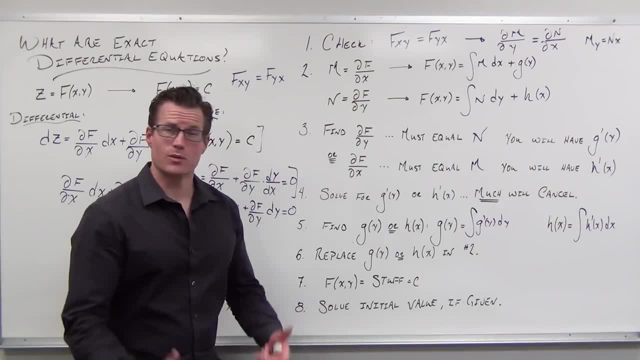 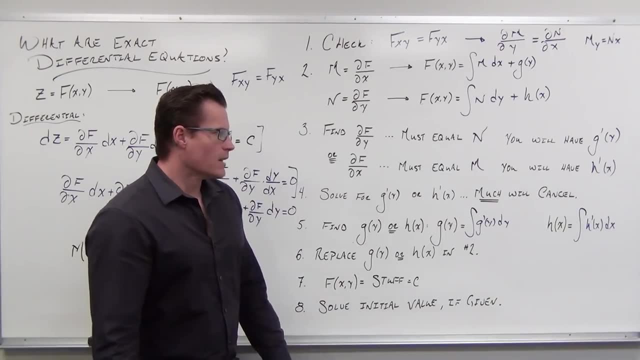 To get to this thing. So let's take an integral. with respect to x, Your variables have to match up. anyway. You're only going to have y's here, You only have x's here, So the dy and the dx should be making sense. Lastly, once you find this piece, man, I promised you earlier, I said: 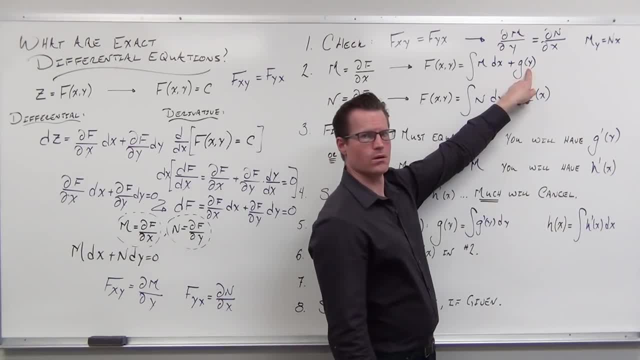 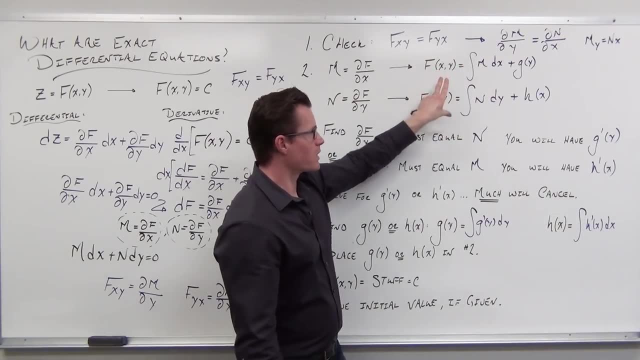 this is your function, right? It just has a piece you don't know. Likewise, this is your function: It has a piece you don't know. So, either way you go, you're going to get the same answer. Um, do one of these ways, And then the piece you don't know can solve for right. 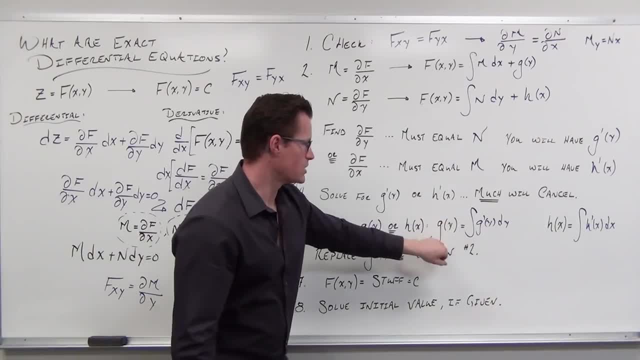 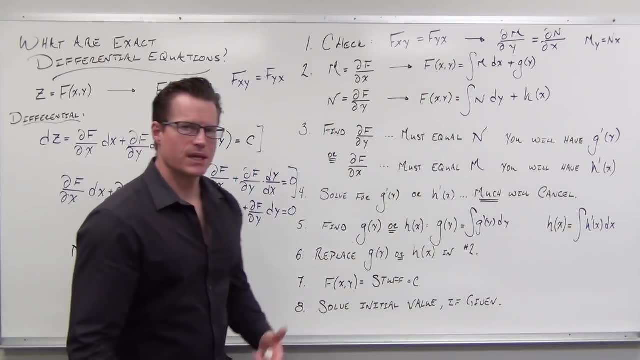 here. So let's replace it. Let's take these two things, this g of y or this h of x, and we replace it in our function here, And then you know what You're done, Because what we're trying to get is our potential function right there. And this does it, man, When you replace. 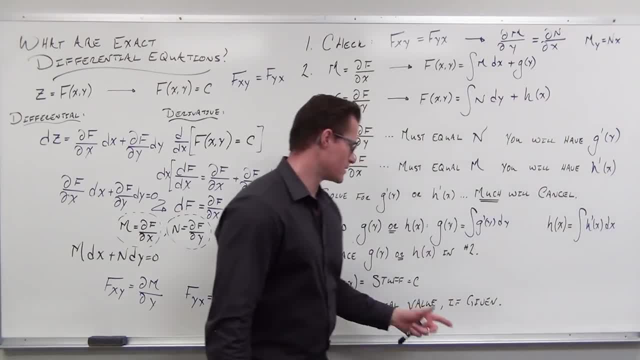 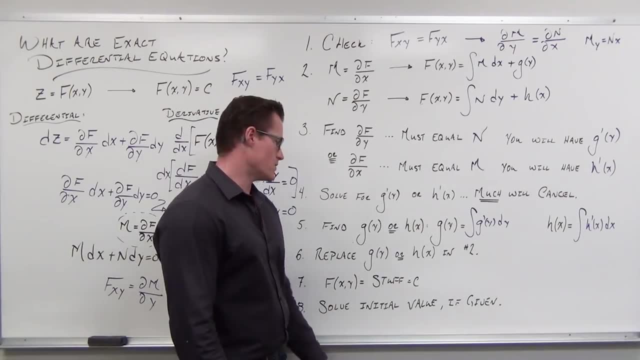 that. that is your function. Set it equal to some constant, some c, and you are. you're money, You're good to go. We're going to explore that in two examples. If you're given an initial value after this step is where you plug it in Um. so so keep in mind what we're doing, right. 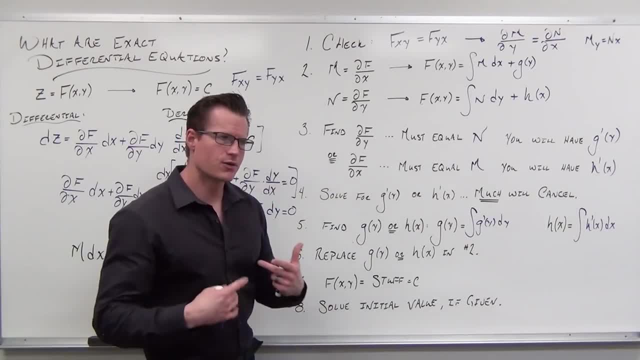 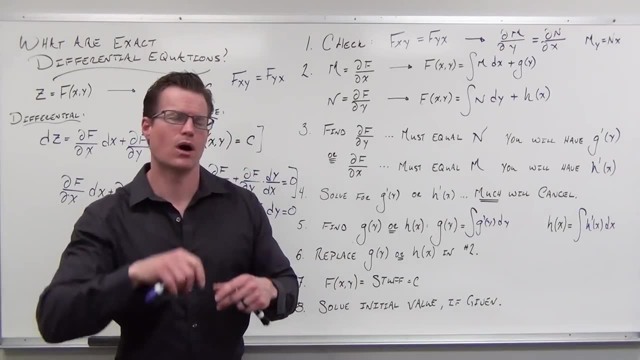 These are level curves, So they're they're curves And, like every differential equation, when we solve it it's giving us a family of those curves, like an infinite family. To figure out what specific curve you want, what particular solution instead of a general solution you need. 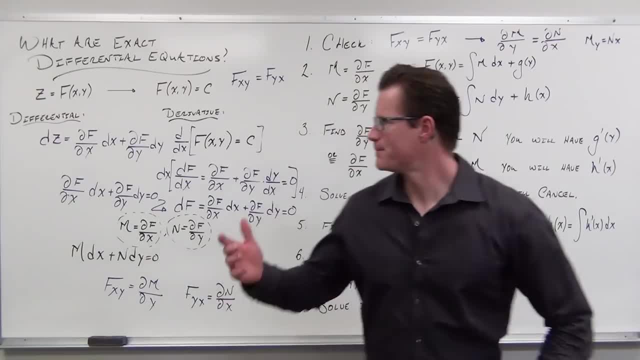 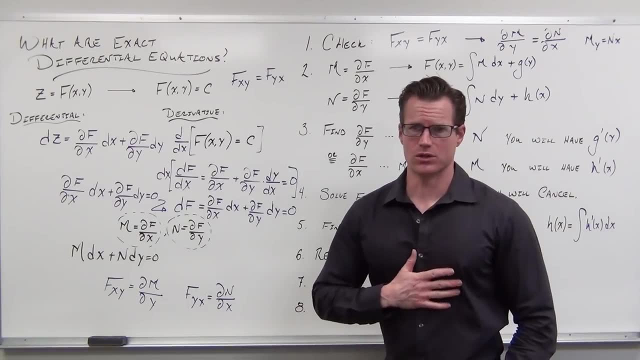 initial value. So I hope that makes sense to you. I hope the the logic behind where you're getting an exact differential equation is explained well enough for you guys to understand. That's always my goal: to make sure that this stuff makes sense. The process right now seems pretty vague because 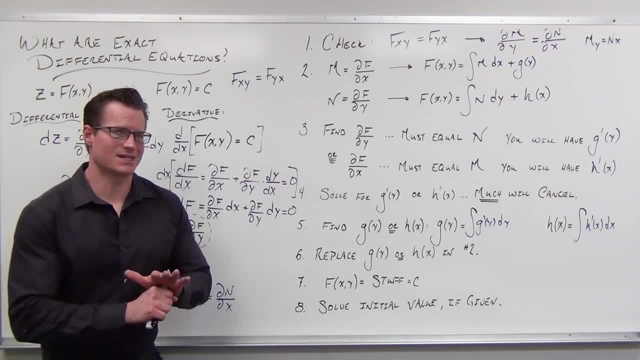 we don't have? um. well, it's not, but it seems pretty vague because we haven't done an example. Hang on for it. We have two examples. I will walk you through. We'll see how all this stuff works. 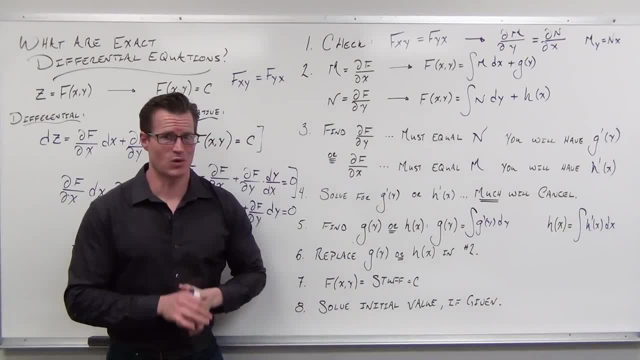 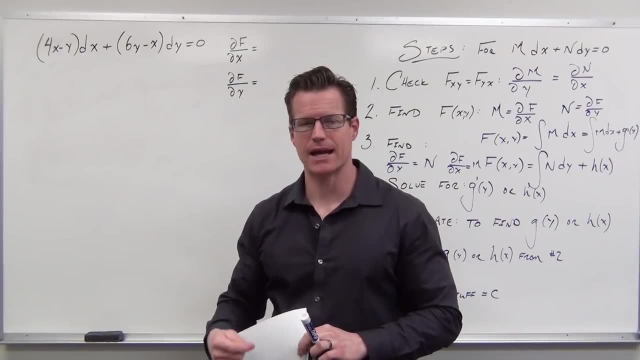 We'll make it a little more concise and then we'll go through it. Okay, Hang on, We'll be right back. Okay, I hope you're ready. We're going to go through, um, how to solve an exact differential equation. What, what it means. I'm going to show you how all these steps make sense. But now when? 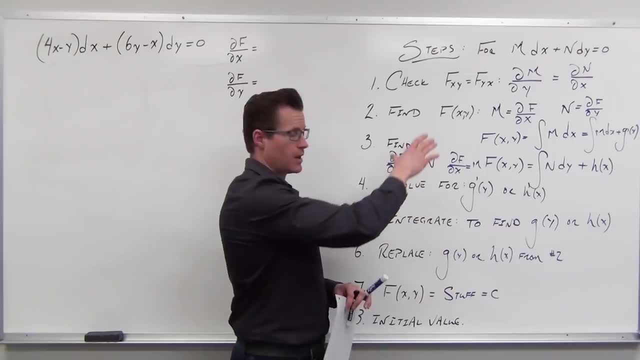 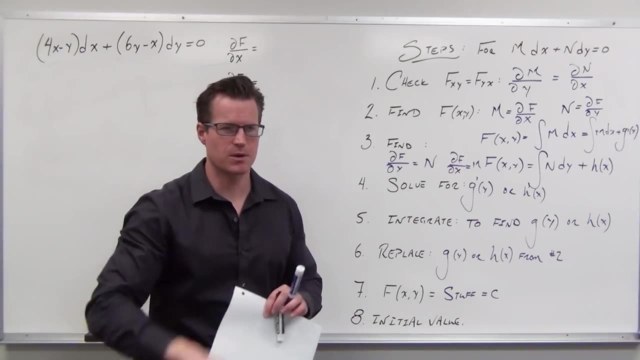 we go through it there, you're going to see where these come into play. So I know this was very, maybe, vague. It does fully explain it, but without doing example you're going to lose track. So stick with me on this one. Let's go through every little detail and make sure that we get it. So, number 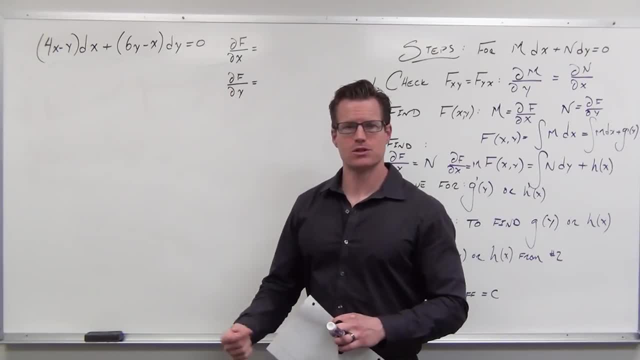 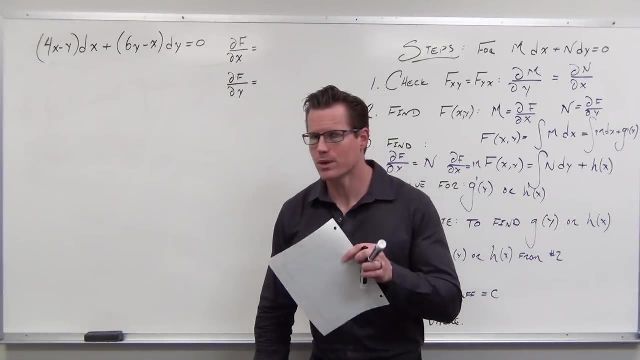 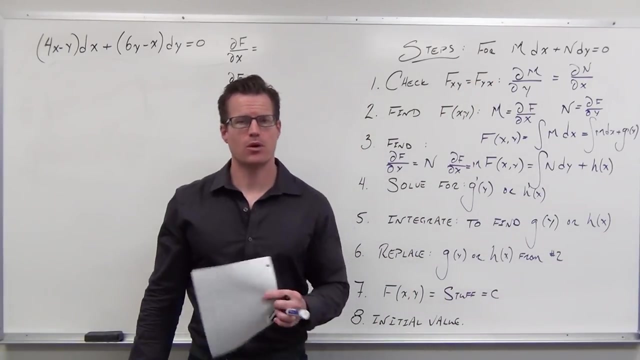 one. uh, what in the world is that? Well, that's an exact differential equation, written in what's called differential form. So we have a differential equation. Is it exact? Well, before we can say that, we need to do a test on it. So, for this, let's test the mixed partials. Let's see what happens Now. 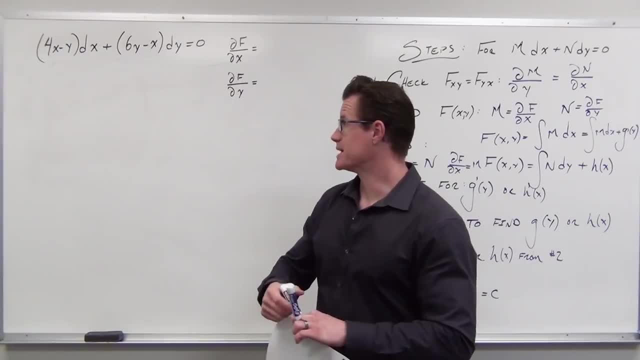 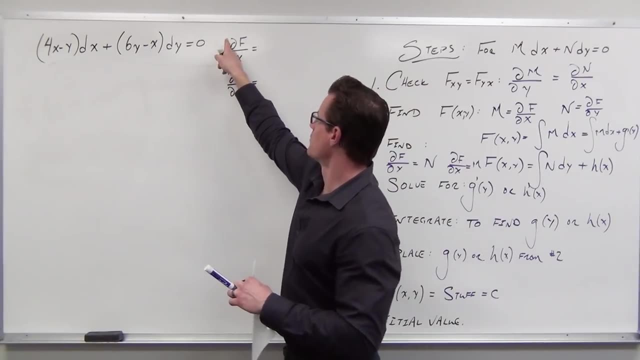 let's talk about the terminology here and what these little pieces mean. So, based on the form of our total differential or exact differential equation, our partial derivative of f with respect to x would be this piece, But this is written three different ways. The partial derivative of 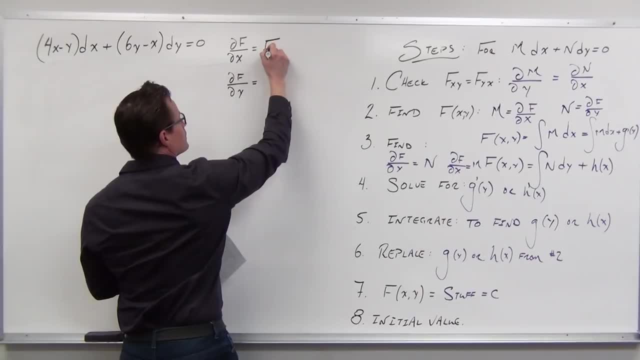 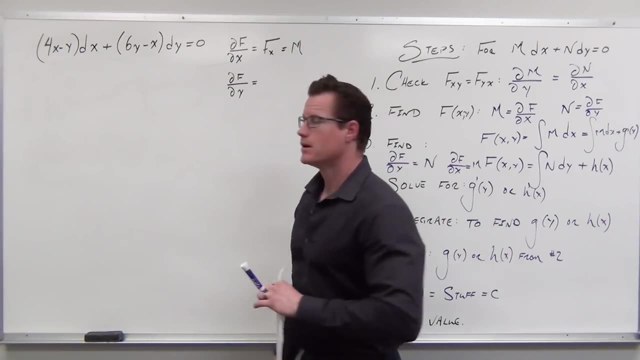 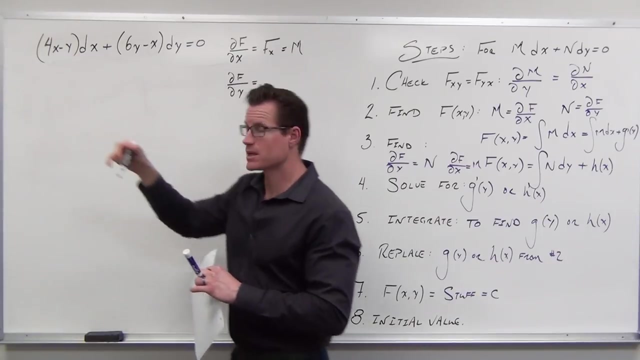 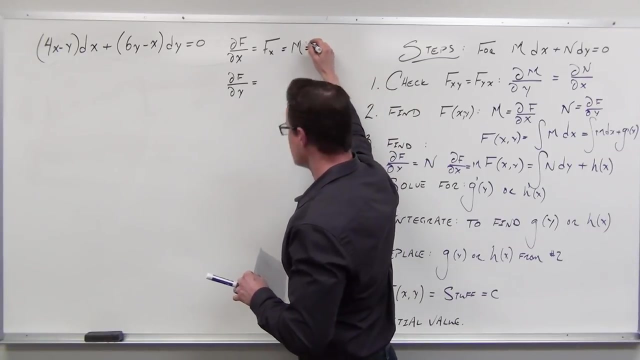 f with respect to x could be written as that Partial derivative f with respect to x, And that is our m. the piece the partial derivative of f with respect to x is the piece that's in front of your dx. So this in this case is just 4x minus y, Now the partial derivative of f. 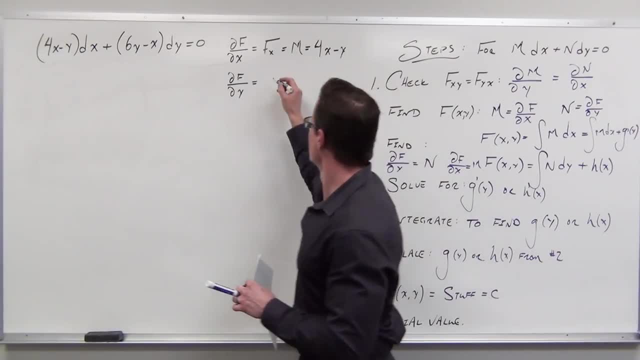 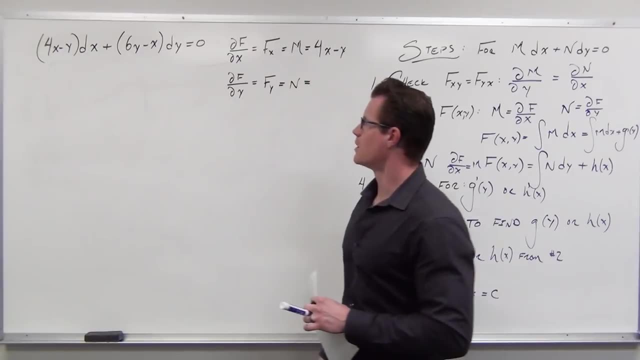 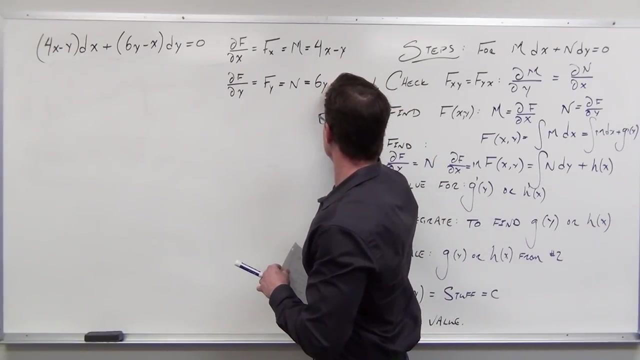 with respect to y, according to our differential form, or you could write it as partial f with respect to y, or you could write it as n. that's the most common is this piece. It's always the piece that's right in front of that dy. I need you to be. 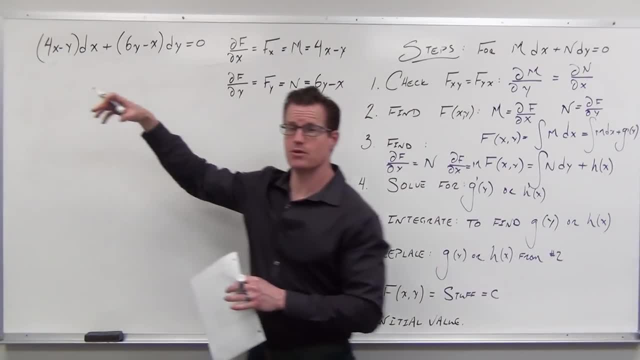 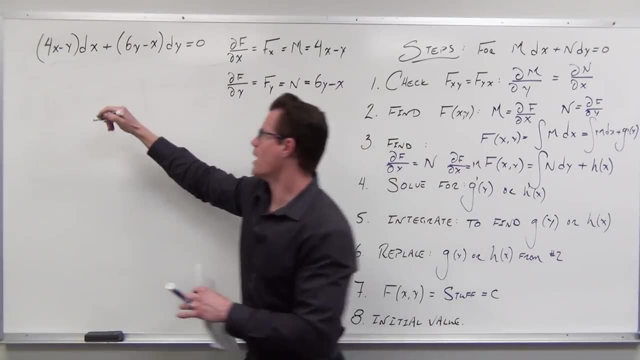 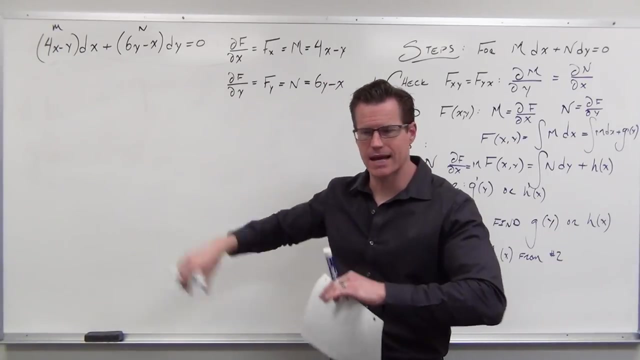 familiar with that. This n is in front of dx, this n is in front of dy. That means the partial of f with respect to x and with respect to y. Now we do our test. We see if this is actually an exact differential equation by doing what's. 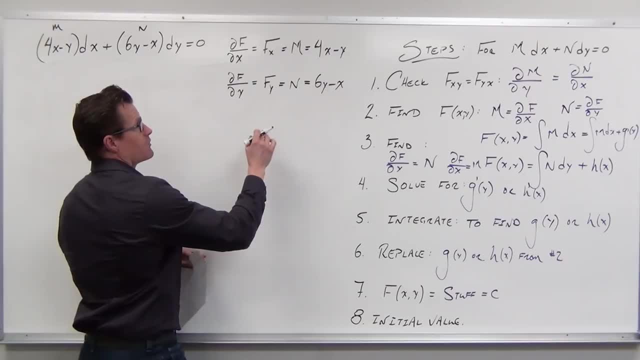 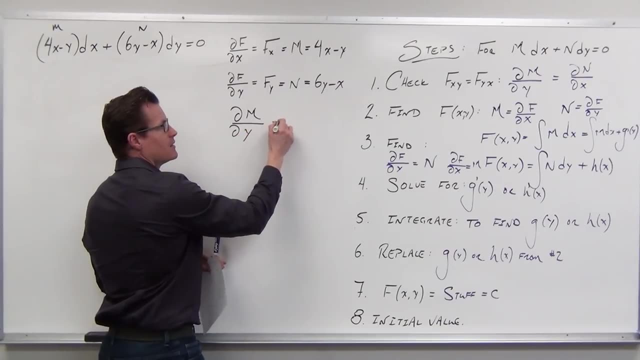 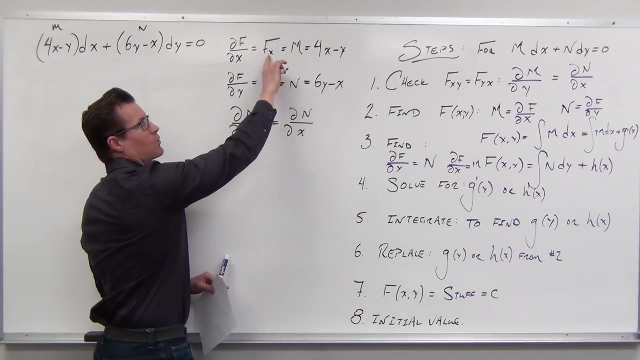 called a mixed partial. So we want to discover: is the partial derivative of m with respect to y the same thing as the partial of n with respect to x, Since this is already a partial derivative with respect to x according to our form, then we're just: 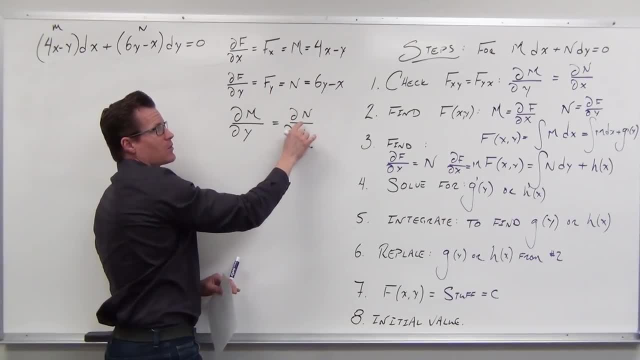 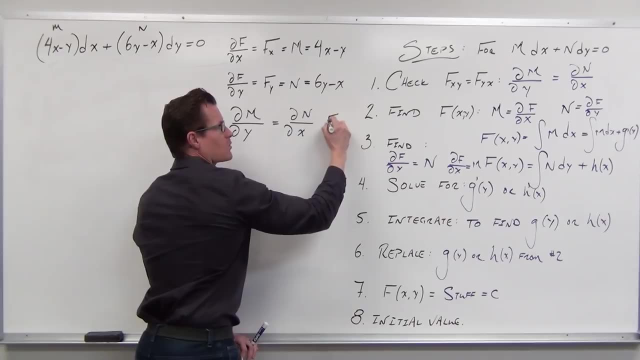 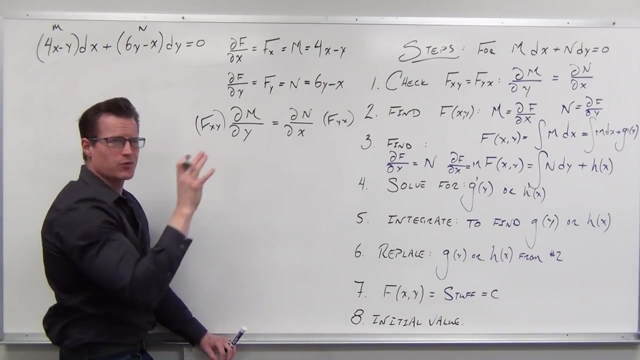 going to do it with y. Since this is already with respect to y, we're just going to do it with respect to x, and that gives us a mixed partial. This right here would be xy, This right here would be yx. Let's try it. So look back up here, hopefully. 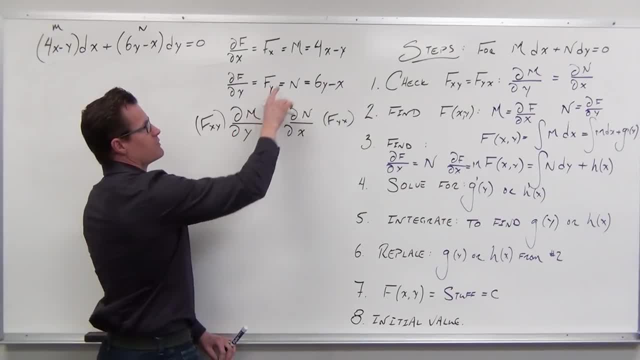 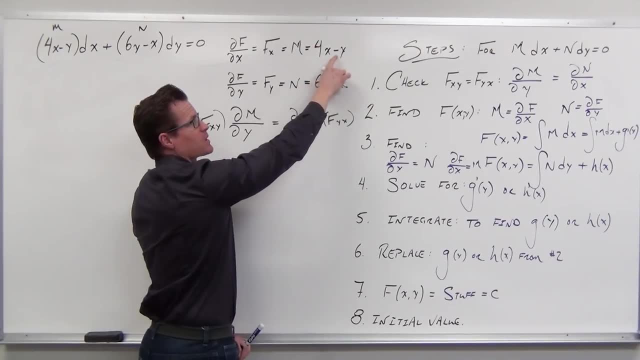 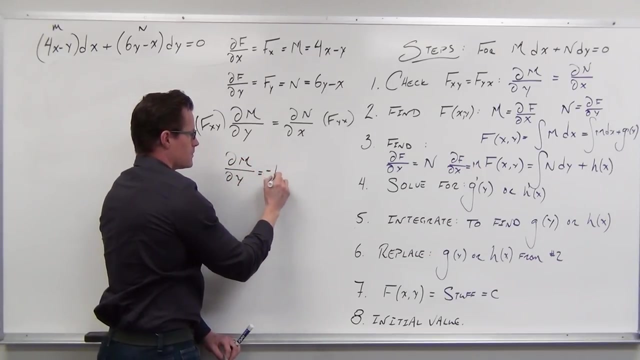 remember partial derivatives. We look at the partial derivative of m with respect to y and say: hey, with respect to y, that's a constant, that's 0.. With respect to y, this would give us negative 1.. Now let's look at the partial derivative of. 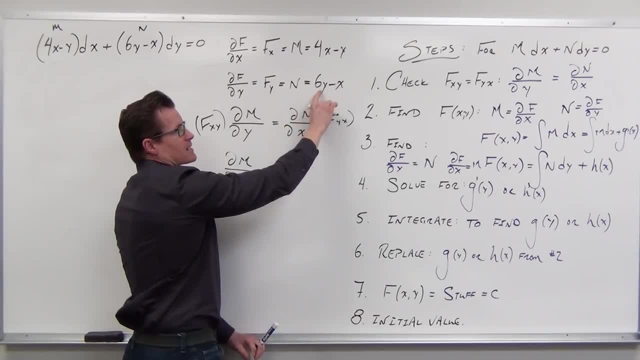 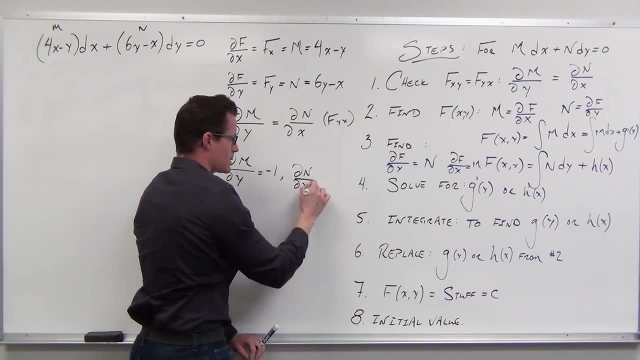 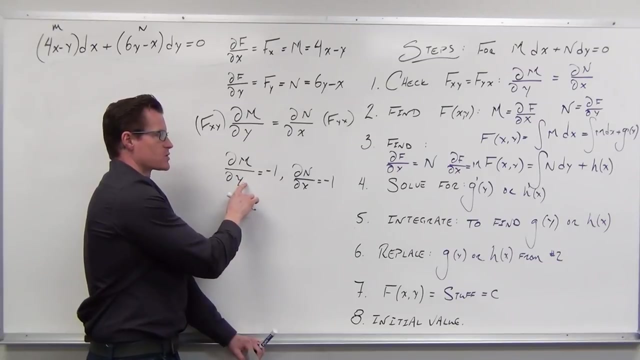 n with respect to x. Partial of n with respect to x. This is y. That would be 0 with respect to x minus 1.. Partial of n with respect to x is negative 1.. This is what we're looking for. We're looking for the partial derivative of m with respect to y and the partial derivative 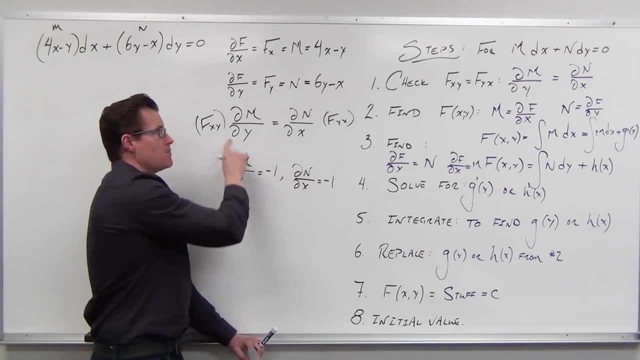 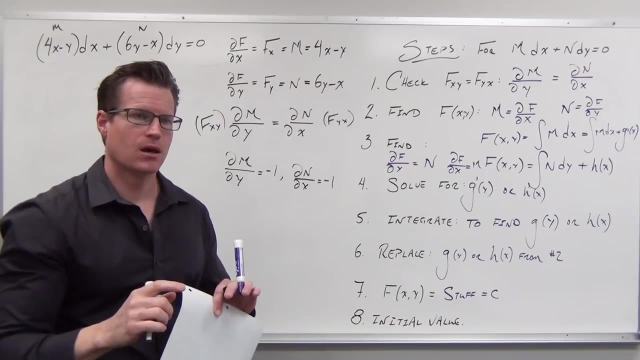 of m with respect to x to equal the same thing. What that says is: our mixed partials are equal. What that says is that if our mixed partials are equal, they're coming from some function where it is continuous and differentiable on a rectangle. 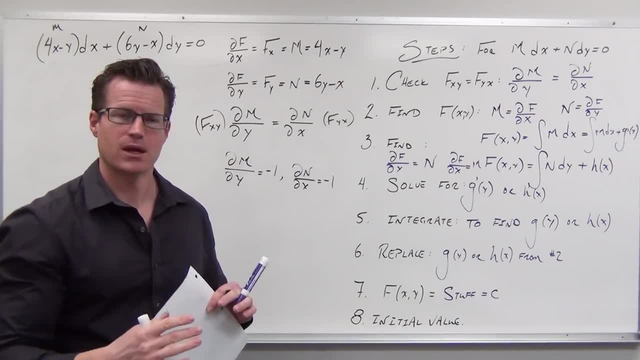 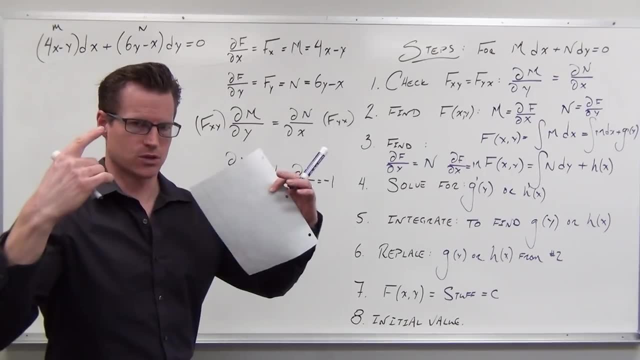 That's saying that we can work backwards and find a valid function on that interval. That's what we're doing here. We're saying, hey, this is now guaranteed an exact differential for some higher parent function. We're going to find that now. So how do we do it? So we've 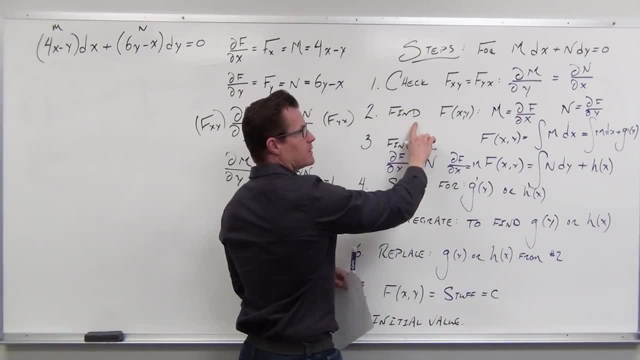 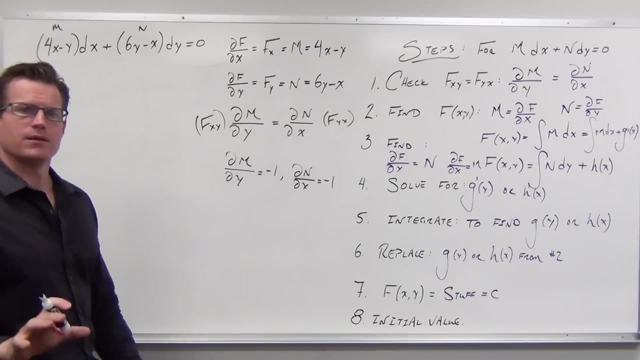 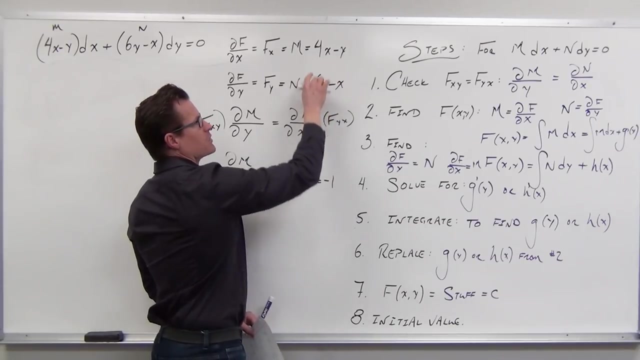 done, checked them. Good, Now we find f of xy. based on that, How does that work? This is where your textbook is going to kind of push you to this, and we're going to do that this time. But I want you to look at this. We're going to look here and see which. 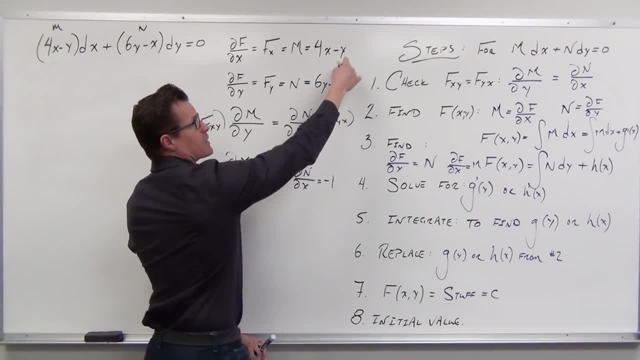 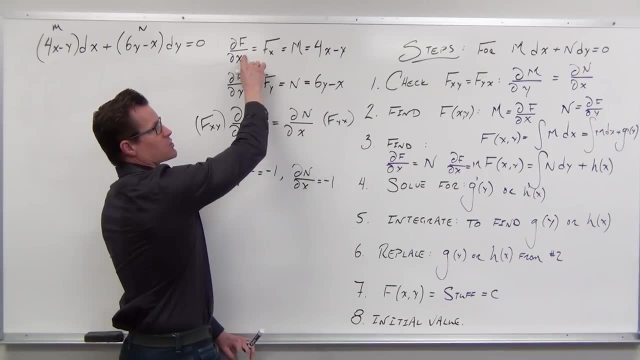 one is easier to integrate. Is it easier to integrate this with respect to x or this with respect to y? Now, why those two variables? This is already a partial derivative with respect to x, so we're going to try to undo that This is a partial derivative with respect to y. 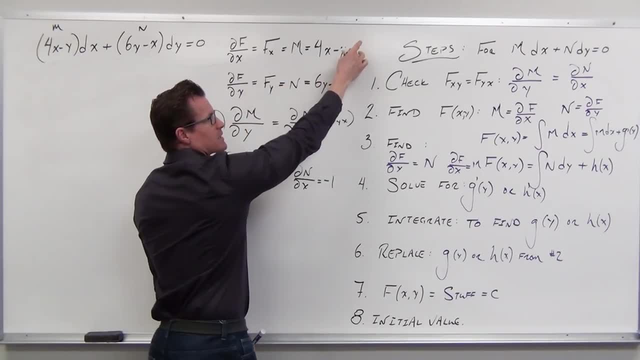 so we're going to try to undo that one. Which one's easier? this with respect to x, this with respect to y, or does it matter? In this case, it looks like they're about the same. So I pick this one because I'm 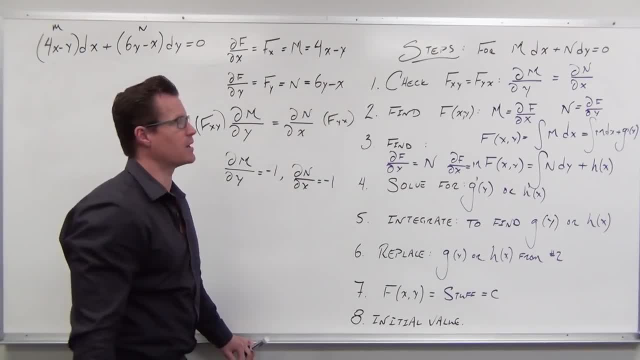 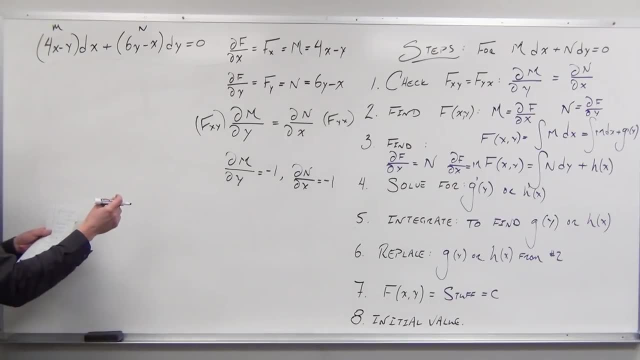 more familiar with integrating with respect to x, because you don't have to do it that way. So let's try it. Let's say: hey, well, you know what? if man, if m is the partial derivative of f with respect to x, which it is, and that equals 4x minus y. 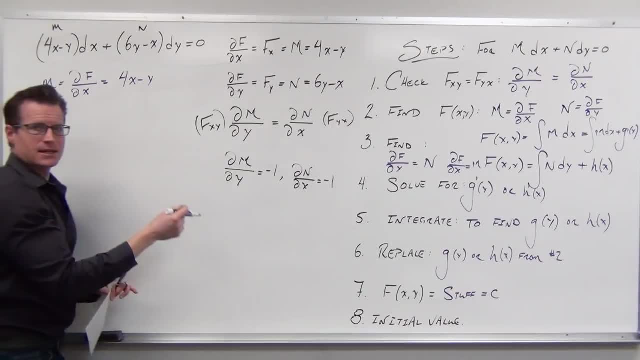 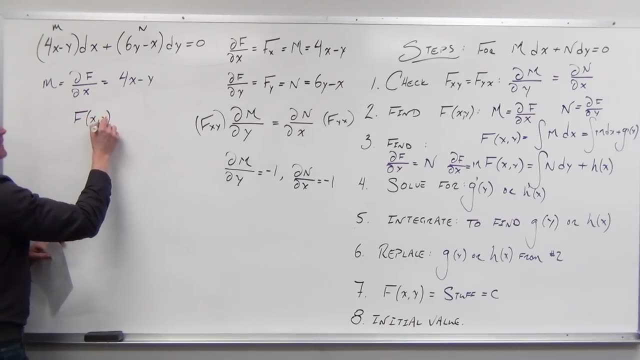 then check it out from here: If I take an integral of both sides with respect to x, then I would get: f of xy is equal to the integral of 4x minus y with respect to x. I'm basically doing this. We're basically saying, hey, take an integral with respect to x, take an integral with 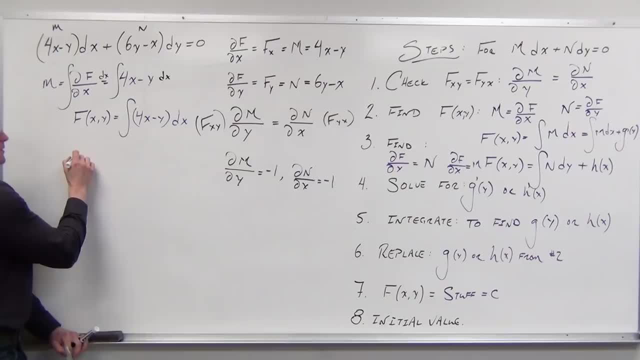 respect to x. That's basically what we're doing And we're saying: well then, this is really nice. The integral of 4x would be: let's see 4x squared over 2.. So x squared over 2, the 2. 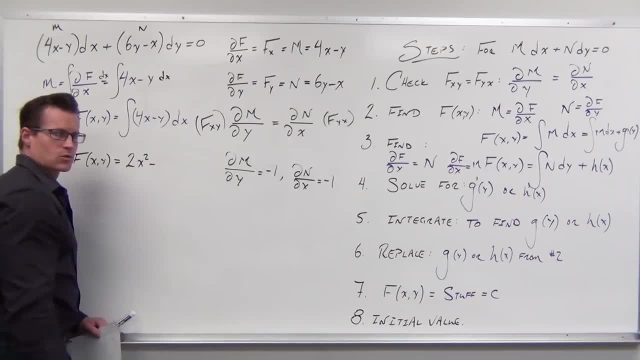 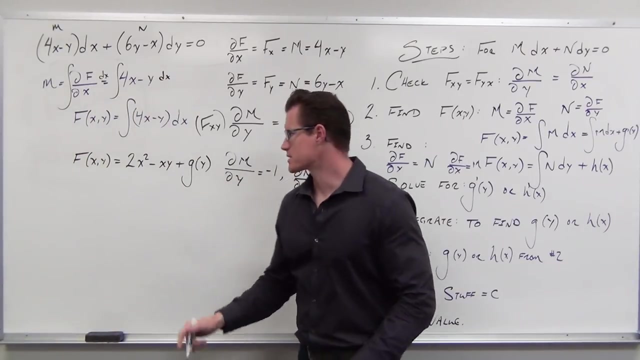 would cancel 2x squared minus integrals of things that are being held constant. So, like y, we would get this xy. But we also get- this is very important- we also get some function of y, Because if I were to take a partial derivative, let's just verify this- if I were to take 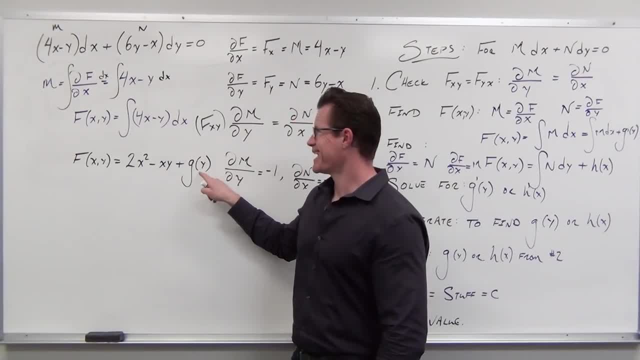 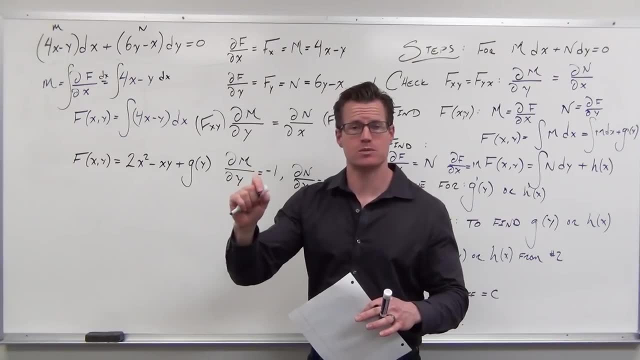 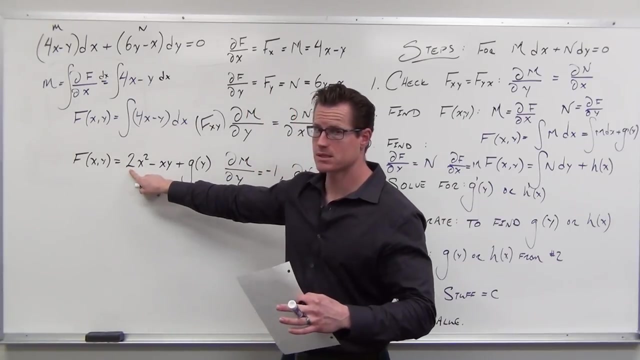 a partial derivative of this thing with respect to x. it darn well better equal m, Because that's what m means. m means a partial derivative of f with respect to x. Let's take a partial derivative of f with respect to x and make sure that happens Here. those are all x's. 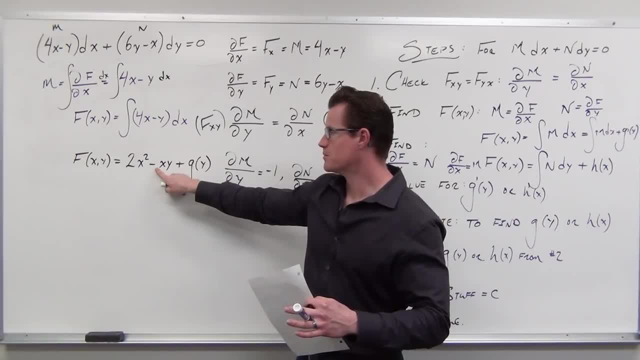 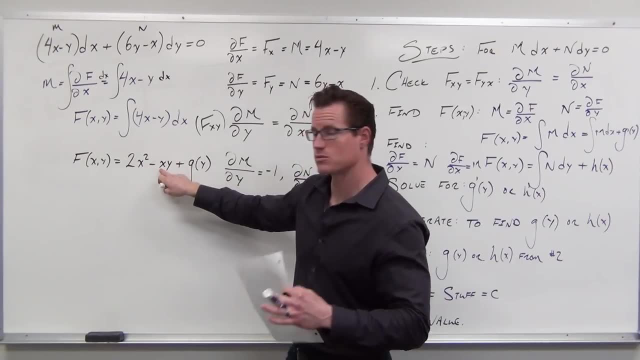 that'd be 4x. Here I take the derivative of x, but y would be held constant. that would be minus x. So this would be 4x minus x And I'm going to take a partial derivative of x. I'm sorry, 4x minus y. The derivative of x would be 1, we leave the y alone as a constant. 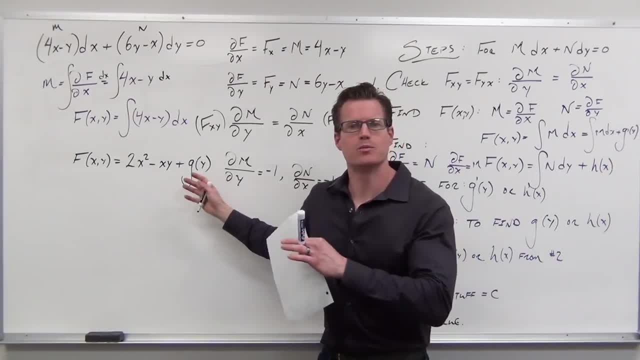 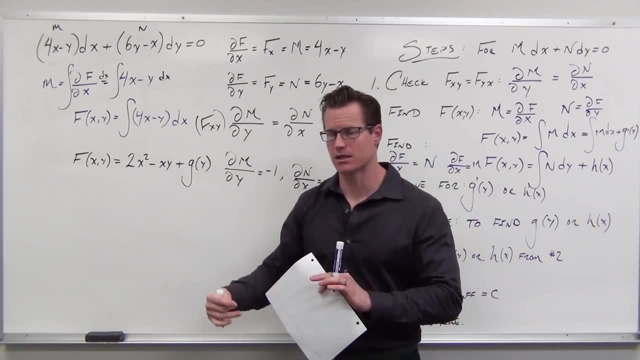 4x minus y is here. Why about that? That would be all in y's. So all of these terms over here that are added, all these terms would go to 0 on a partial derivative with respect to x Man. I hope that makes sense. That's where a lot of students lose it and go. what? 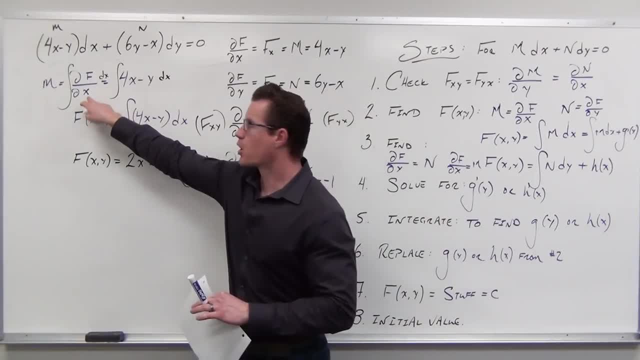 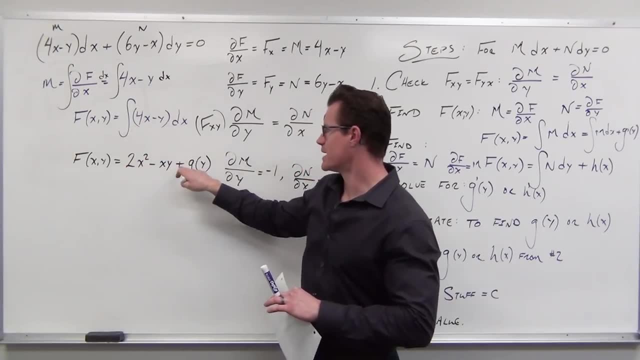 about that one. Why is that there? Because if this is a partial, that's a partial. then when I do an integral of both sides, I do it with respect to x, So I get x squared over x, So I get this, but it has some function of y because that integral, that partial derivative, 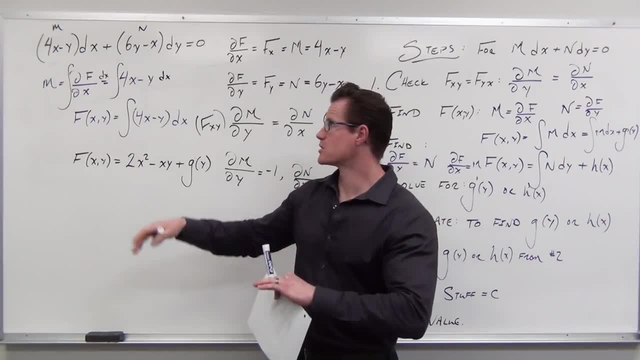 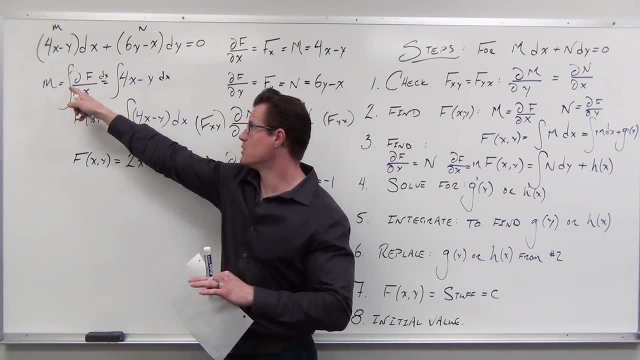 says, all those y's would go to 0.. Are you with me? So we've checked it, we know it's exact. we've labeled it, we've picked something. we're going to integrate either m or n. m you integrate with respect to x because it is based on a partial of x. We do that, we. 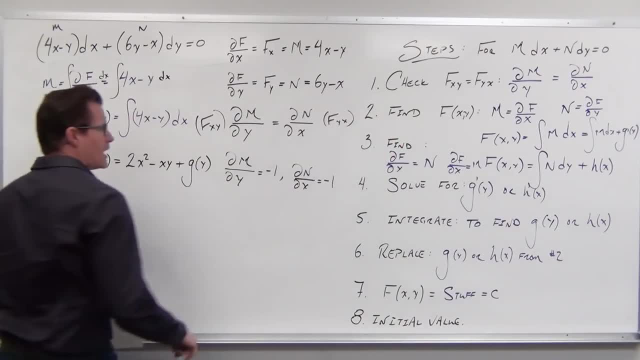 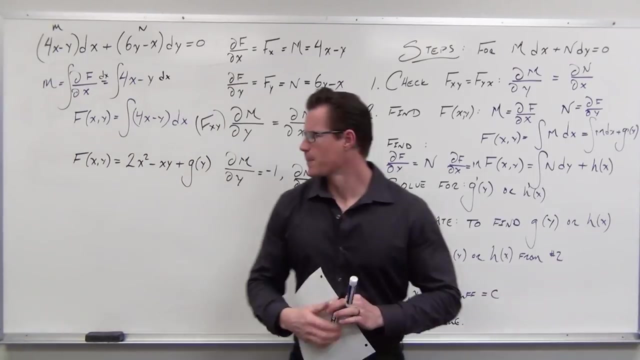 have a function of y considering a partial derivative. But now, so we're right here, we found one of these Two things. Now, what we're going to do is we're going to take a derivative and we're going to say: what's the point of doing this? Why would we take a derivative? Well, if you 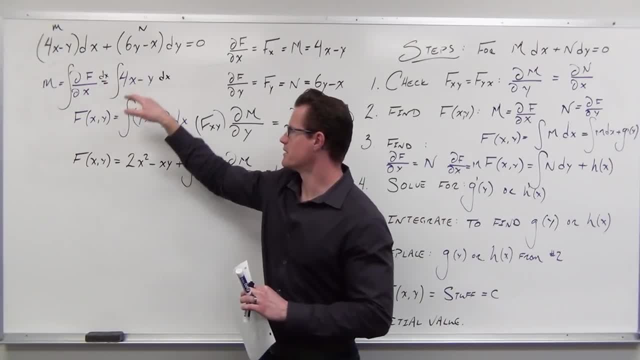 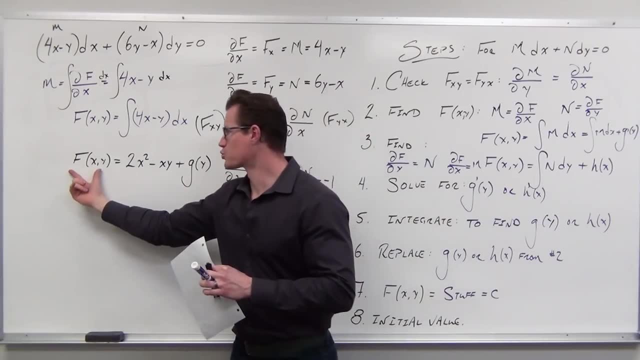 base this on m, and you said this is with respect to x. I did an integral with respect to x. I have this thing with a function of y, then let's be smart about it. What we have now is something that's really close to our final answer, this f of x, but we don't know. 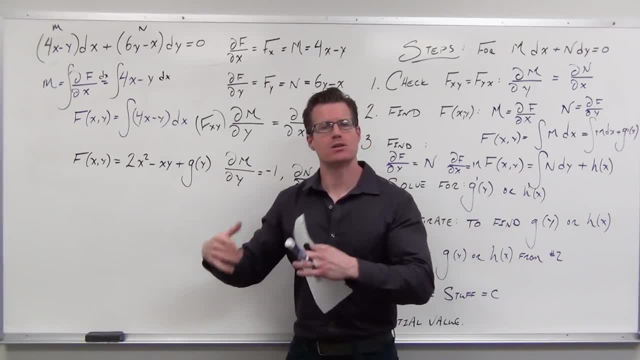 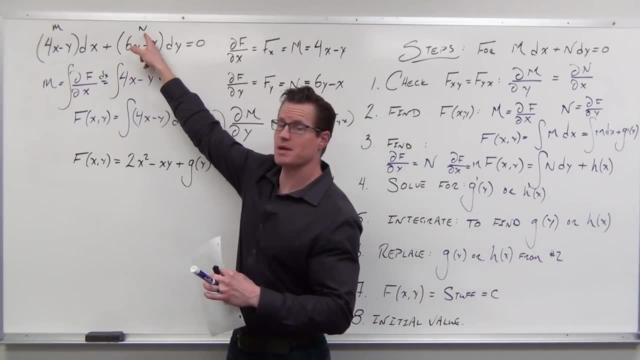 that piece. We don't know what g of y is. Now is the process for finding that Well, but we know something about this. We know that the partial derivative of f with respect to y, the partial derivative of f with respect to y, is exactly 6y minus x. So 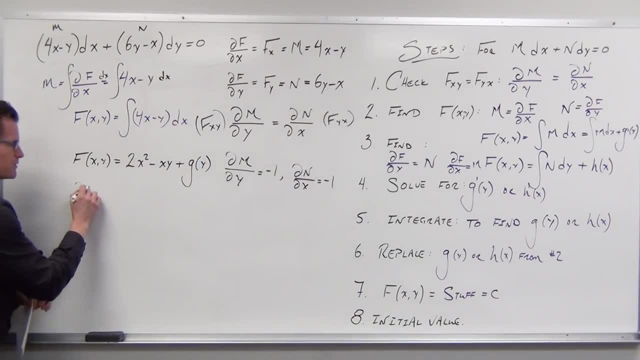 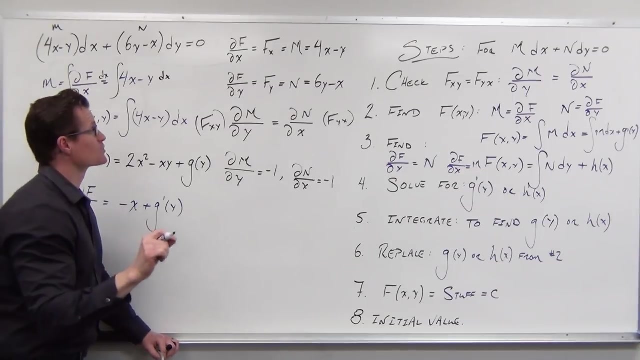 what if we were to take the partial derivative of f with respect to y? This would go to 0.. This would go to minus x. This would go to the derivative of g with respect to y. And this is really important right here. 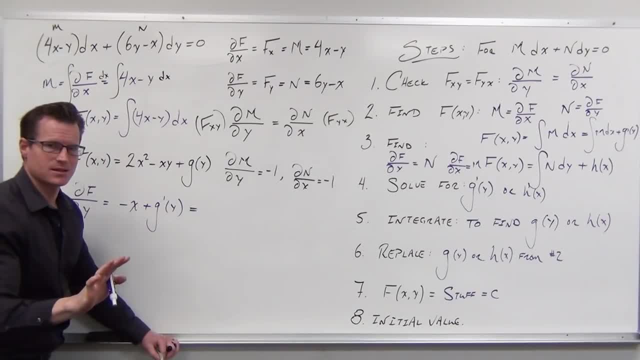 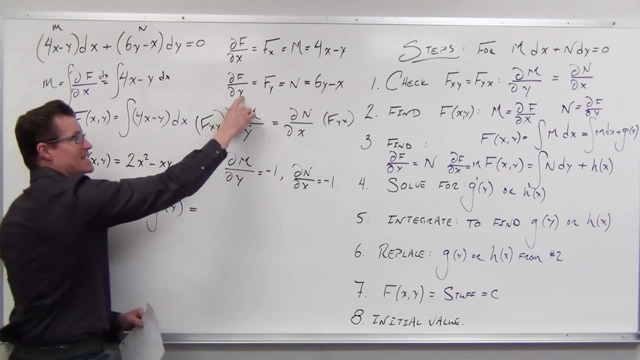 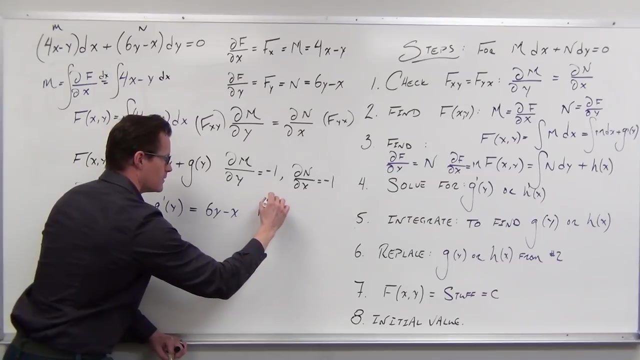 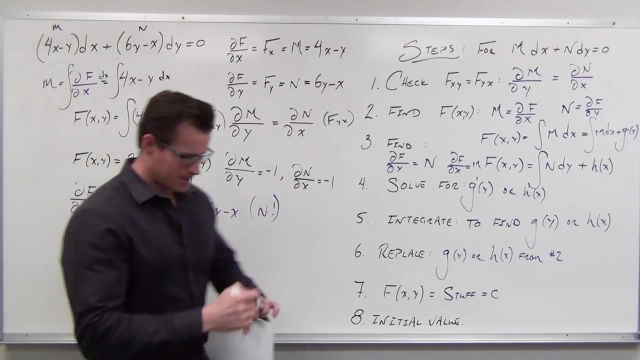 Understand this. Please get this. This is exactly what n is. The partial derivative of f with respect to y is exactly n. It's n, not n factorial. I'm just being n, It is n. You have to get that One last time. I want to let you know because it's getting exciting. 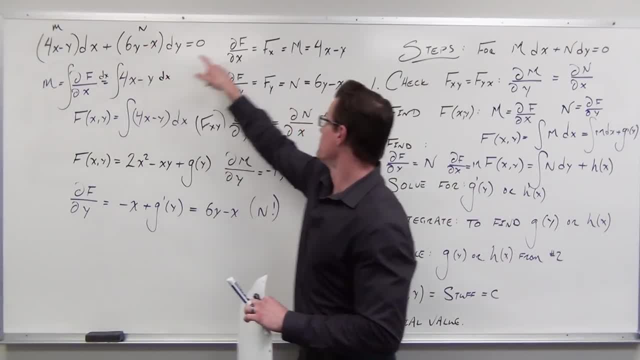 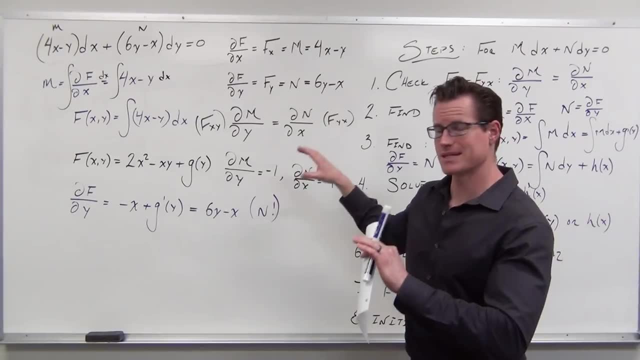 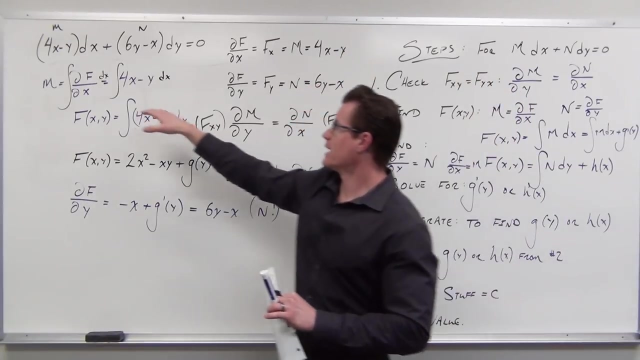 now, Is that an exact differential equation? Yep, Because we checked the mixed partials and that says that that comes from some parent function that's continuous and differentiable on an interval. this has to be an exact differential equation for one of those things. How do we do it? Pick either one, m or n, and just integrate. 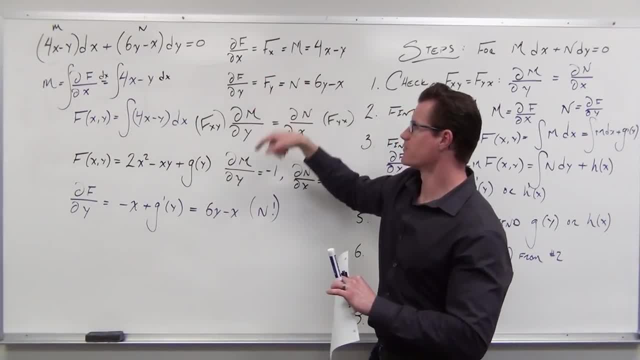 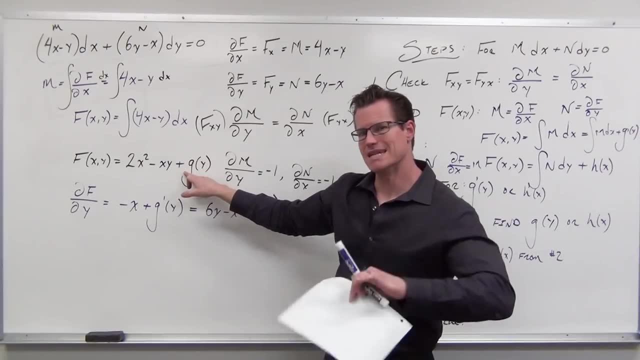 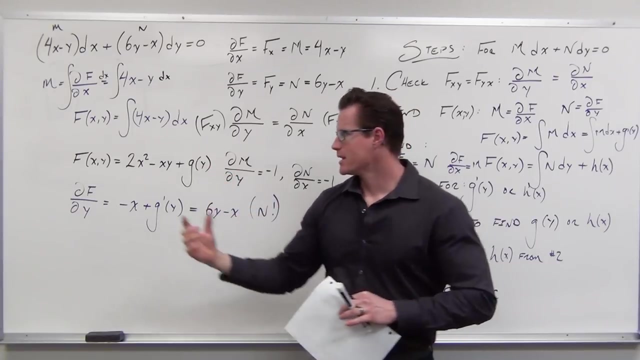 with respect to x for m or y for n. Great, You're going to get something very easy to find typically And you get some function of the variable that you didn't integrate with respect to. So for dx, you're getting a y. Then be smart about it. If this is the function that we're 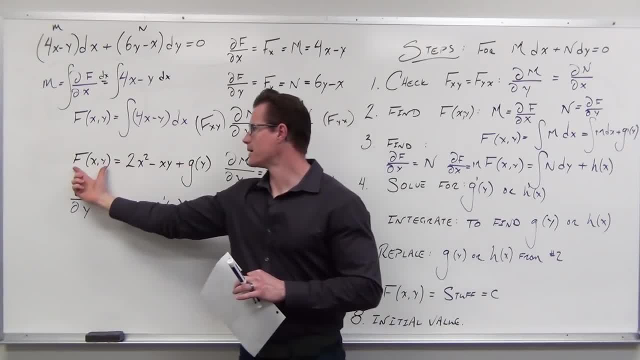 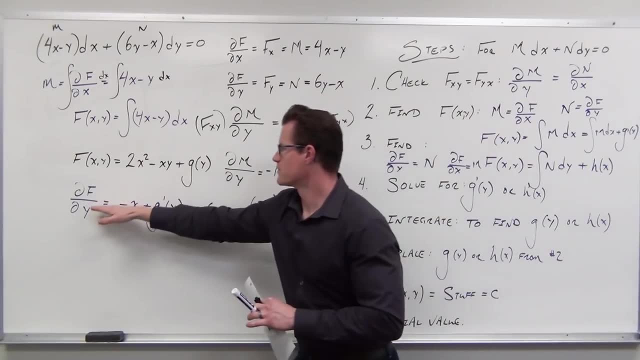 looking for. but I don't know this function of y. let's take a derivative with respect to y. Why? Because we know that piece too. So take the derivative with respect to y. So the other thing, the variable you didn't integrate with respect, to take that derivative. 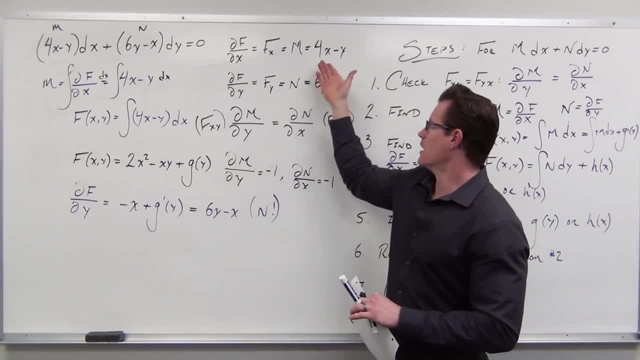 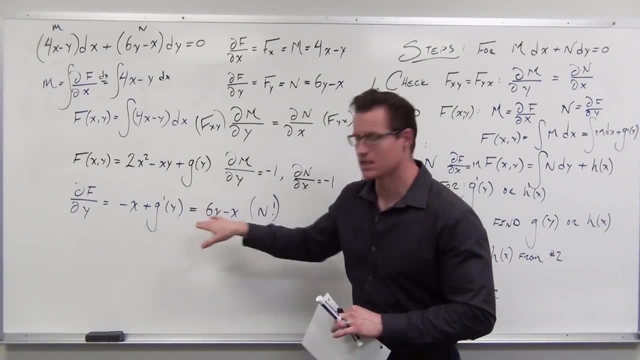 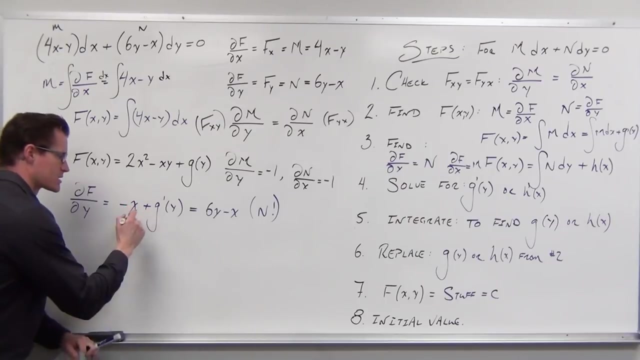 and set it equal to the other piece. So basically, integrate m, take a derivative, set it equal to n. The key is: don't forget about that. all right, Now lots of things are going to cancel. typically, So, like here, you add x to both sides and we get g. prime of y equals 6y. 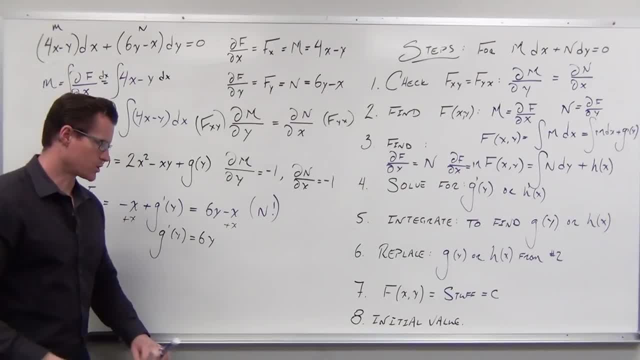 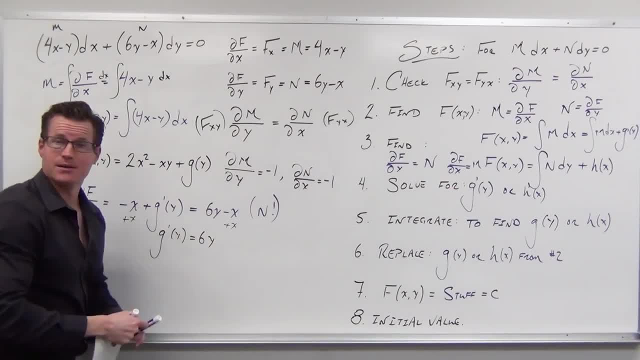 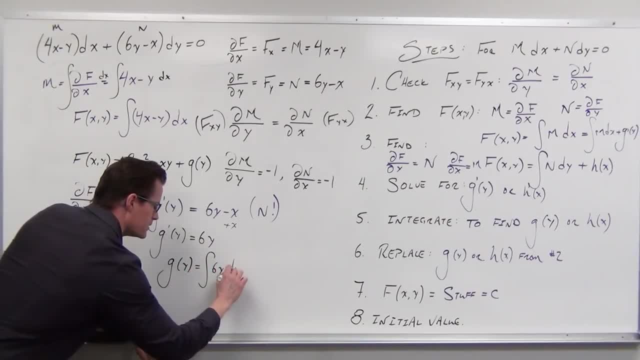 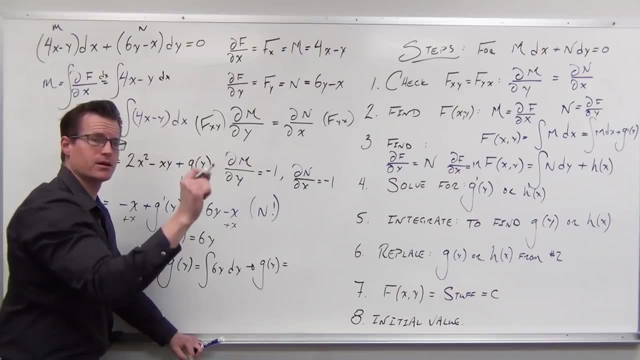 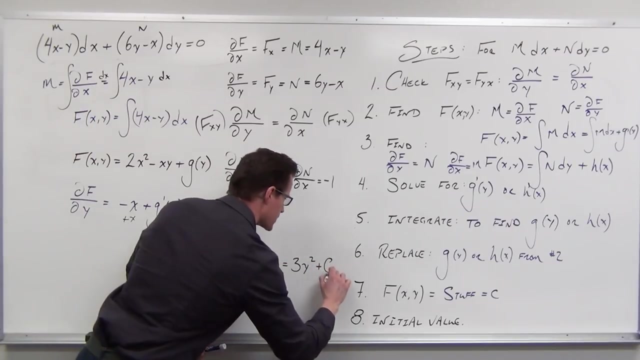 equals the integral of 6y dy, So g of y would equal. let's see, so it's 3y squared plus some sort of a constant. Now do we need the constant? Not really. I'll show you why, so I'm going to put a little c sub 1.. 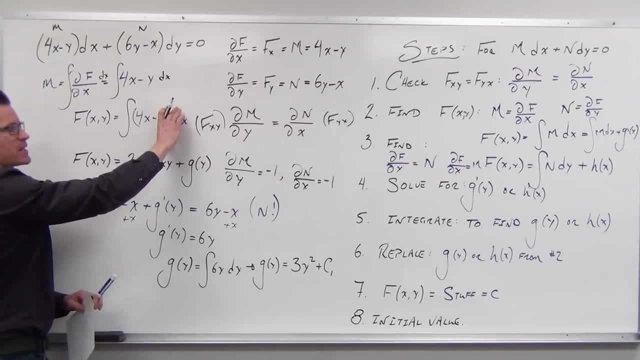 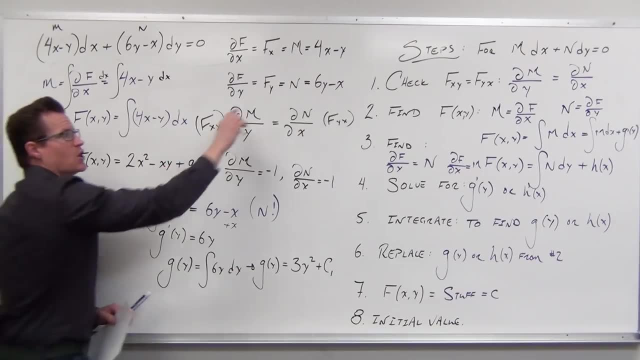 But here it is. We took our m, we integrated with respect to x, getting some function of y we didn't know. We took a partial derivative with respect to y, because we know what that's supposed to be. What that does is that allows us to solve for the missing, the derivative of the missing function. 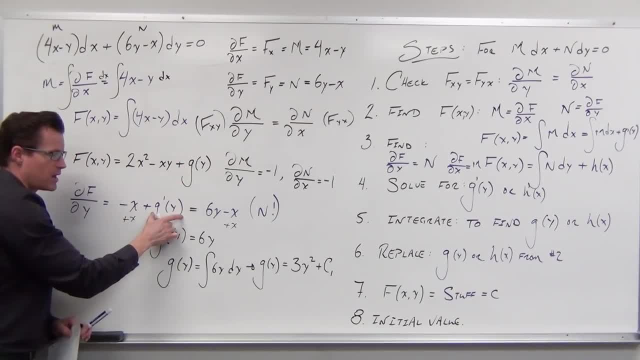 of y that we got. So notice, take a derivative of this, you get g prime y. Solve for that. How do we solve? how do we undo derivatives? Well, we take integrals. and you've just found the missing piece. 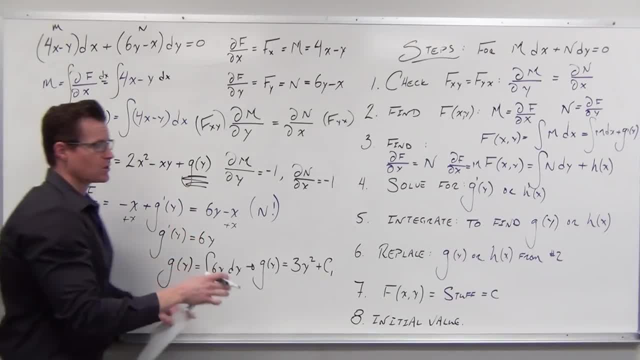 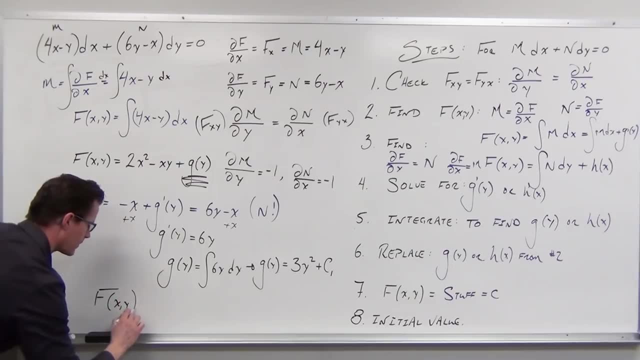 that's right here. You just found that, So replace that from step number two. Replace it from right here. So our function is now: this is great, We got that from integrating our x's. This is great, We got the same thing. 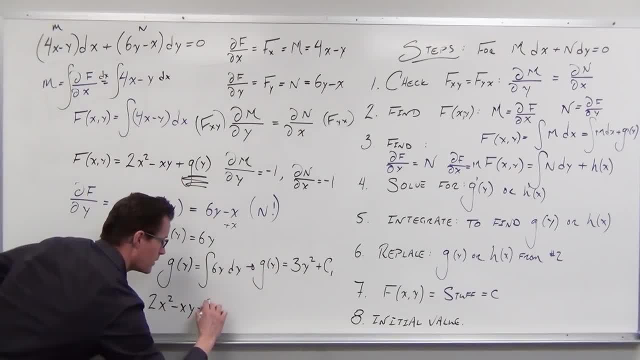 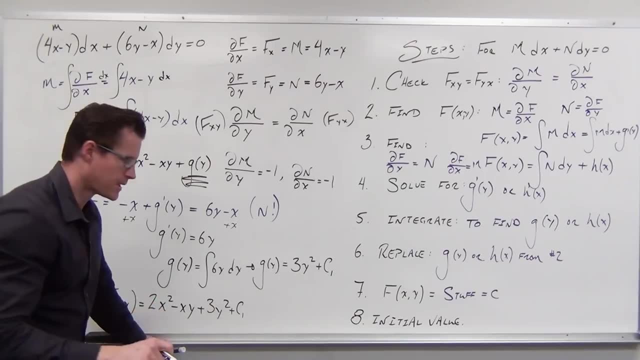 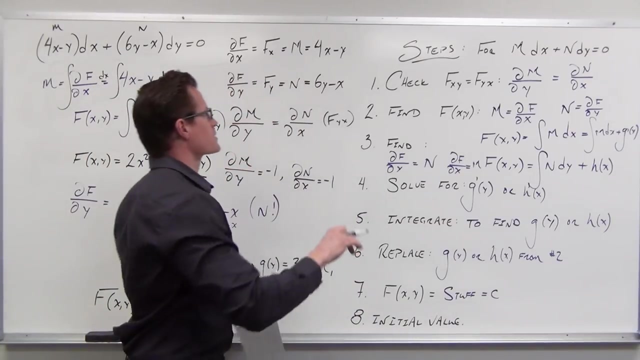 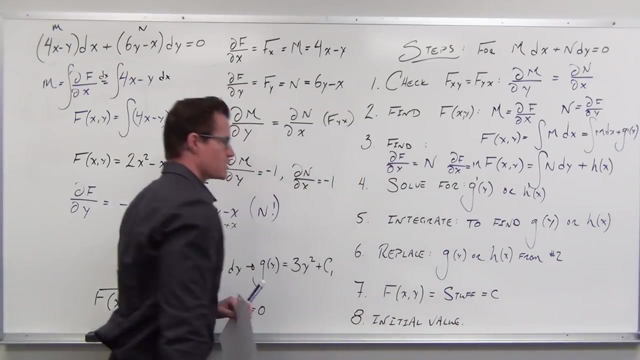 But now we know this. This is 3y squared plus c sub 1.. But here's the thing, Here's why this constant does not matter. We know that this is. this was an exact differential equation for something that's of this form. I erased it. That's something of this form right here, So something in. 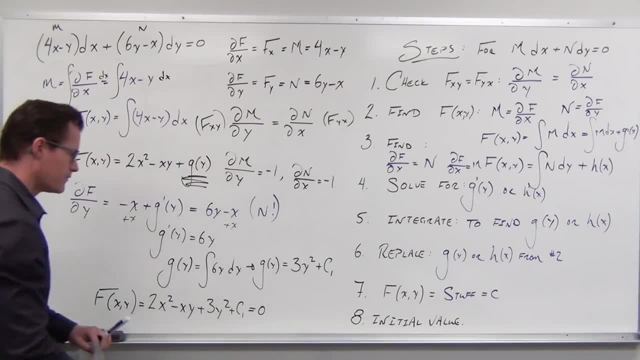 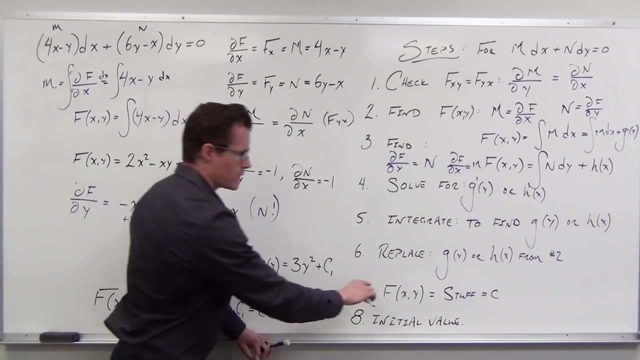 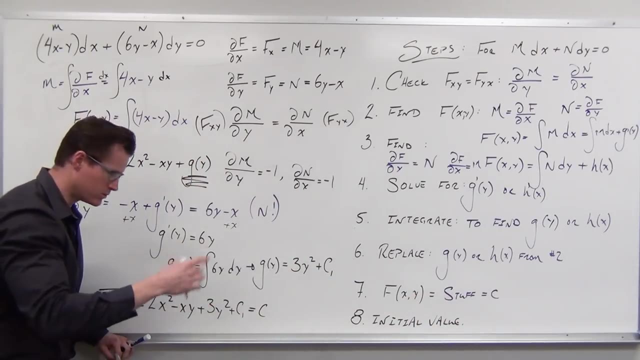 the form f of x- y equals c. Well, if this is sorry, not zero- f of x, y equals c. So we have solved it. We now know the function. We have all of our stuff, all of our complete function. There's no g of y, no h of x, But we know that. 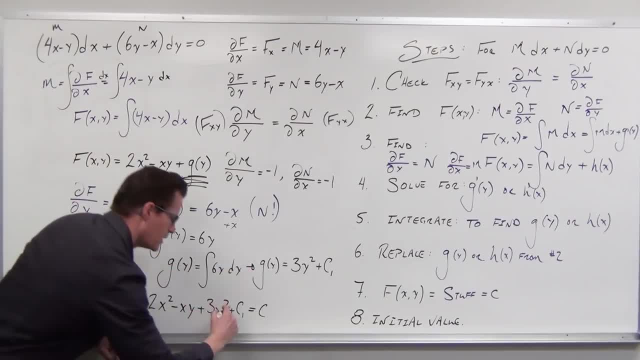 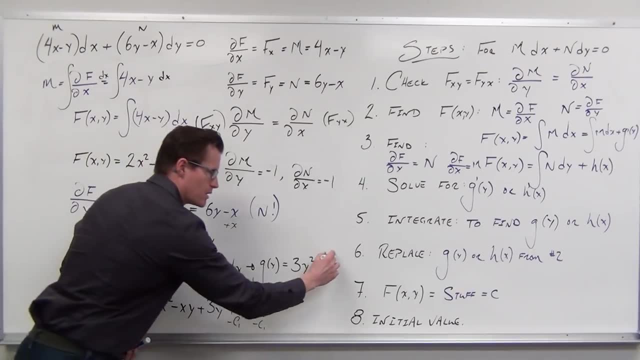 this comes from some function of x's and y's equal to a constant. Notice how we can just subtract this constant and you would get just another arbitrary constant. So typically people don't even have to show that You don't even need it because you're going to wrap it up in the 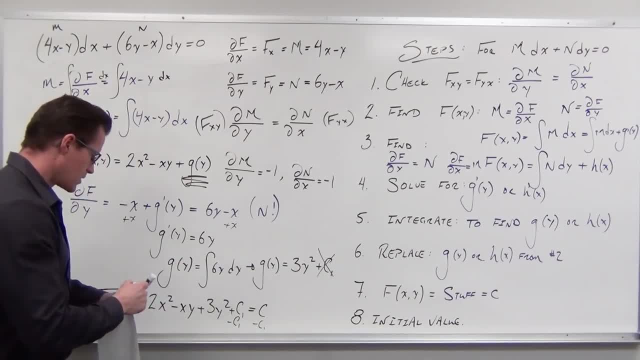 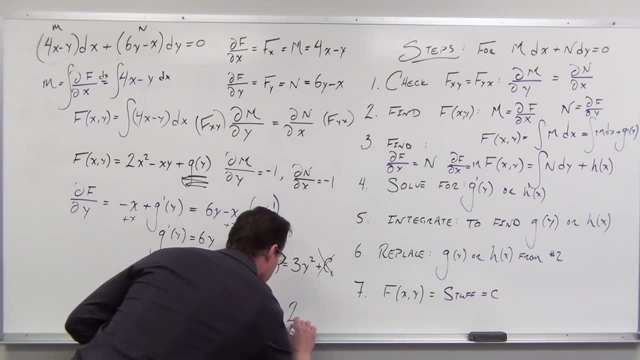 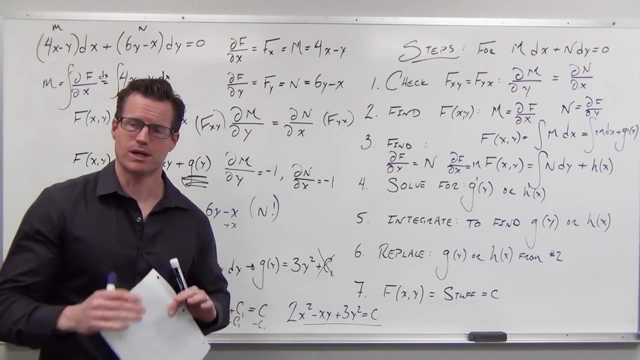 constant Either way. So for us, our final solution would say that is a function in terms of x and y equal to some constant. Exactly what we're looking for. Exactly something that's producing level curves. for us, That is rad, Like that's. that's what we want. 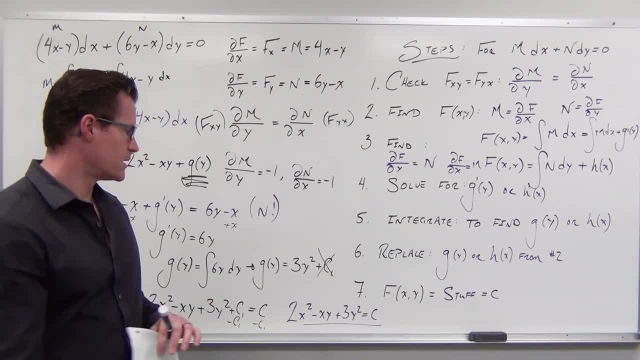 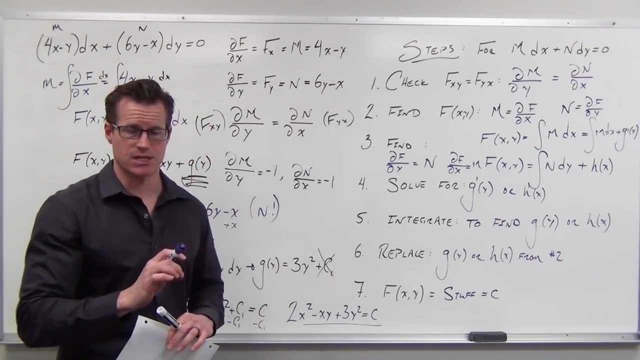 Now, if you had an initial value problem, say y of zero equals one or something- you could plug in the zero for the x, the one for the y and you could actually solve for c. That would give you a specific curve going through a specific point. That would give you a specific differential. 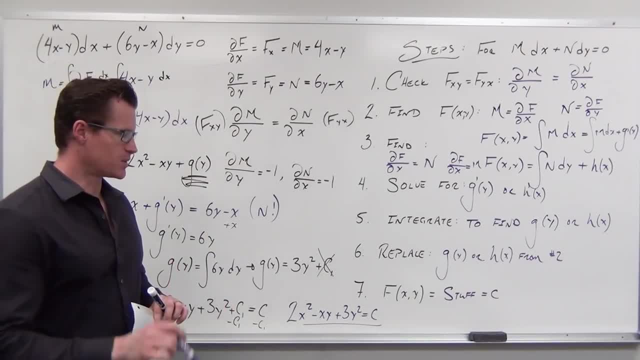 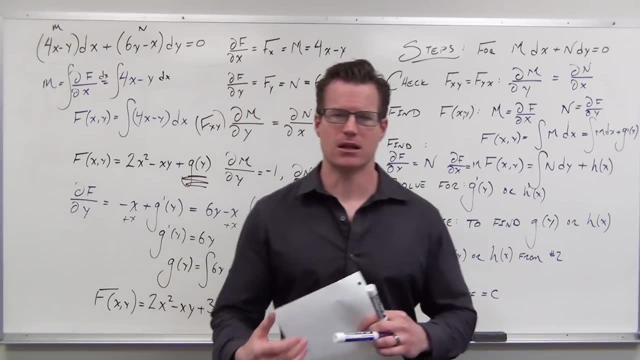 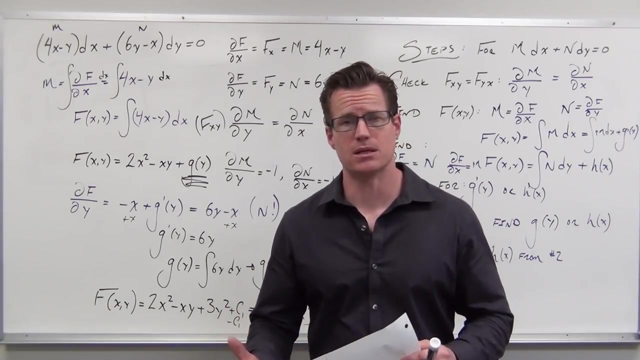 equation, Sorry, a specific function that satisfies that particular solution to that exact differential equation. I hope right now that that has made sense to you. I hope right now that you understand a little bit better about what an exact differential equation even means, Because half of it, not half of it, some of it is knowing what it even means. What it means is it's 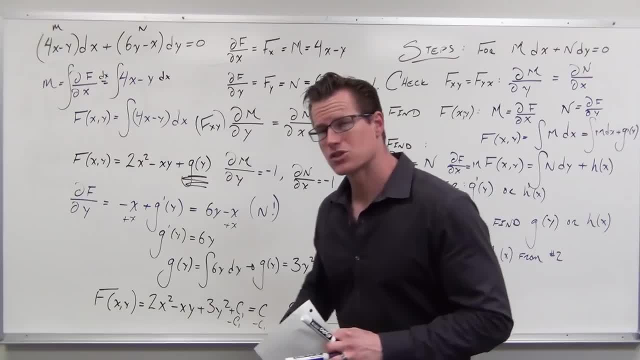 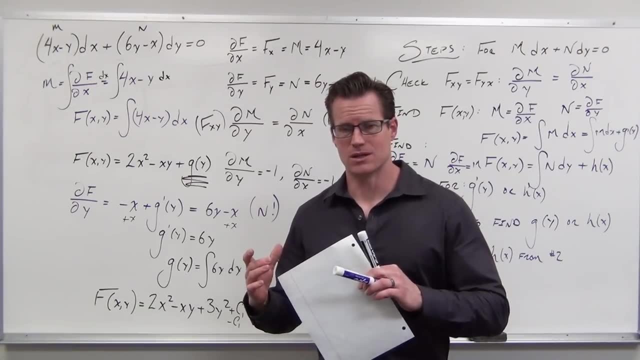 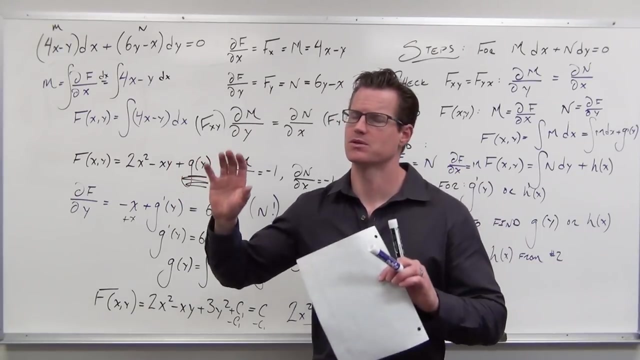 coming from a differential form from some function that looks like this: And if you have mixed partials that are equal, it says that that differential equation is an exact form of a differential equation for such a function. All we're really doing: take a piece and it becomes. 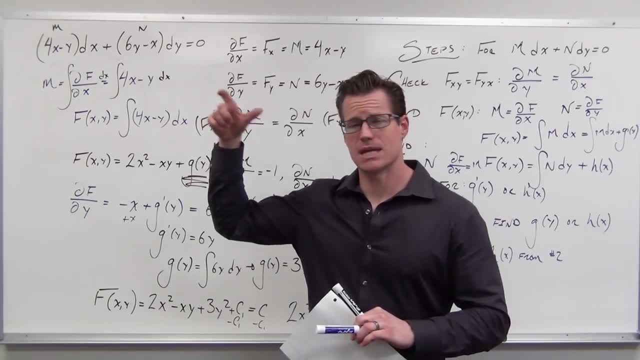 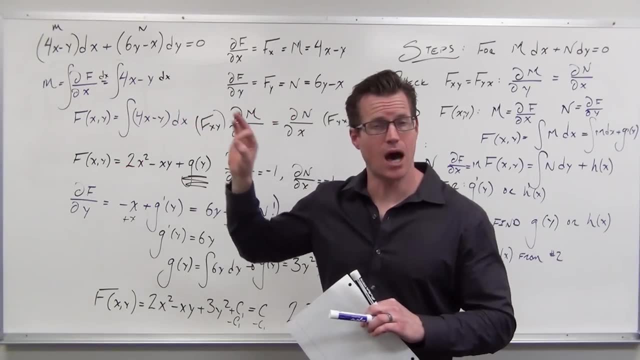 very easy when you get it okay And I hope that I've made it make sense to you. Take a piece, either m or n, do an integral, have a function You don't know. take a derivative, set it equal to the other piece. solve for that derivative of. 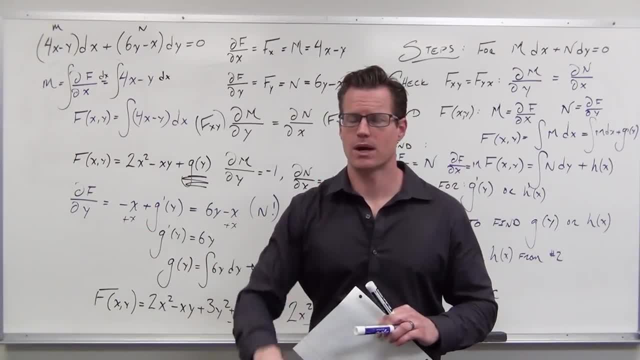 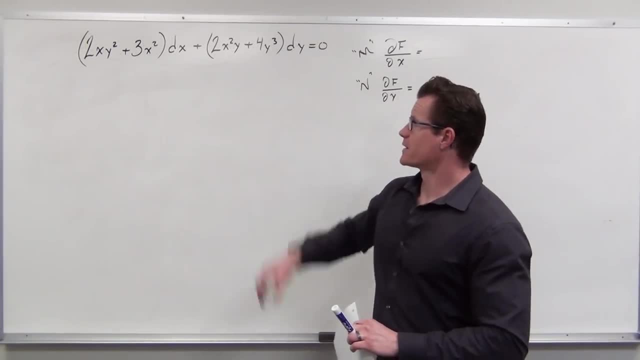 the function you don't know, integrate and then plug it in. We'll do one more right now, and then the next time we'll practice just the heck out of it. All right, here we go. We got time for about one more, So we're looking at this. We're going to determine, firstly, is this an exact differential? 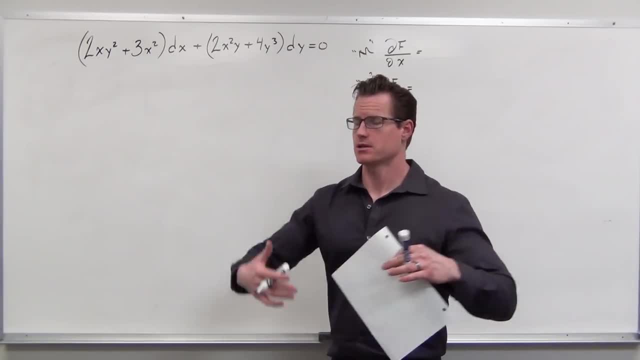 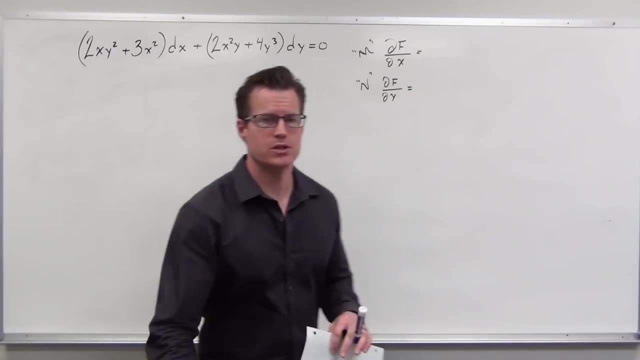 equation for some function that I'm going to try to find. If it is perfect, We have an easy way to do it. It's very streamlined, very nice once you get the hang of it. But we got to check it first because there's no sense in going through this if the mixed parcels are not equal. So I want. 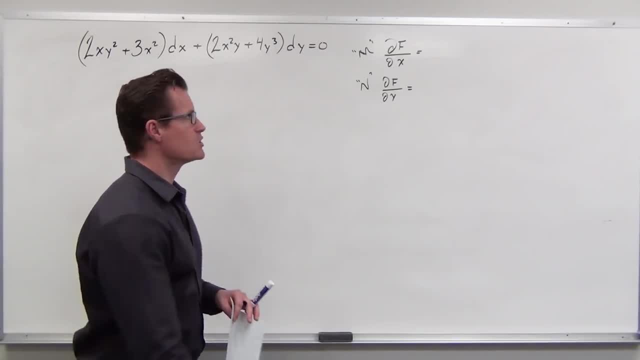 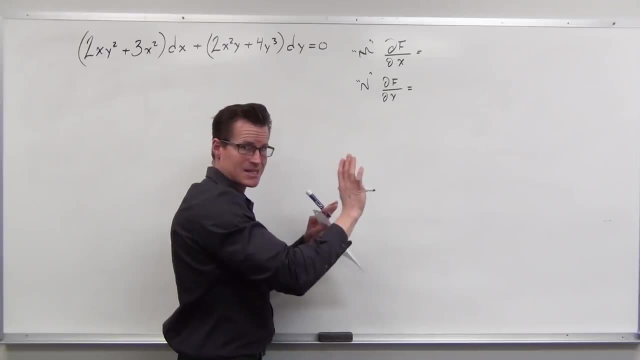 us to be able to identify this. I need you to be able to identify this. I need you to be able to identify that, from this form, the partial derivative of f with respect to x, if such a function, if this is a differential equation for such a function, if a function exists for which this 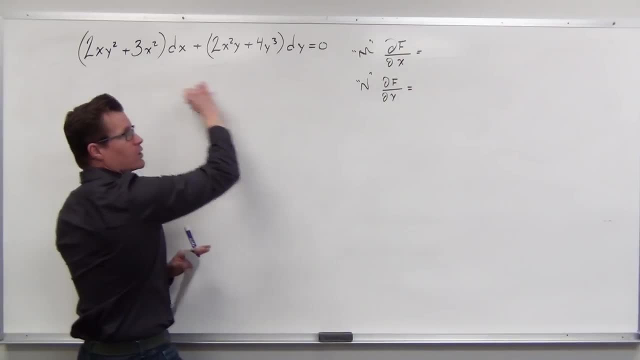 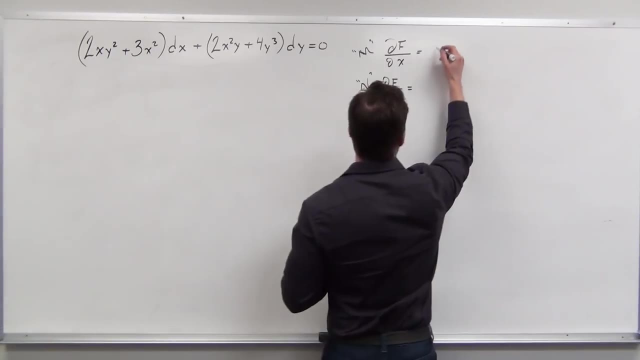 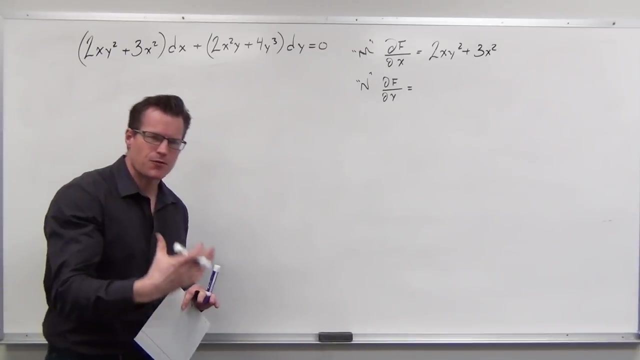 is the exact differential equation, then this part would be the partial derivative of f with respect to x. That's this. It's always next to the dx. And if such a function exists, such that when I take a derivative of it and put it in a, 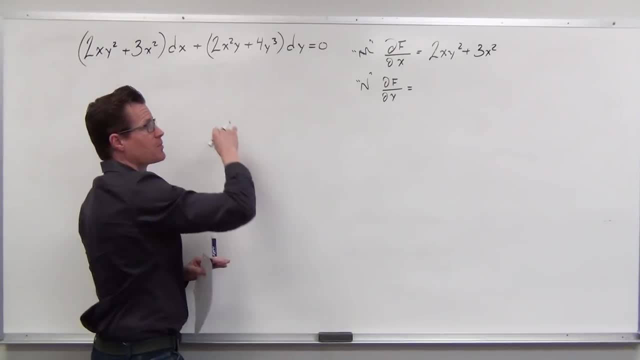 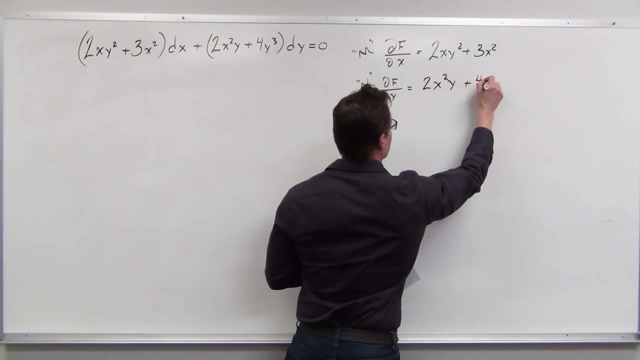 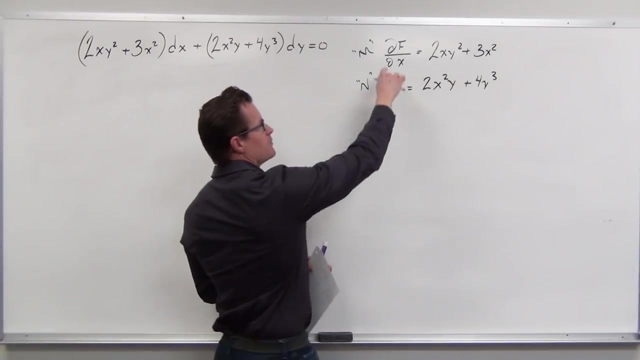 different form. it's this, then this would have to be the partial derivative of f with respect to y. It's always next to the dy. Now our test comes in and says: take the derivative of m with respect to y and f with respect to y, And if such a function exists, then this: 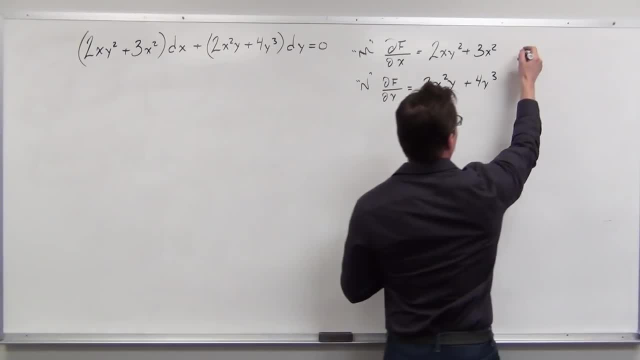 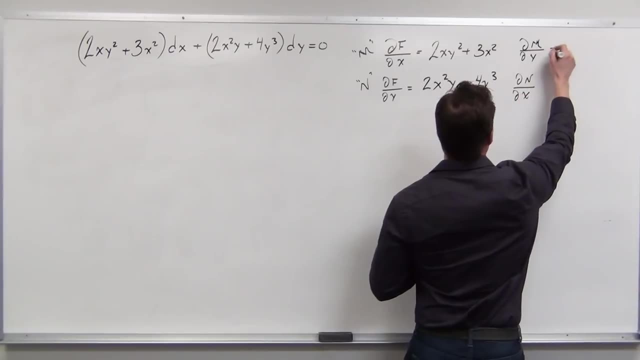 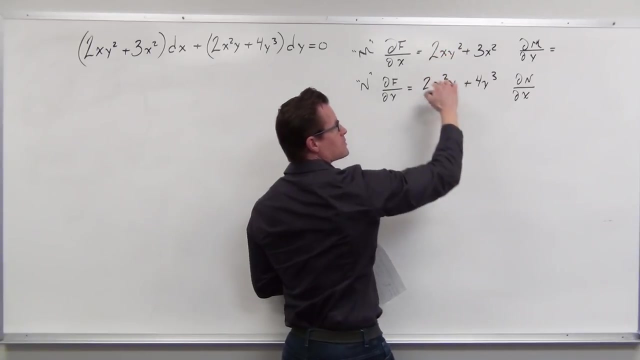 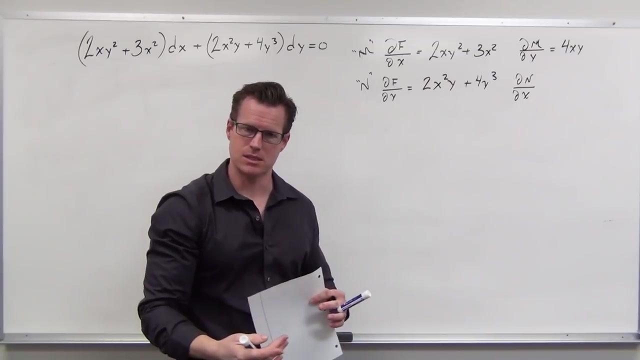 would be the partial derivative of n with respect to x And it will create some mixed partials. So this with respect to y says that's treated as a constant. So this would be 4xy And that would be 0. That would be a constant term if we're only looking at y's or variables. 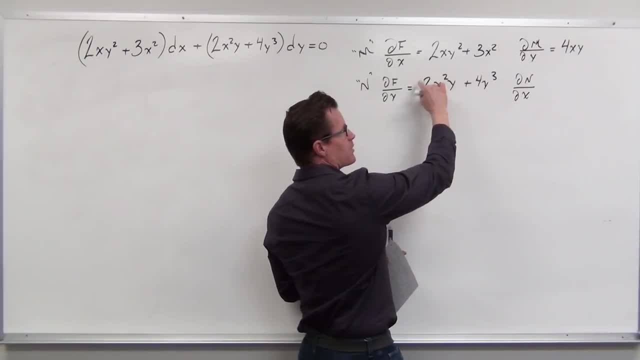 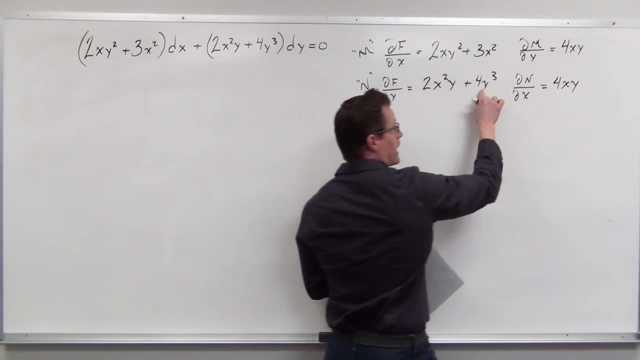 Likewise here with respect to x. we're going to take the derivative of y And if such a function exists, that would be a variable, That would be 4x, But that y would be a constant like a coefficient, But that y with respect to x becomes a constant. Hey look, those are. 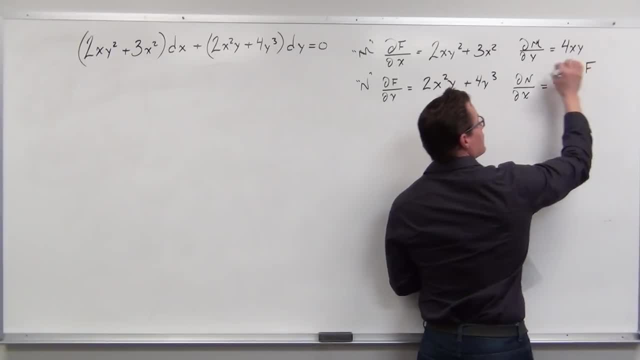 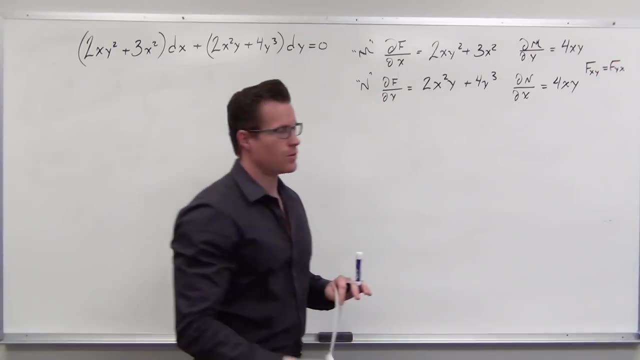 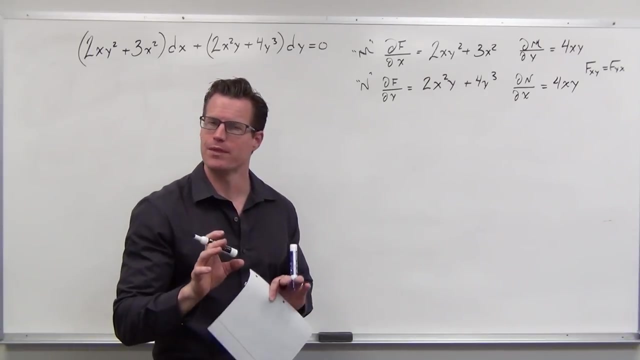 exactly the same. What this has proven is that f of xy first equals f of y, then x derivative of y with respect to y and then with respect to x. In other words, our mixed partials are greater than the number of differentơi commutators we are. 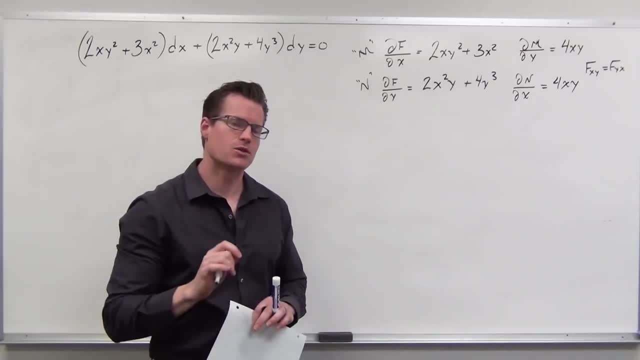 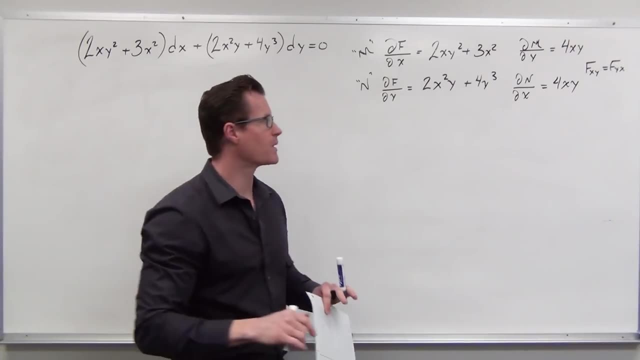 taking, And it's my discovered explanation this time that all the Detroit distributions proved that the division was speeds of greater than or greater than a function. Now what that says to us, it's very important- is that this is an exact differential equation, written in differential form, of some function that is. 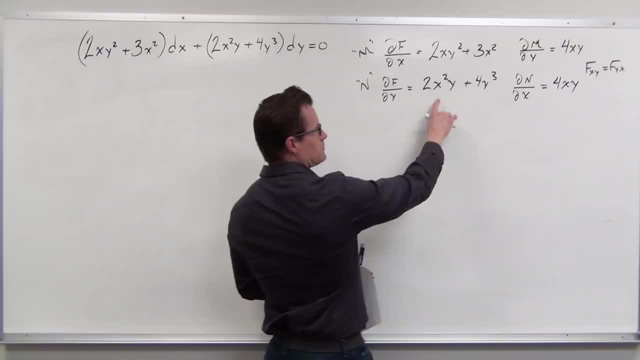 continuous and differentiable on some rectangle. Now it's up to us to find it. I mentioned earlier that it does not matter which of these you integrate, You just need to know which one you're integrating. So you either integrate this with respect to x, because that's parallel. 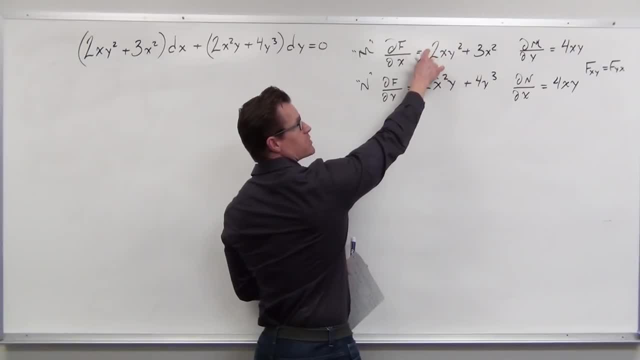 to x, because that's where it came from, Or you integrate this with respect to y. The point here is that commands between one zero and function k all are corruption. we'll be thinking of it in terms of operation only as we go more broadly, So you integrate this. 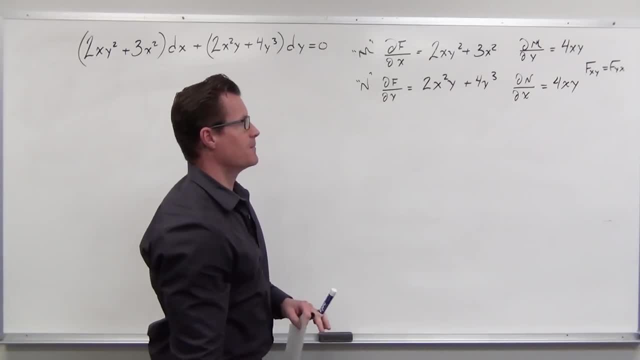 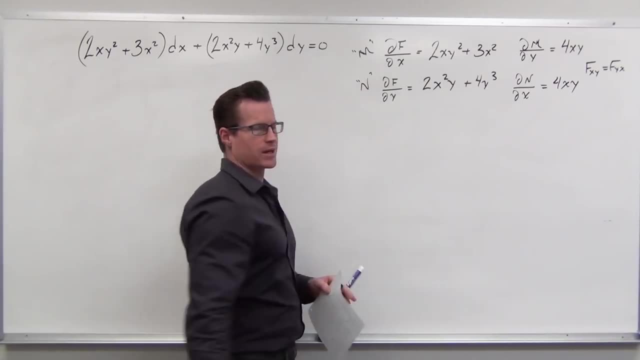 integrate this with respect to y, because that's where it came from. They look about the same Next time. the last example: on the next video, I'm going to show you how to do this one. It's: yeah, we can do that, So let's go ahead and let's. 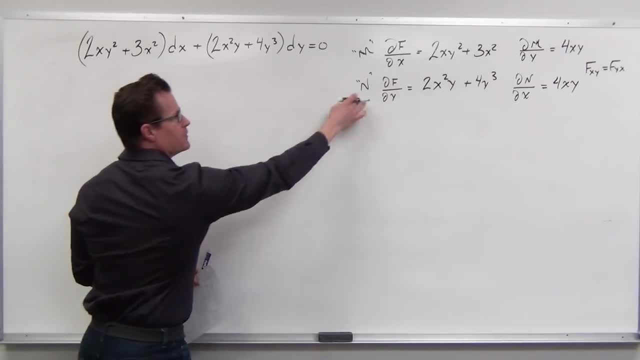 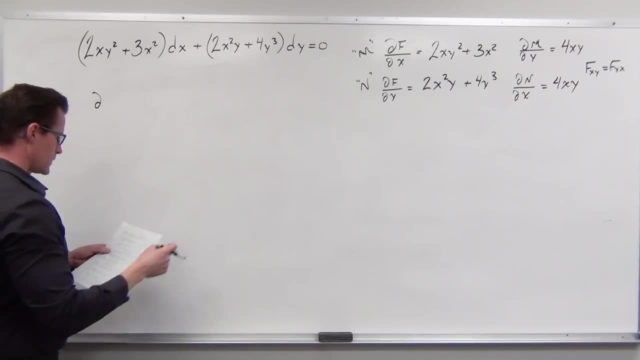 look at this. Let's say: let's pick this and say: I am going to take the integral of f with respect to Y. That's our n, That's 2x squared y plus 4y cubed. Now, what do we know about that If that's the partial derivative of f with respect? 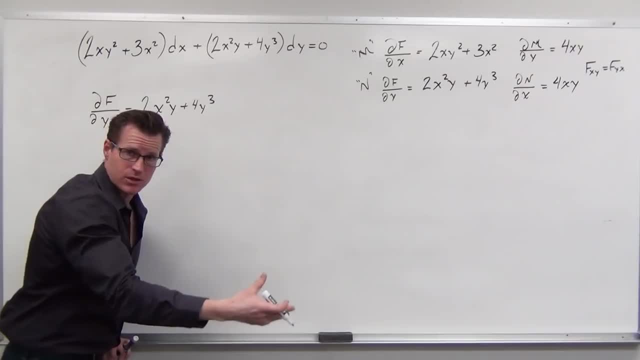 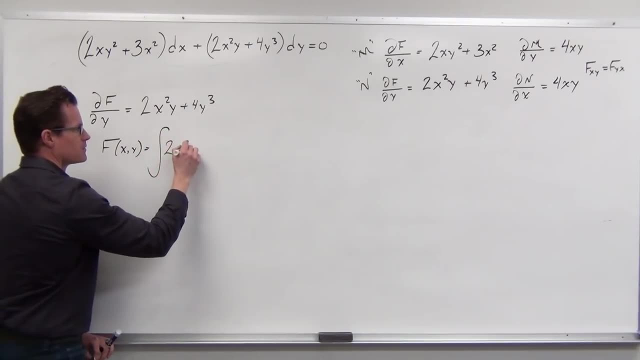 to y. how we undo all two derivatives is with integrals. So let's integrate this side. but we're going to do it with respect to y and then we're not going to be able to do it in 0. So in this case we do the. 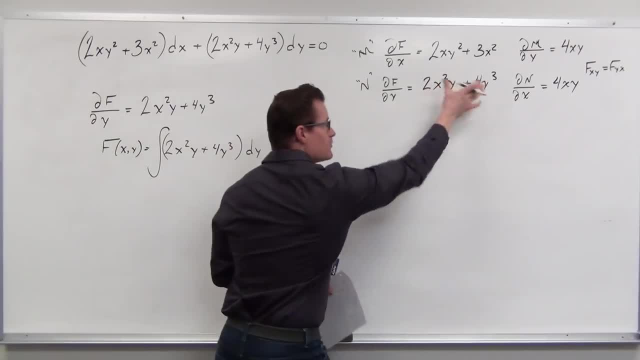 integral of f. we should being able to do it with respect to y. So let's make this- We're doing this with respect to y, because that's what n came from was a derivative with respect to y. We're just undoing that and say: let's undo the. 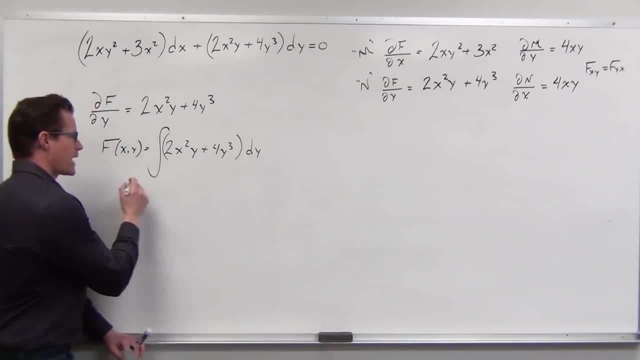 derivative with an integral with respect to y. But what's going to happen Here? when we integrate with respect to y, we'll have our 2x squared, y squared, but we would divide by 2.. This is all treated like a constant, So 2x squared, that's. 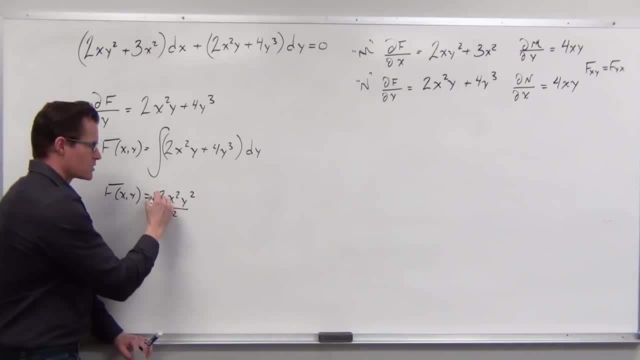 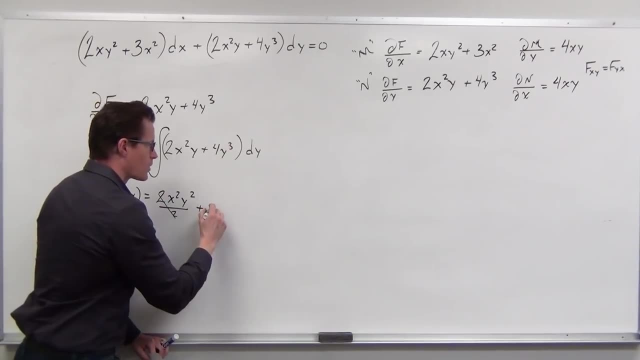 like the number five and then y squared over two. Our twos are going to disappear. Plus, this needs to be integrated with respect to y. So we'd add one. that'd be four divided by the new exponent. so that'd be four. y to the fourth over four and that's gone. 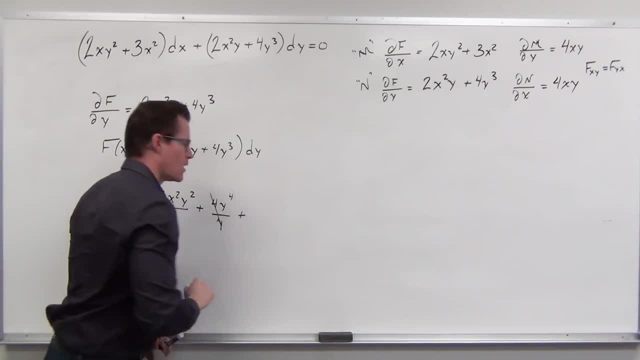 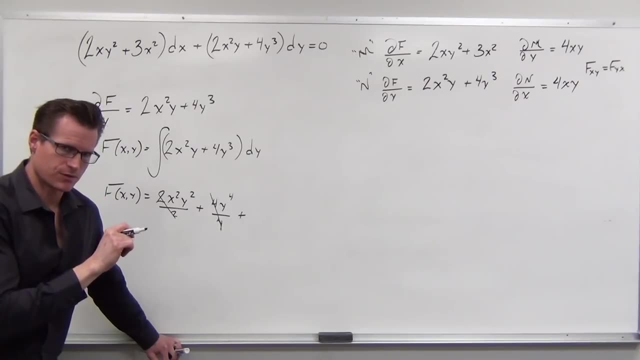 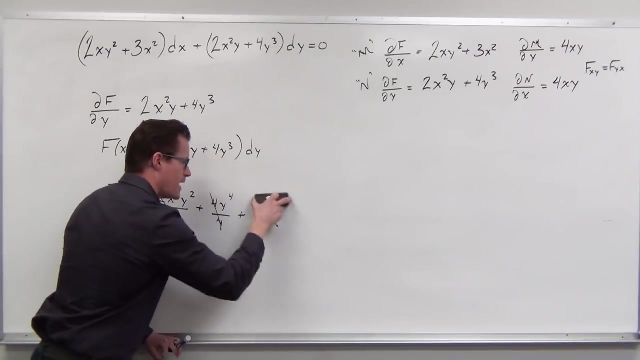 Now, every time you integrate, you know you get a constant right every time. But when we're dealing with stuff that came from a partial derivative- this was the partial derivative of f with respect to y to y- that means that every function of x would have been cancelled out, just 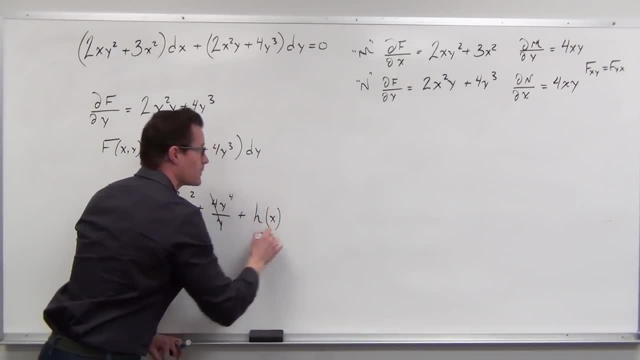 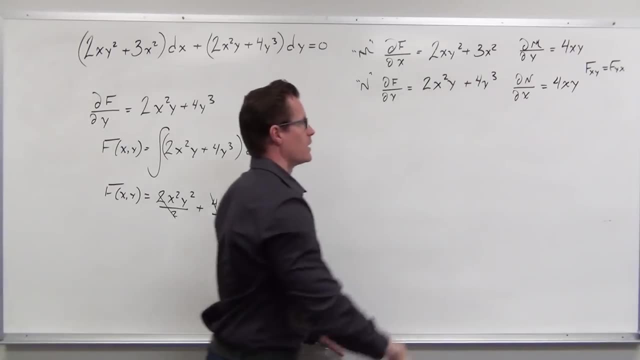 exactly like we did up there Right here when we took this with respect to y, this x cancelled out. When we took it with respect to x, that y cancelled out. So understanding that this came from a partial derivative with respect to y means that any. 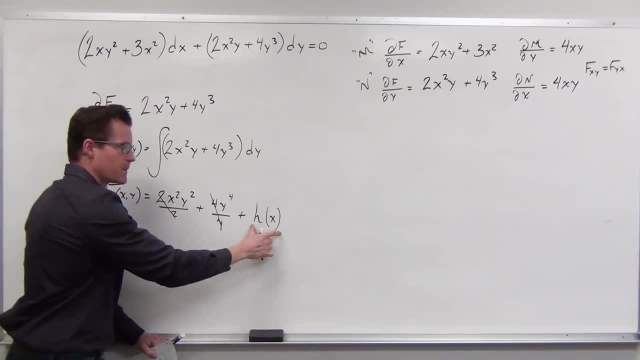 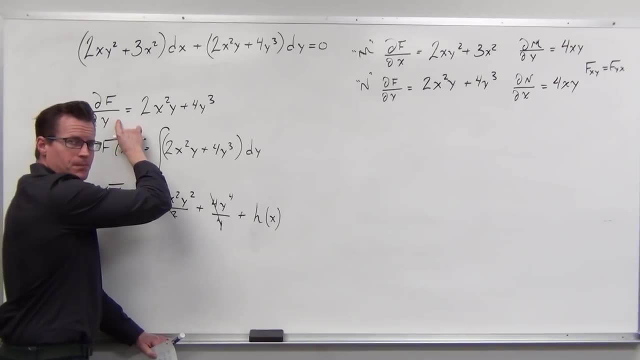 function of x that would have been there in the original function would have been cancelled to get this piece- I'll say that again, Because that's a partial derivative with respect to y- any terms or functions of x alone would have been cancelled out when we took a derivative of this with respect to y. Therefore, when we get a, 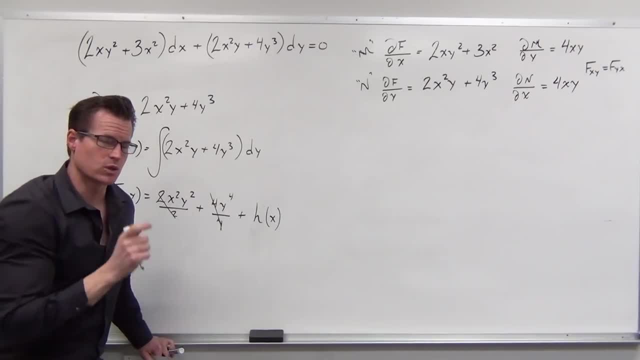 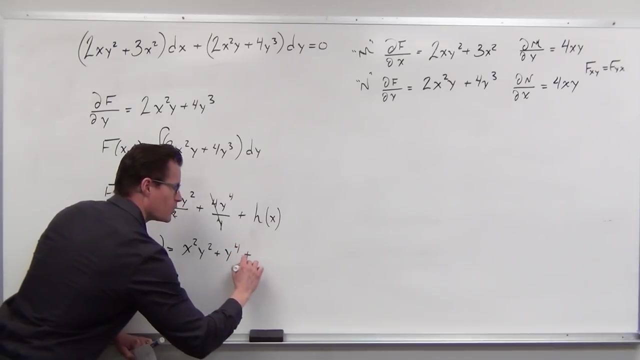 constant. it can possibly have x's in it, because those would be held constant, with a partial derivative with respect to y. This is what our function looks like. Our function really is this. Our function is x, x squared, y squared plus y to the fourth, plus some function of x that we don't. 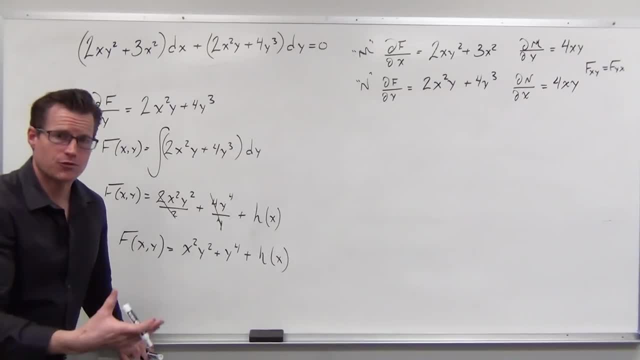 know Now how do we find that? Well, beautifully, since we used n to find an integral, to find our function, now we can take a partial derivative of f with respect to whatever variable you didn't just integrate, So we integrated with. 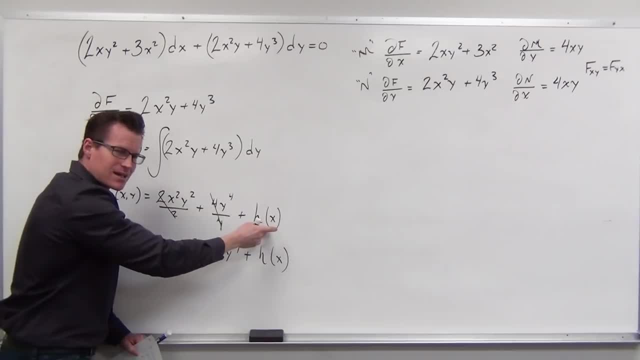 respect to y. right You go. okay, I have a function of x that I don't know. If we want to find a function of x that I don't know, let's take a partial derivative with respect to x and set it equal to the thing. 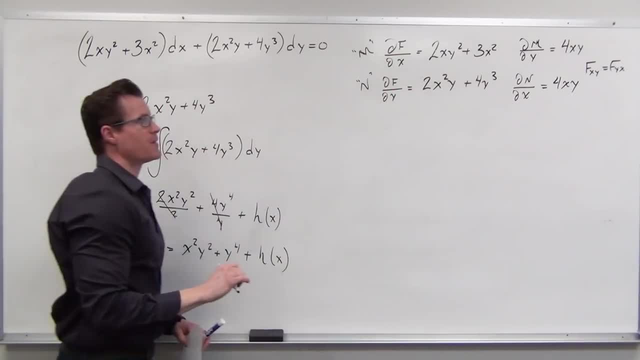 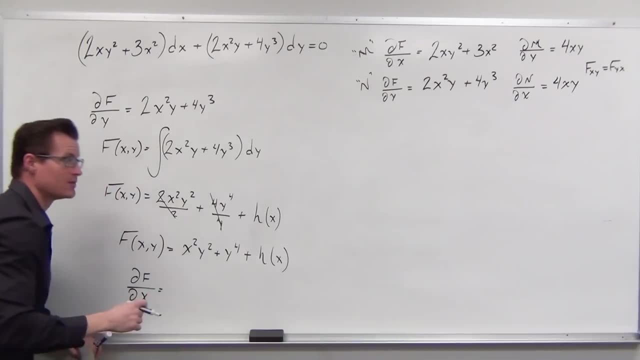 that it has to be. M is the partial derivative of f with respect to x. So if I take the partial derivative of f with respect to x, you have to believe that I'm going to be studying this. equal to M. This is M. This is exactly what that. 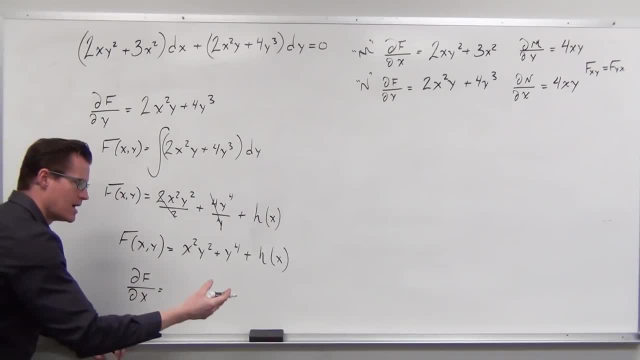 means. So let's take this partial with respect to x. now The variable that I did not just integrate in order to find the function that I don't know. Well, let's see here. That would be 2x, that would be constant. 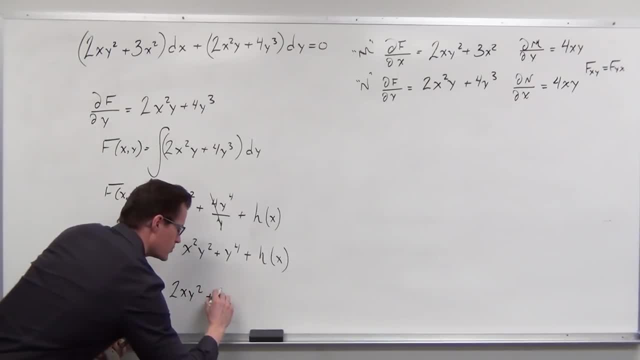 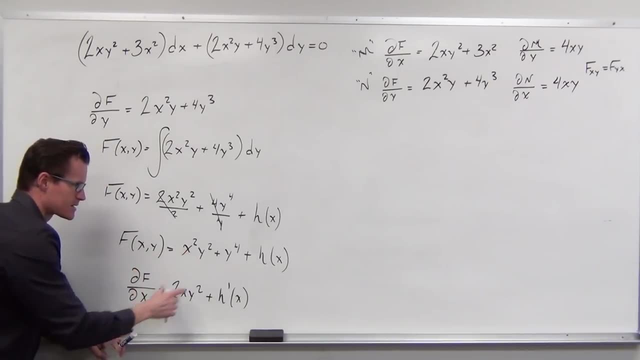 This would be a constant, that's 0.. Plus, if I take a derivative, I'd have a derivative with respect to x. Check it out. this is so cool. Take a derivative with respect to x. this is the derivative with respect to x. 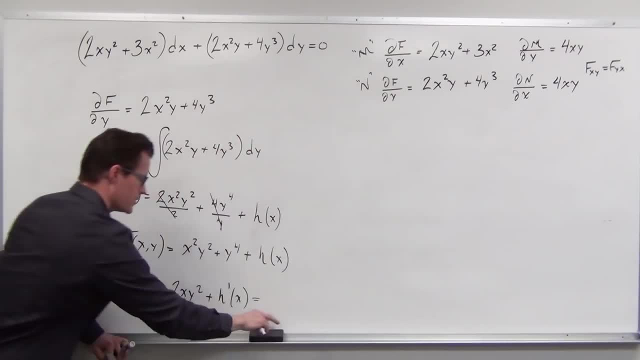 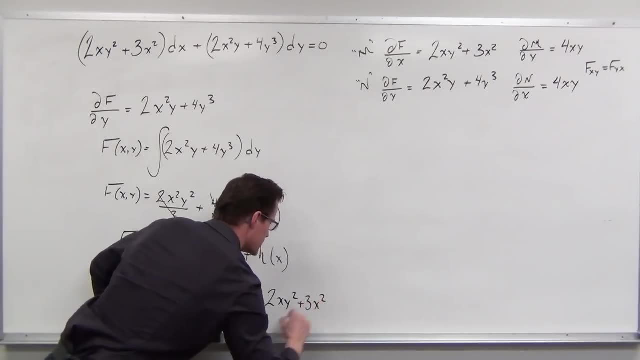 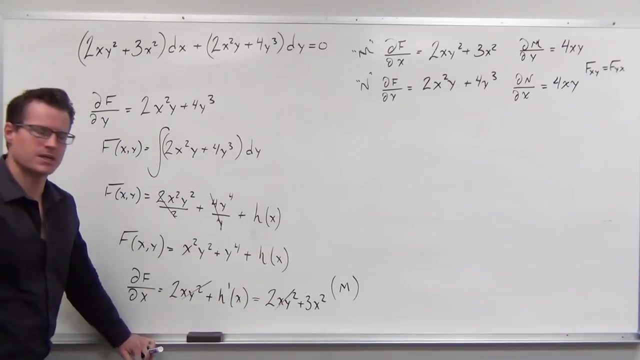 and this is m, the derivative with respect to x. Notice, as predicted, a lot of things are going to cancel, Because you're going to everything with y is, in other words, in this case, and everything with x is going to be done the other way. 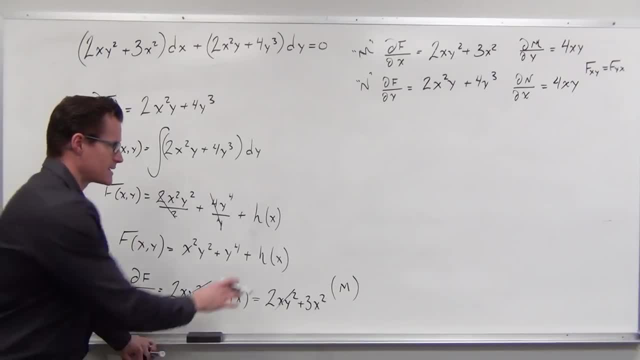 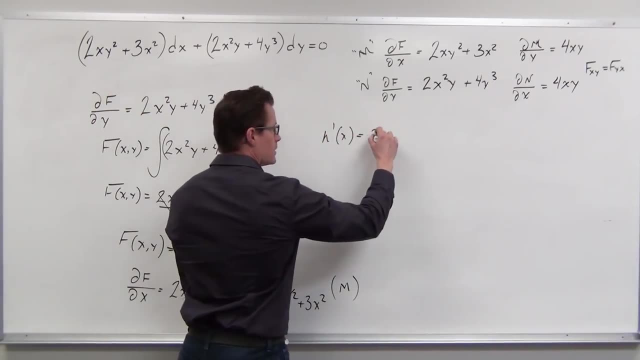 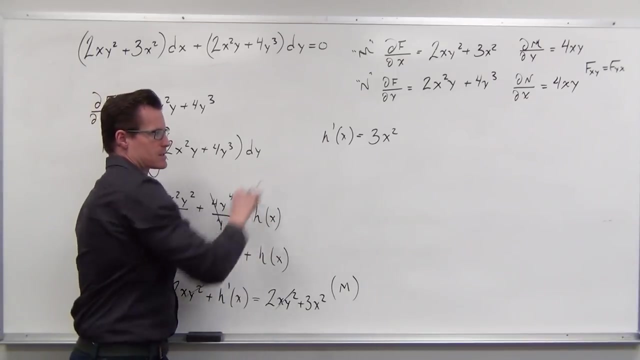 you're just going to have a function in terms of x or y. That's exactly what this says. So a first derivative of the function that we didn't know is 3x squared. I'll say that again: The first derivative of the function that we didn't know is this: 3x squared. 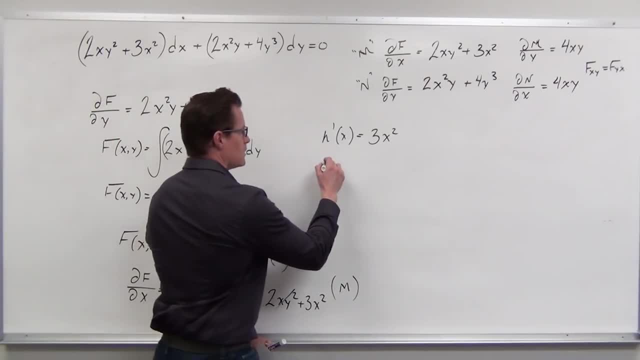 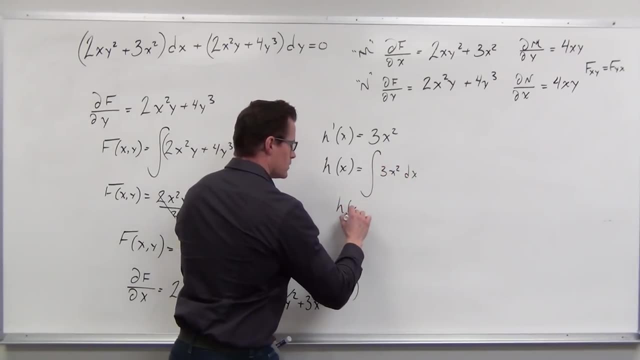 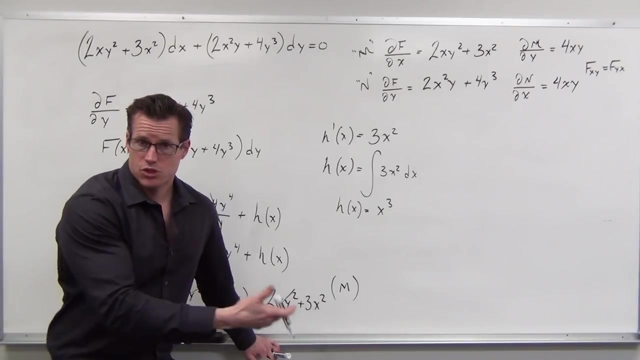 How do you undo derivatives? Let's integrate. Then h of x would equal the integral of 3x squared dx. Or let's just execute. Do I have to do a constant? You should when you're doing integrals, but here we don't have to. 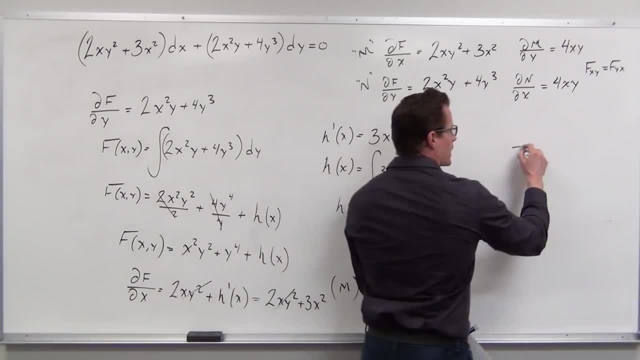 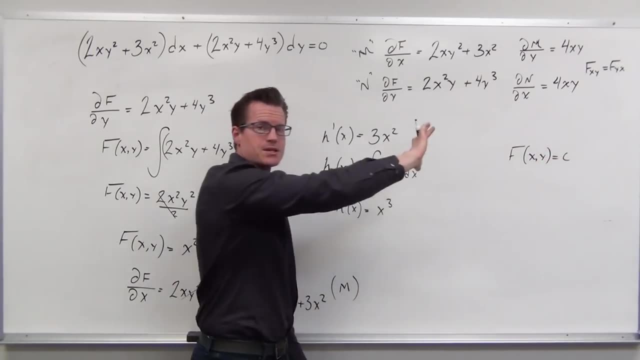 because we know where we're going with this. We know we're going to have to do a constant, We know we're going to have some function equal to a constant anyway, And that constant would just get wrapped up in the second one. Now, if you want to show it every time and subtract it, totally cool. 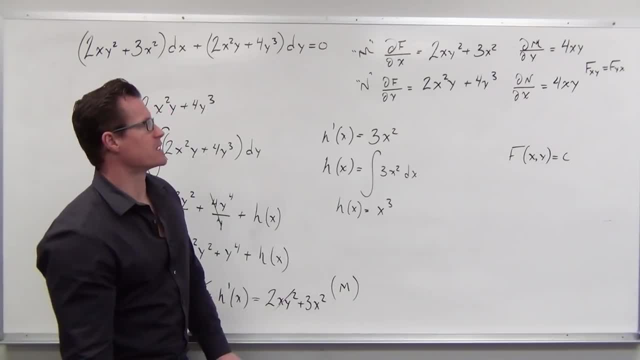 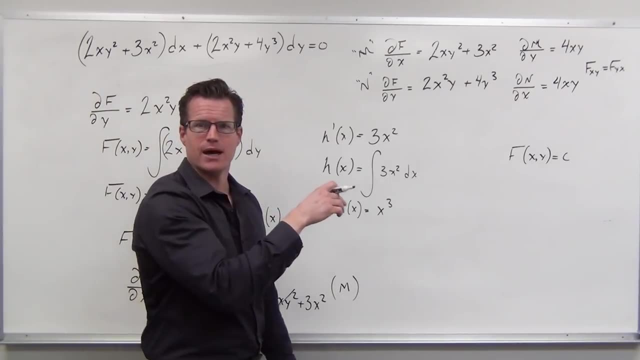 but we don't have to. What we do have to understand is the following: We've got to understand that if our mixed partials are equal, this is an exact difference in the equation. If right, Once we have that, once we understand, that's an exact difference in the equation. 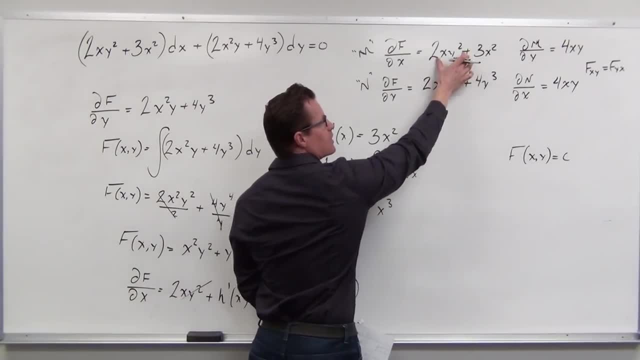 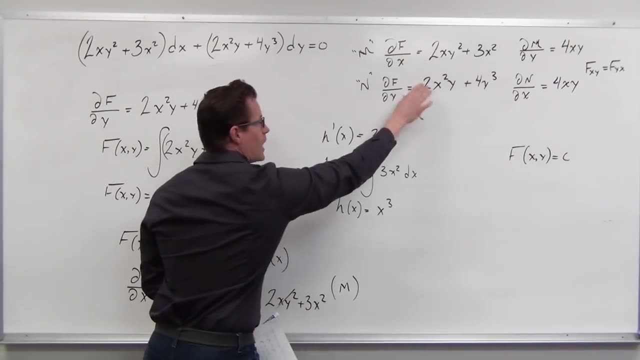 take one of these partial derivatives of f with respect to whatever variable you want, whatever looks easier, And integrate. Integrate n with respect to x, n with respect to y. I did the second one to give you some diversity here. So with respect to y, 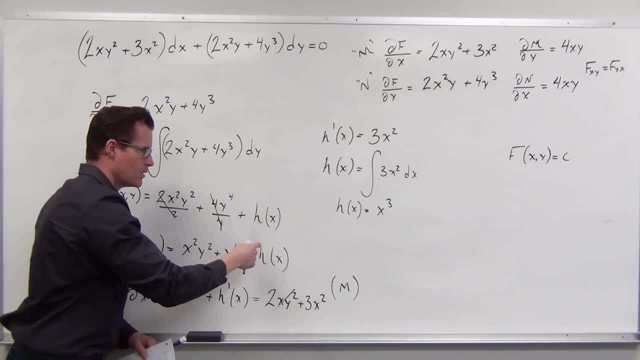 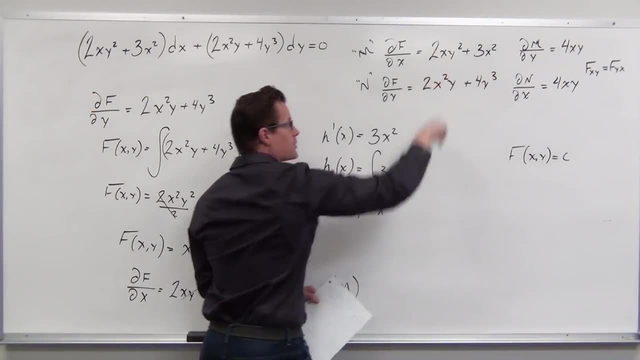 Great, Okay, do it. You can have a function of x that you don't know. Okay, Well, now take a derivative again, but with respect to the other variable, So you can set it equal to the other thing. 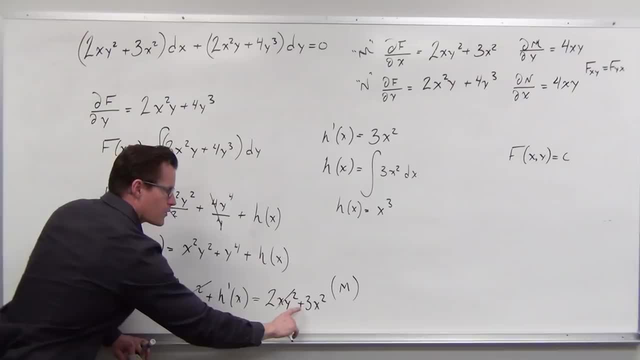 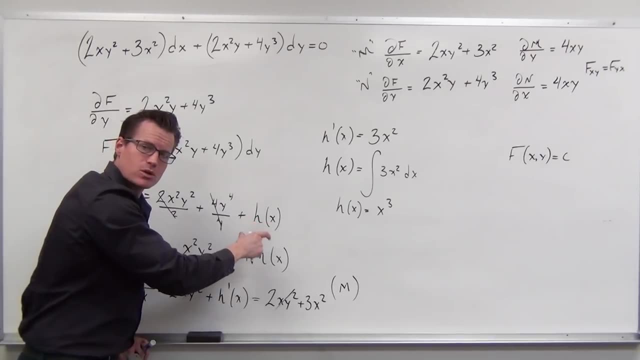 That's going to allow you to make a derivative solve for the first derivative of the function of x that you said would have been held constant under differentiation with respect to y. in this case, We do our integral, we have our function and we are done. 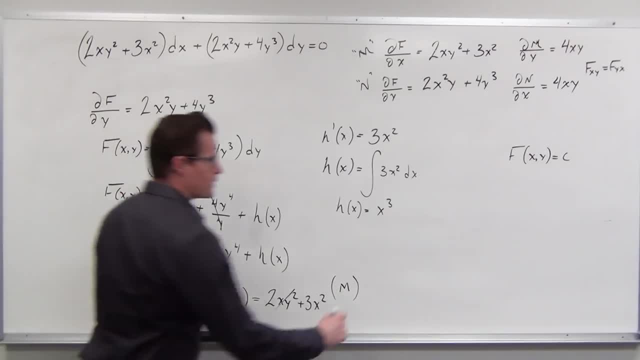 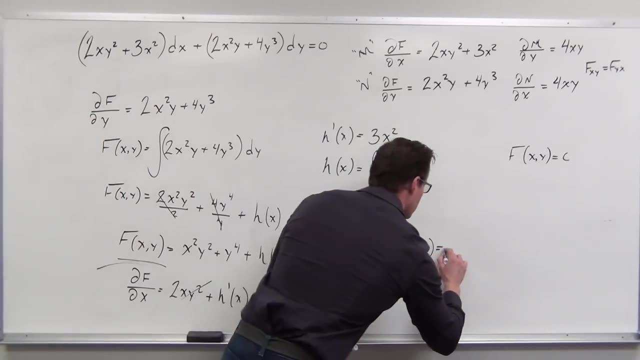 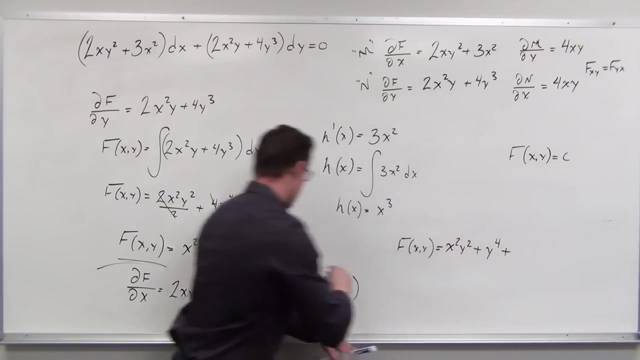 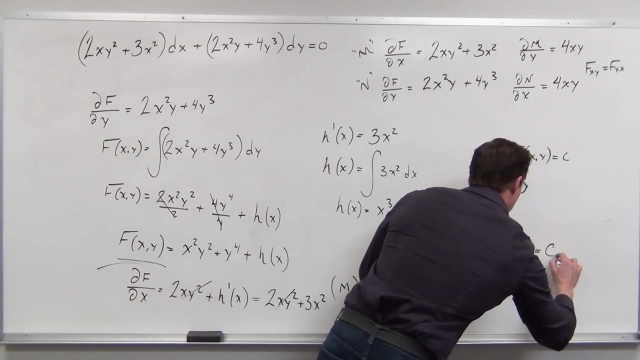 So our function of x, right here, our function of x and y, was x squared, y squared plus y to the fourth, plus some function of x that I didn't know and have just found, And that's going to equal some sort of a constant. 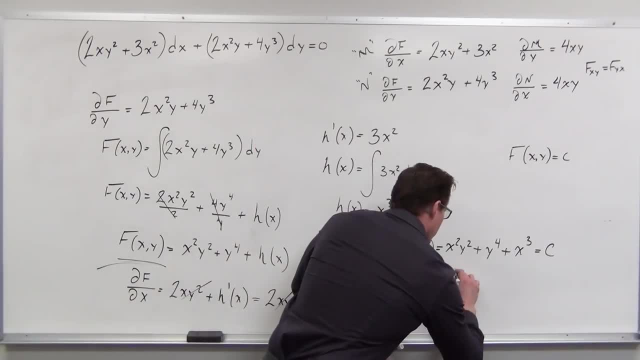 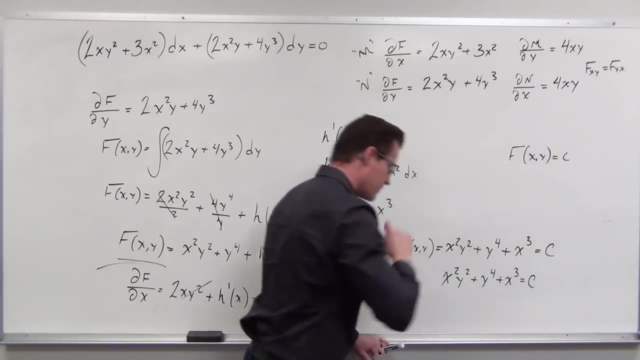 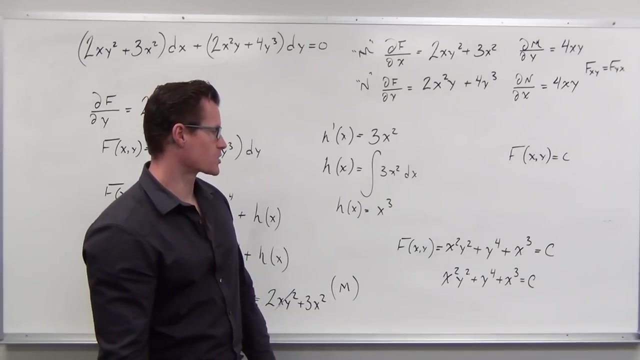 Because that's where these functions come from. Now we can write it simply like this, And if you had an initial value problem, this is where you'd go ahead and plug it in. What's really cool is if you take a partial derivative. 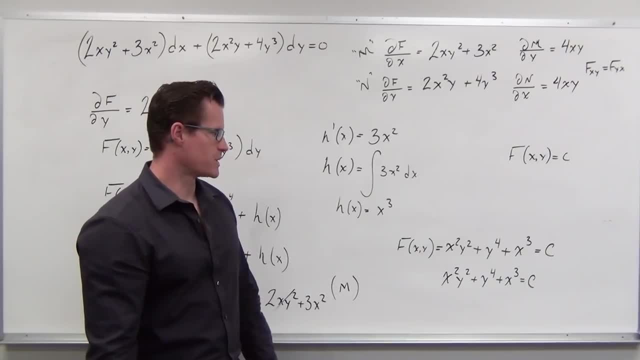 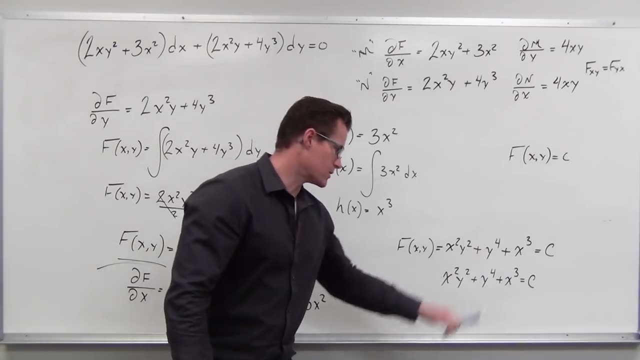 I'm sorry. if you take a derivative of this with respect to x on both sides and you start figuring it out and put it in differential form, it's going to be exactly that thing. On the right-hand side, you get zero. 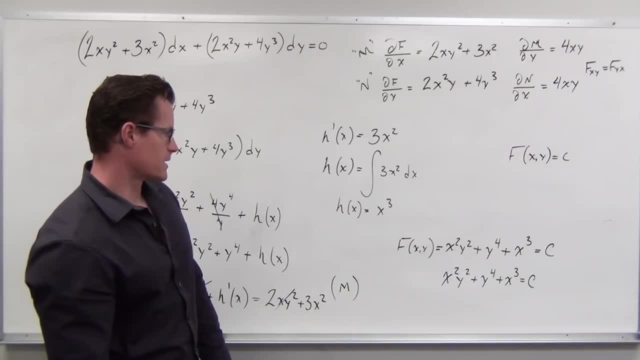 On the left-hand side, you get partial derivative with respect to x, That's that 2xy squared plus 3x squared. That's right there. And then partial derivative with respect to of f, with respect to y would give you that 2x squared y of 4y. 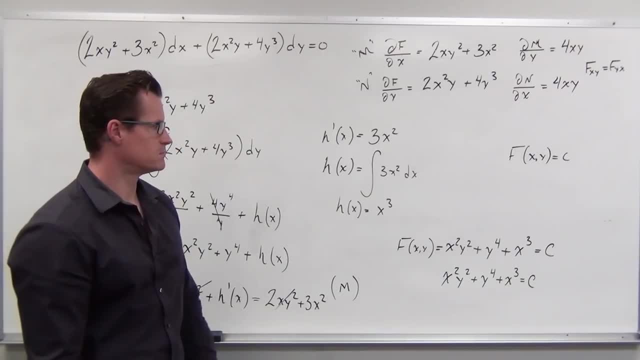 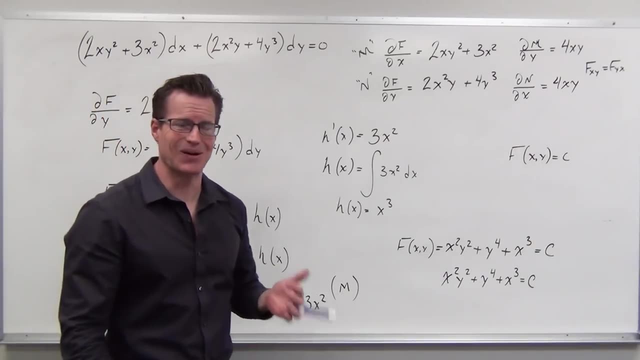 The third and then that second part would be dissolved. so I would go to zero And you'd have that dy dx which gets spread here and here, And that's it. That's so cool. So anyway, I hope that that's made sense. 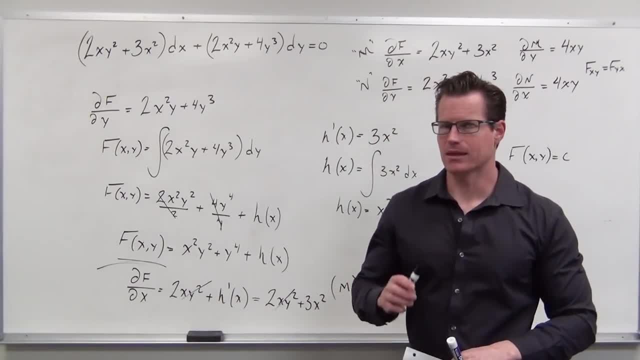 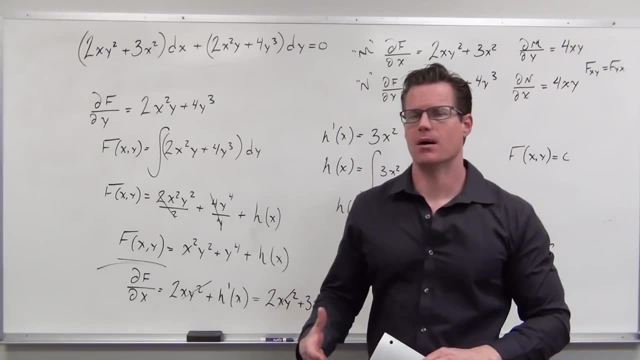 I hope that I've illustrated this well enough that you understand what exactly a differential equation, that exact differential equation is, where it comes from and what you're doing when you're undoing it. I hope I've explained to you the necessity of doing the test first. 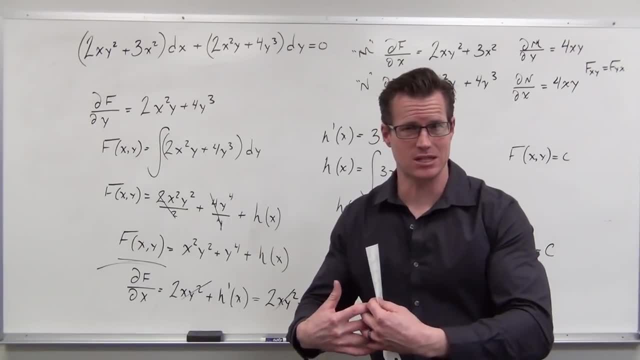 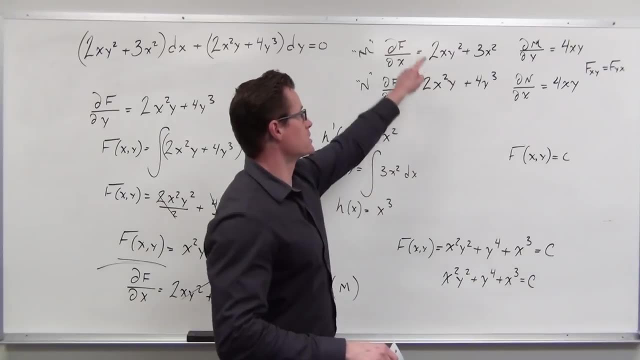 because that's saying that mixed partials are equal. therefore your function. It is continuous and divergible on some sort of a rectangle. I hope that I've made it very clear that most textbooks will always do this integral and then take a derivative and set it equal to this thing. 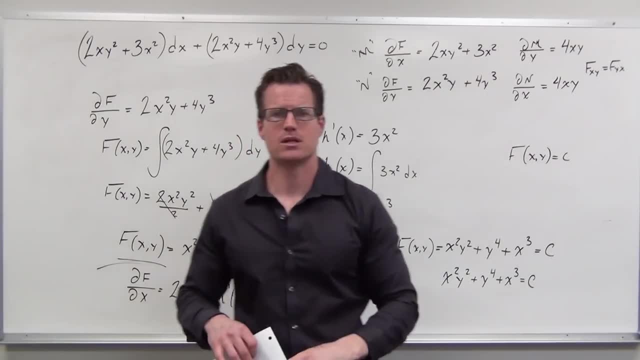 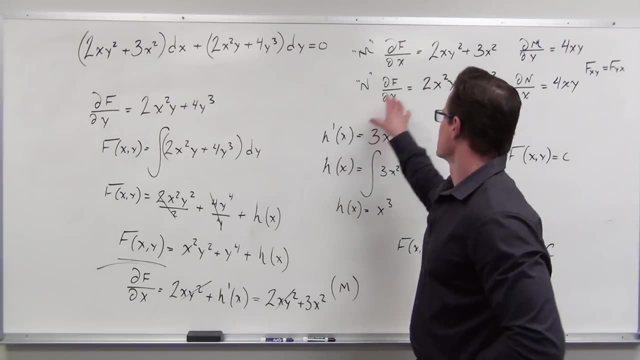 And that is okay to do. Most of the time that's fine. I made the point in the second example, kind of went off script here a little bit to show you that that's not necessary. You can certainly take the integral of this with respect to y take a derivative. 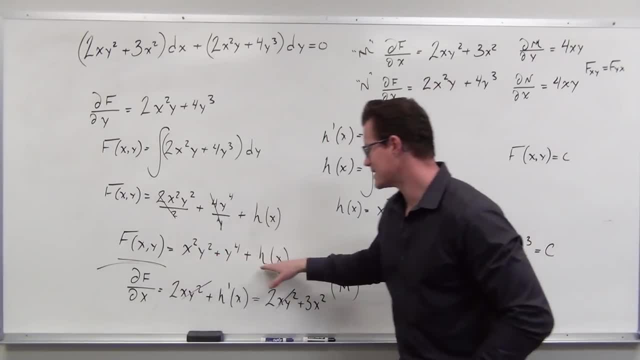 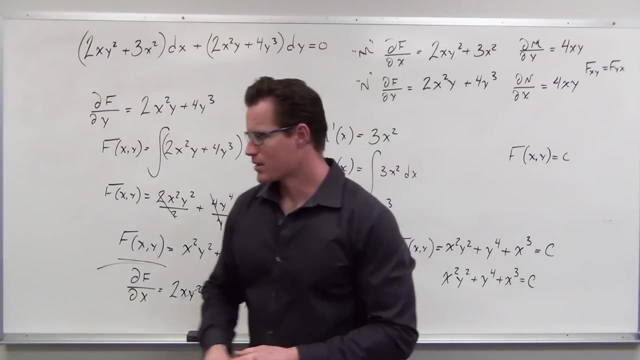 keep it in the function of x. take a derivative with respect to x and then set it equal to m. That's the opposite way. It will give you exactly the same answer. It does not matter which way you do that. So, other than that, I think that's about it. 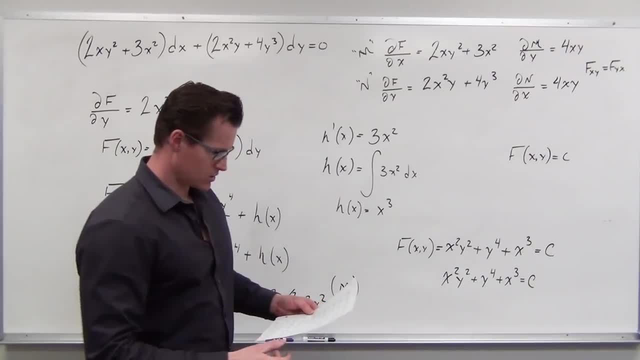 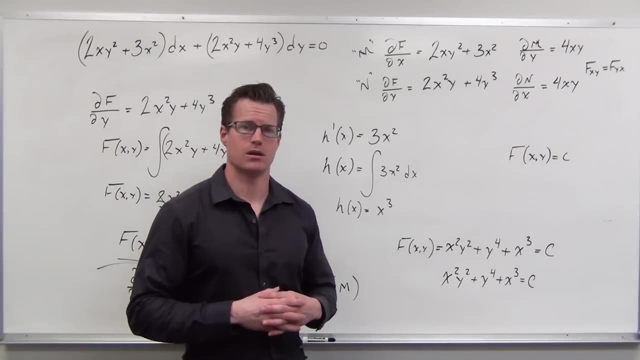 Next time, what we're going to do is we're going to practice, man, just a whole lot of these to make sure that we're really good at it. Then I'll talk about an integrated factor that we can use on these things. that might not be exactly exact.